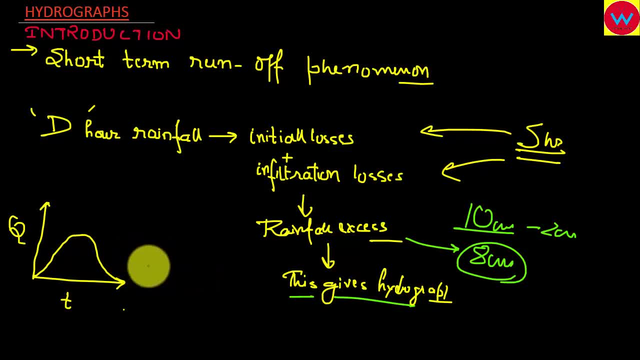 versus time in a channel or in a stream. So we have- we have seen earlier that how do we calculate run off and what is run off? basically you need to go to that lecture to understand the concept of run off. So rainfall axis is that thing which causes run off. basically, it's as simple as that. 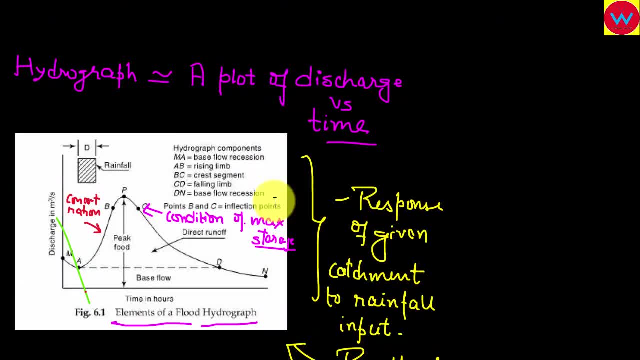 Now we look at a graph of hydrograph for how hydrograph is plotted and what are its various characteristics. So first of all, we see that, as I have told you, hydrograph is a plot of discharge versus time. that is, here you have discharge and here we have time. 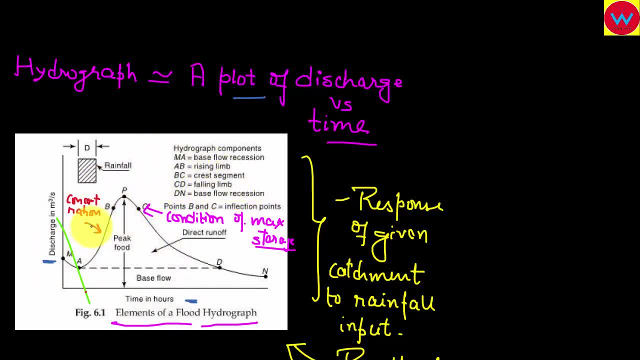 now, what are various elements of it? this is called as concentration concentration limb. that is from a to b, but before that m. a is your base flow. base flow means that, suppose this is your river, this is, this is your riverbed, and we say that we have contribution. 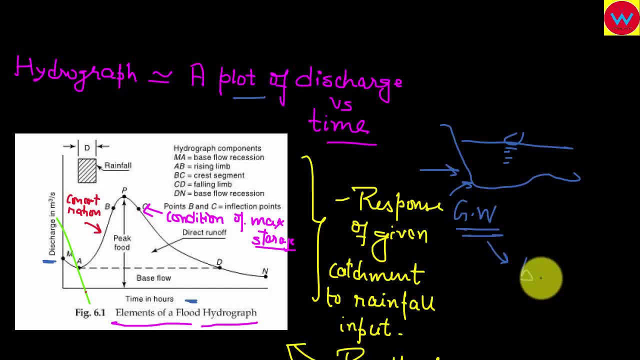 from groundwater. so this groundwater is called as base flow. that is, even without rainfall there is some contribution or some flow from the groundwater. such flows are called as base flow. so m- a is your that base flow and a- b is your. rising ring, rising limb, means suppose this is our catchment area and here we are. 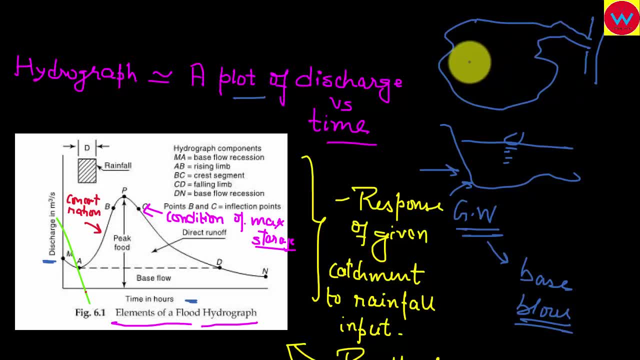 looking at our outlet. so if the rainfalls takes place, water will move from these channels to this outlet basin. so when rainfall is taking place, when rainfall is taking place, we know that water from all these areas will eventually come down. so what will happen? that here we are. 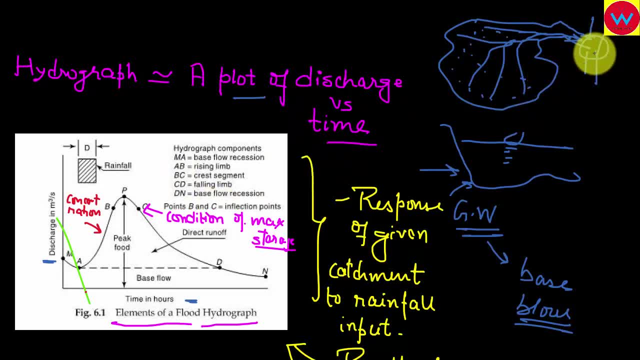 measuring this graph. we are plotting this graph based on the discharge and time obtained at this place. so, from a to b, we have rising limb, that is, our water is being concentrated, or that most of the water is starting to come down to the outlet basin or outlook, or the catchment point. that is why we 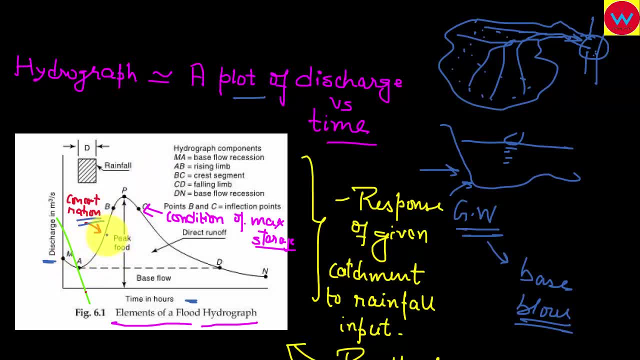 have this high peak value, that is very quickly, in very short span of time, we have most of the water reaching our outlet basin. then from a to b, we have a rising limb. then from b to c we have crest segment. that is, this is the time when we have peak value of our discharge in our catchment basin or 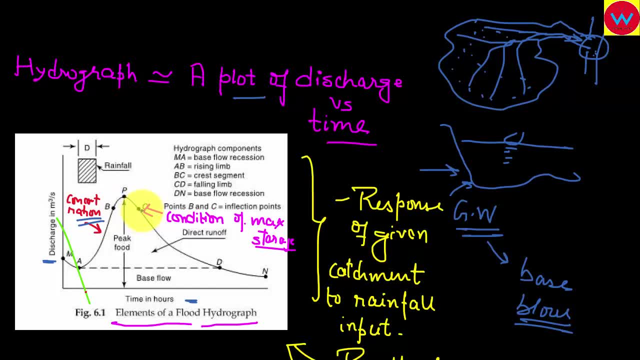 then from c to d, we have falling limb, that is, the water has stopped coming into. water has stopped falling or rainfall has stopped, but most of the water peak flow has occurred and the water is now starting to recede. that is means the discharge value of water in the stream is very less, or 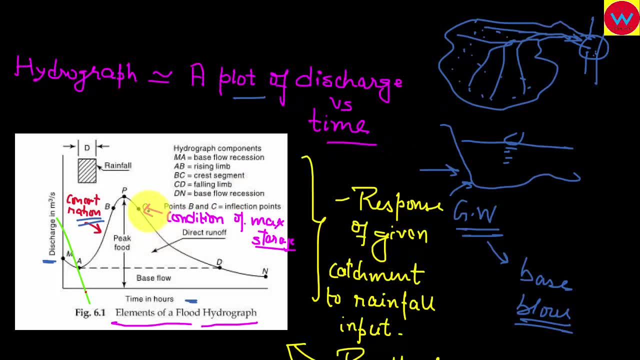 it's likely to be going down. that is what we have this value of. that is what we get from this curve of cd. this is what we get from this curve of cd. this is what we get from this curve of cd. this is called as falling limb. this you notice. you will notice that the peak of, or the slope of, this cd is. 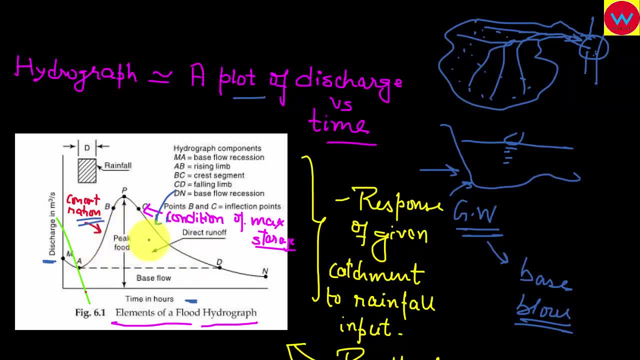 lower than the peak of a and b, or that is the slope of a and b. this is because the water gets accentuated or accumulated very quickly, but it disposes or it goes off relatively slowly as compared to its get concentrated. therefore we have cd limb as. 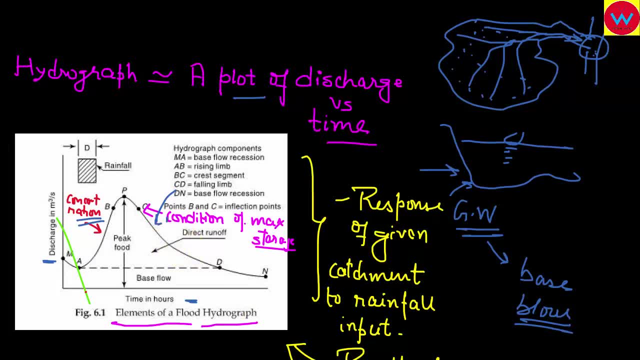 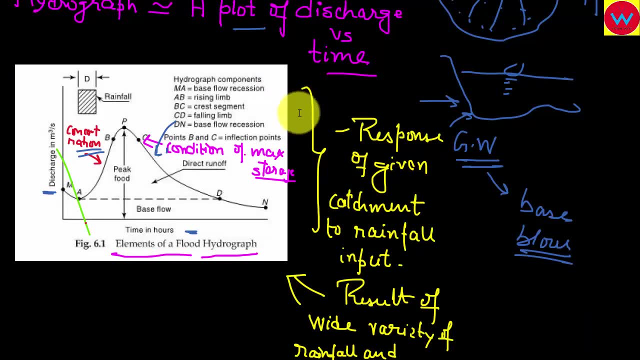 our falling limb, which is has a relatively mild slope than ab limb. one of few defining characteristics of hydrograph is that it represents the response of catchment of rainfall input. that is what is the response of catchment area. that is how this catchment area is likely to behave when this rainfall will take place on it. this is 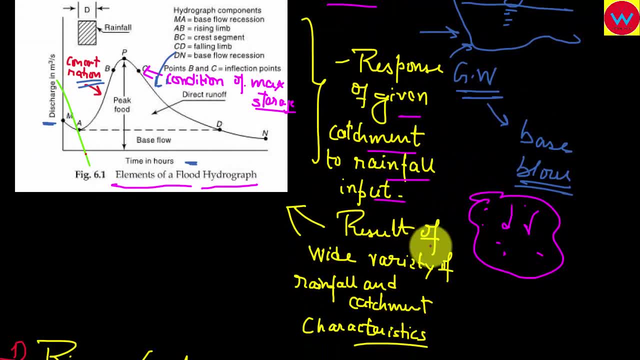 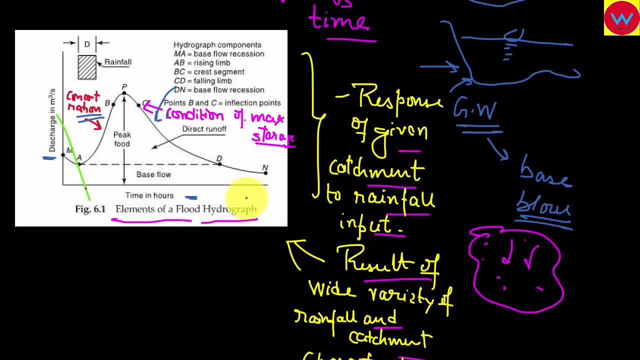 what the general event is. so so at one point there is is every case a rest spot of due. so we mean almost every case is a whole, lots of different case, and so you can see, and these aspects may be associated to var number of factors, or factors associated with: 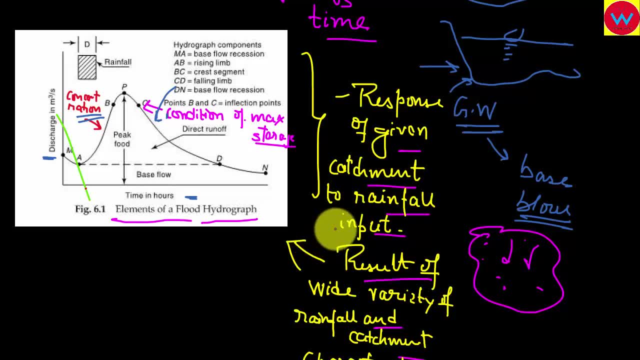 change under the changing trend of thefalls vary depending upon the current behavior of cadavers. whatever different aspects be, and however different features be, hey, they still after they are declined, given by this hydrograph, and it is also the result of wide variety of rainfall and catchment characteristics. 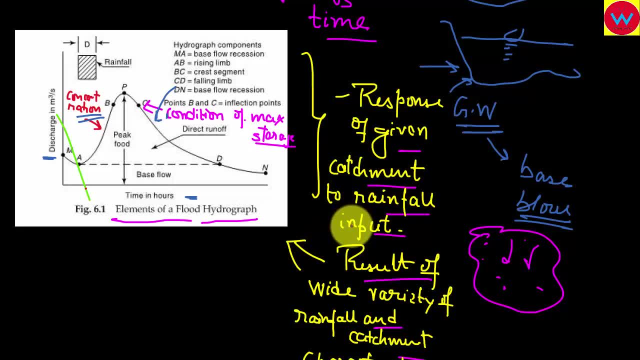 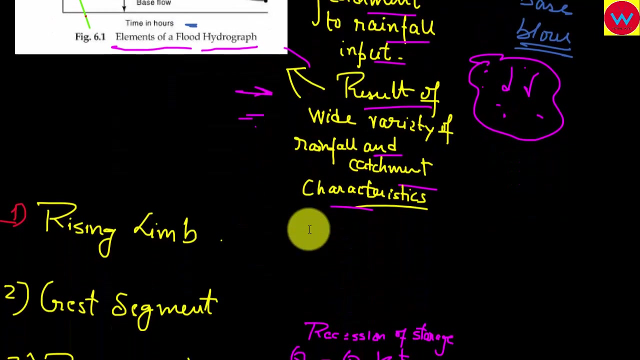 rainfall is taking place and what is the shape, our catchment area, how drainage basins are spaced. so all these factors affects our the shape of hydrograph. so we will be looking at how to calculate hydrograph and how we can simplify the model based on few input that we get from this data of rainfall. so, as we have, 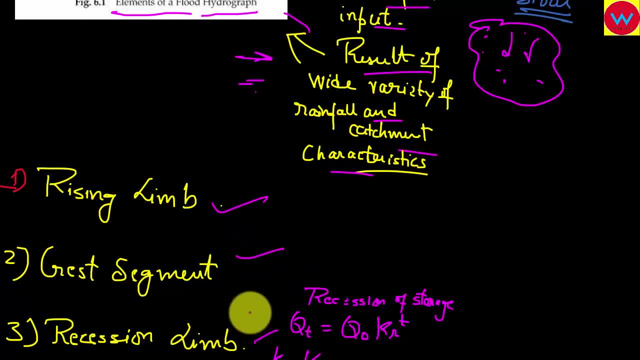 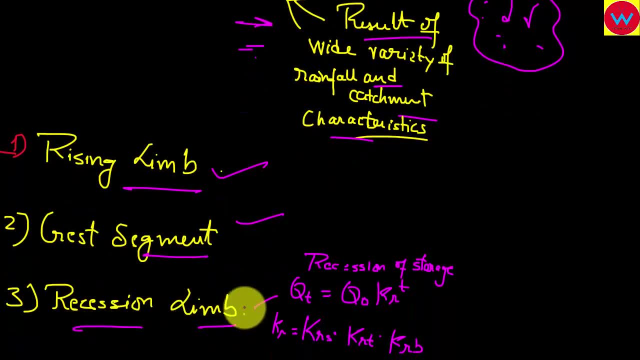 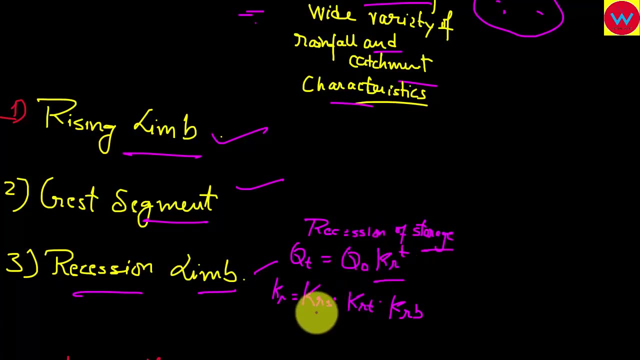 seen that there are three basic part of hydrograph: rising limb. that limb which rises, and we have crest segmented, is maximum discharge value segment and then we have recession limb. recession limb is basically our characteristic of, basically characteristics of storage basin. it is, it is, it is independent of. 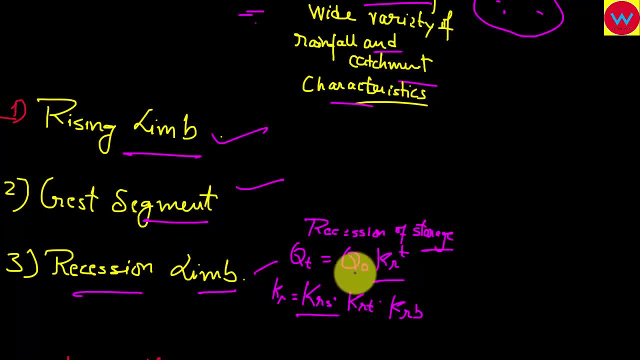 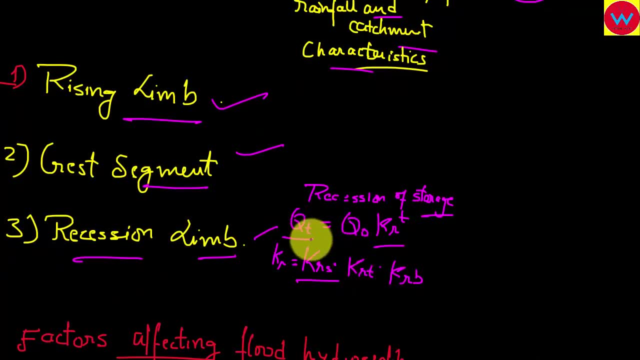 base our rainfall characteristics. it is dependent dependent on catchment characteristics. it is dependent on the rainfall characteristics. it is dependent on the characteristics. this QT is is discharge of recession limb at any time. T and Q naught is the discharge at time is zero and K? R is recession factor now. 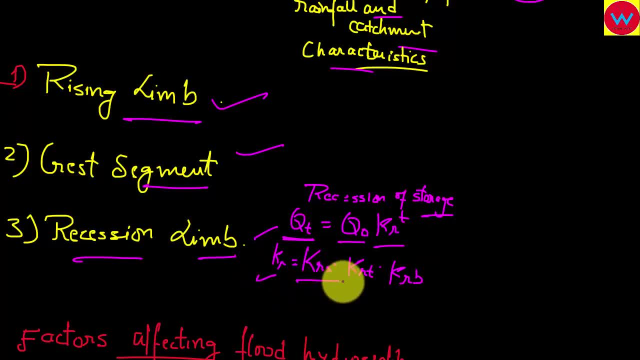 this K R is. K R consists of product of three recession factor, that is, K RS, K RT and K RB. it is our base flow and interflow and surface storage. so recession factor of these three is being multiplied to obtain K R and then K R is used here to obtain the discharge of the 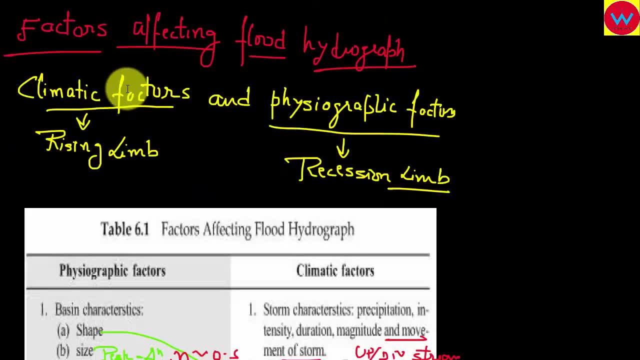 recession limb. now let us look at what are the factors affecting flood hydrograph. we have basically two factors which influences our hydrograph. first is climatic factor and then we have physiographic factors. climatic factor: as I have told you, it affects rising limb. that is, it affects 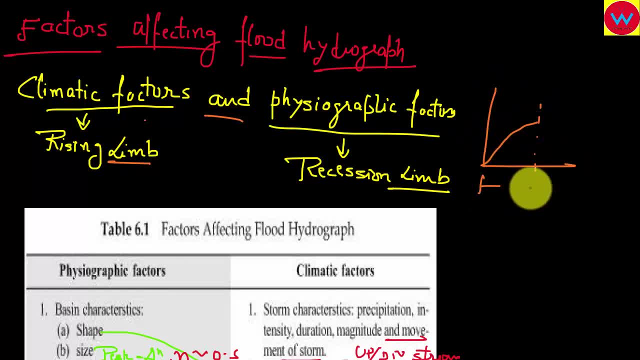 this, this part of our hydrograph, this, this thing which arises. this is affected by climatic factors and physiographic factor affects recession limb. that is this: the recession of storage water is affected by physiographic factors. so this we have. we have physiographic factors. 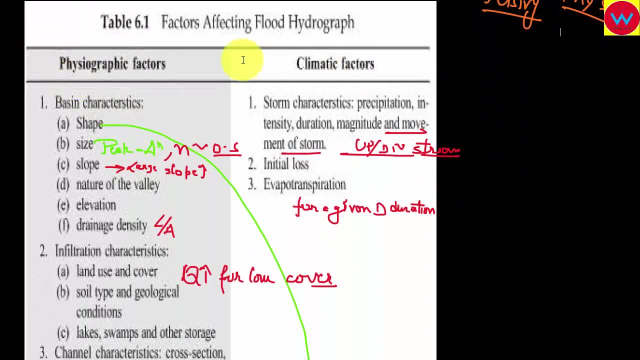 lets see in detail connected to administration of imbalance in fb alphabetic system. let us see in detail what are different physroscopic and climatic factors. physiographic factors means basic characteristic, such as shape, size, slow nature of valley, elevation, then identity. so how does shape of catchment basin effect flood hydrograph? so it is like: 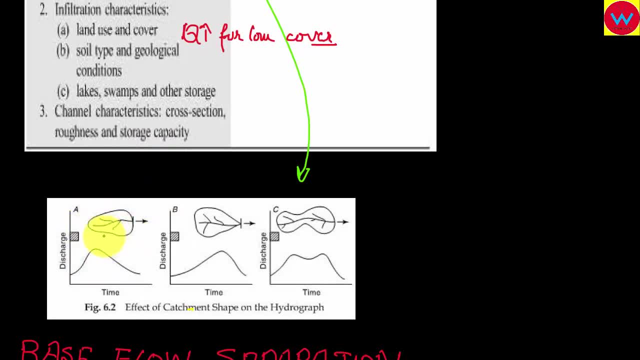 this: if our shape is like this shape of basin is like this, then we have peak. will B be occurring at this place on the completed basin condition or how it could develop in future condition as this which is replace water system. it i can say in future case. so we see in this scenario, which in this scenario where the life actually problems with thisATHG 프로ạie of chain, as the different characteristics, what are different signature factors. after this we also change damithowar at the peak, so we can close thatмент now, as we have in this scenario. so we will see these Brothers in future case as the differences form in how does accessing flow". 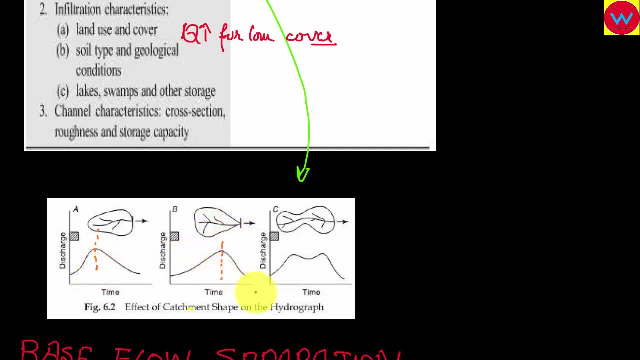 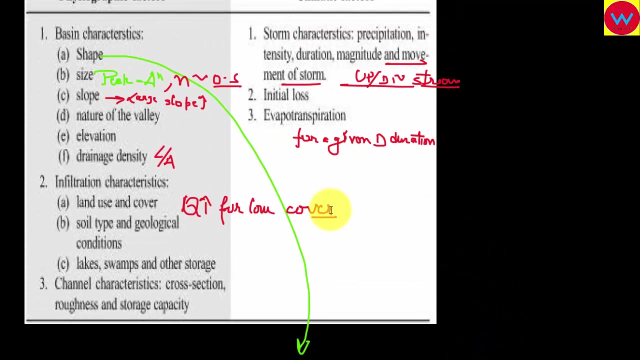 If shape of basin is like this, then peak will be delayed because the water will take more time to reach this outlet basin. If we have shape of our catchment area like this, then there will be multiple peak hydrograph. So in this way peak shape of catchment affect our hydrograph characteristic. This is an important point from view of examination at every level. Now we have size. We know that peak is directly proportional to area. The greater the area turning into stream, greater will be the discharge value and greater will be the value of peak. 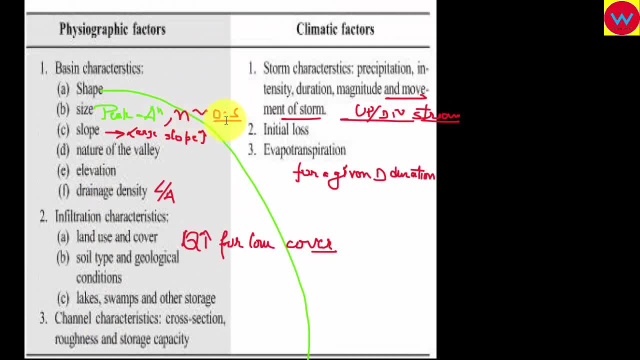 So it is directly proportional to area and where n is exactly equal to 0.5.. Now we have slope For slope, as we can say that the larger the slope, that is, if this is our basin and if this is our second, then in this case the discharge will be greater because the water will be draining off very quickly. 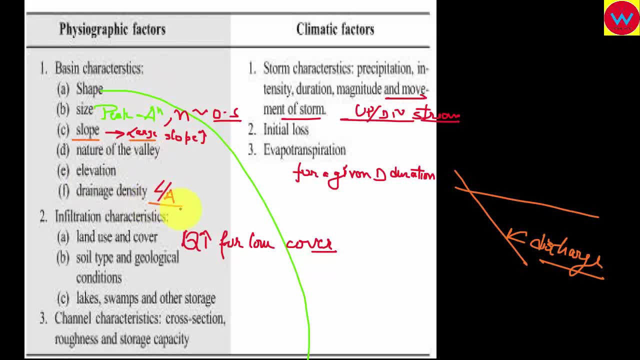 So, similarly, nature of valley, elevation, drainage density And for climatic factors we have strong characteristics. that is, precipitation intensity, duration- If in duration is d is you can say greater than q will be- also be greater and the base of the base of hydrograph will be longer. That is, for longer amount of time we will have this hydrograph and movement of stream. that is if 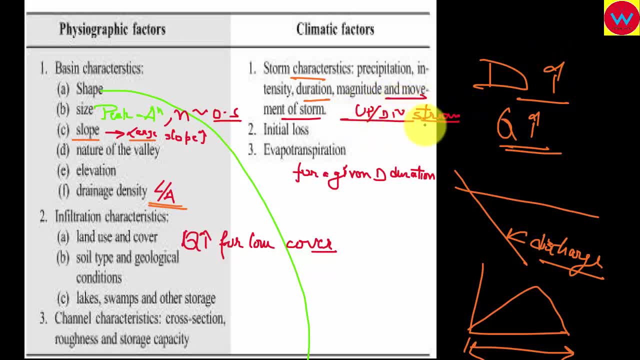 If the storm is moving upstream, and then it means that basin discharge will be, This peak of the discharge value will be less, and if it's moving downward, then peak will be more. There are factors such as initial losses. If initial losses are less, it means that most of the water will be flowing down the valley and we will have higher value of discharge. 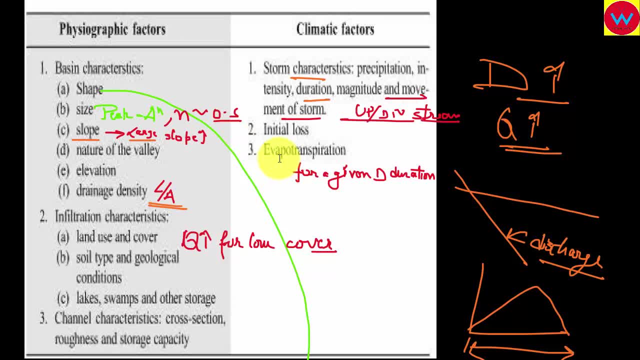 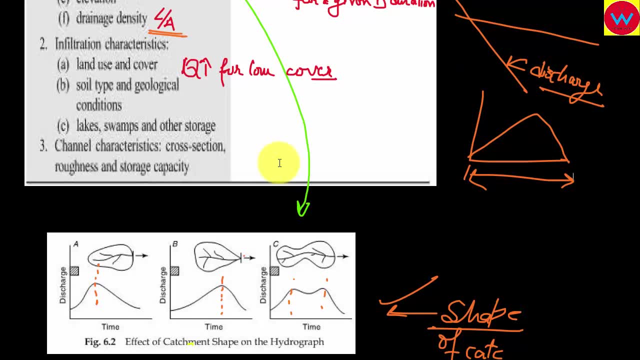 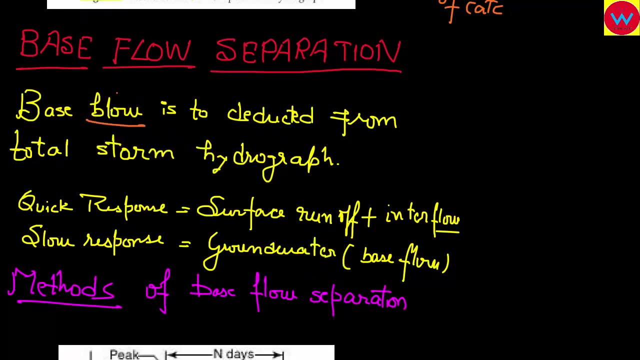 Evapotranspiration in a similar case. if there is a high value of evapotranspiration, then discharge will be higher, The discharge will be less and we will have less peak of value of hydrograph. Now come to the next concept of base flow separation. Base flow separation means that the value of this base flow is to be deducted from total storm hydrograph. 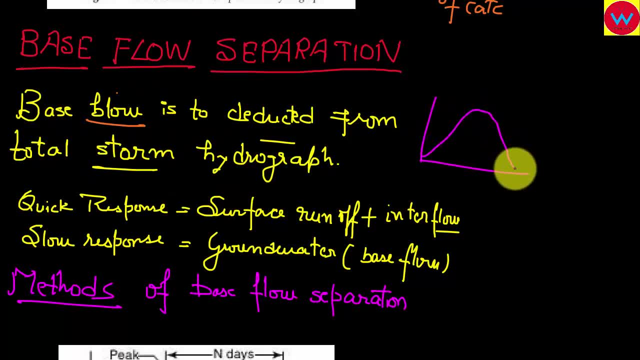 It says that if suppose we have this hydrograph value, then some, for some portion, we will be having our base flow, that is, continuous contribution from groundwater. So we have to deduct this value, this value, from our total hydrograph, total storm hydrograph to calculate, to arrive at DRS, that is, direct runoff hydrograph. 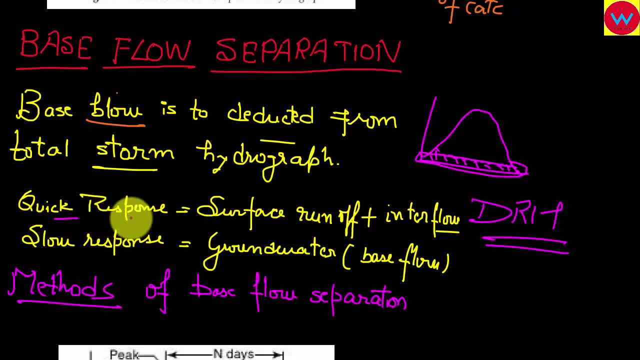 So there are few things in hydrograph, such as: first is quick response. surface runoff plus interflow is called as quick response and slow response, that is, groundwater flow or base flow, is called as slow response, which we have seen in runoff chart How we can measure base flow. 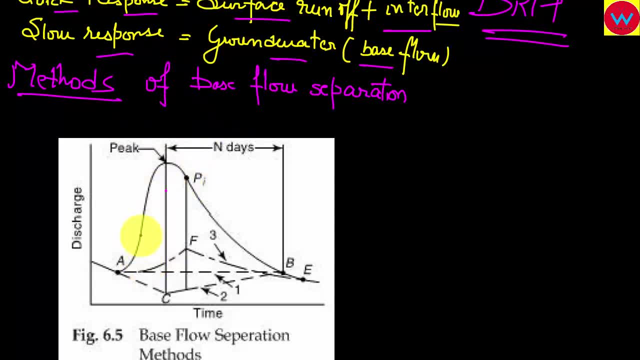 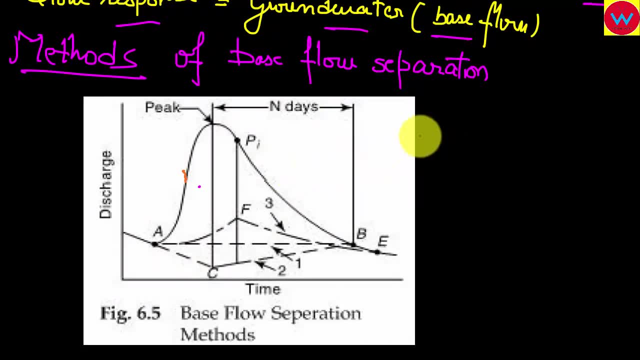 Let us look at it. So this is our hydrograph value, and now we will look at what are the various ways in which we can measure the base flow, or how base flow can be separated from direct runoff hydrograph. This is your direct runoff hydrograph peak. that is starting from here. 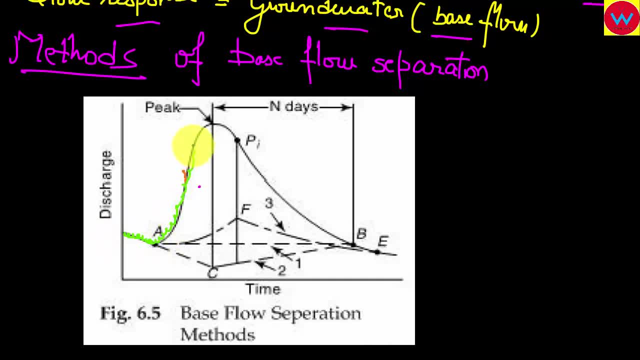 We have this curve as flood hydrograph. This is combination of runoff or rainfall characteristic. Now what we have to do is we have to separate base flow from this flood hydrograph. There are three methods of doing this. First method is that we connect A point and we connect B point. 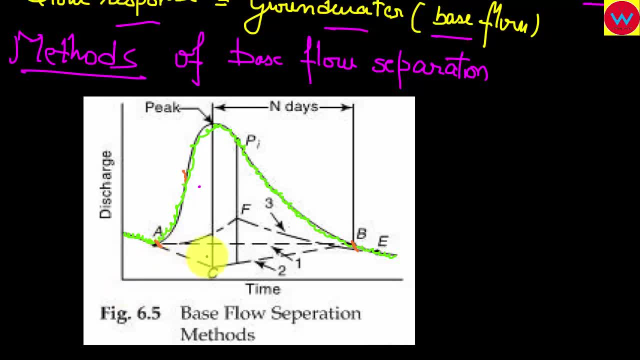 So we all the values below this we remove. then whatever curve we get, we call it as DRH. Second option is that we extend previous slope, That is, we extend this line to this side and then we extend this line to this side, And then we have what we call as second method of base flow separation. 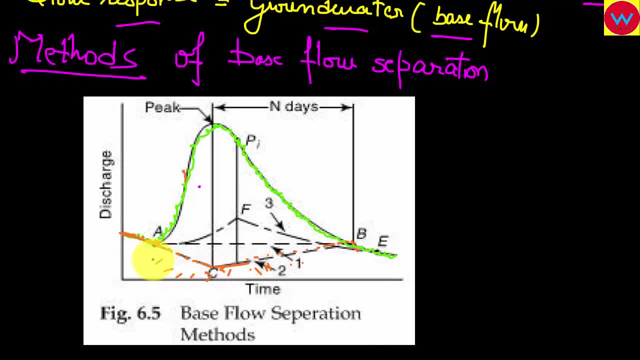 That is, all the water below this line will be called as the base flow. And third is that we draw an inflection point. That is, inflection point is that where slope of this curve changes, that is PI. This is our inflection point. 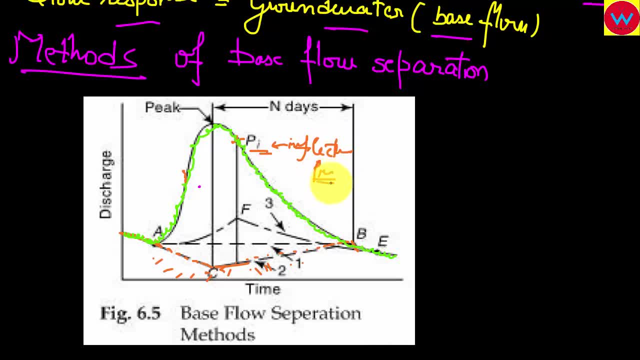 We draw vertical from inflection point and then we make a smooth curve, joining A and B In this process. whatever value we get below this line, we separate it as base flow, And whatever value we get above this line, we call it as our direct runoff hydrograph. 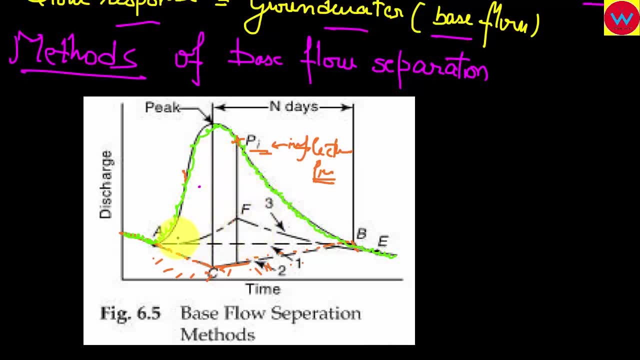 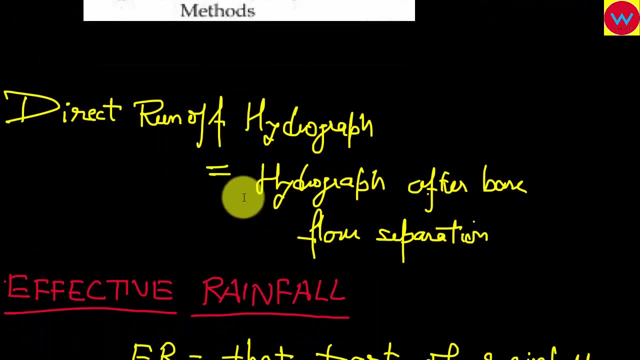 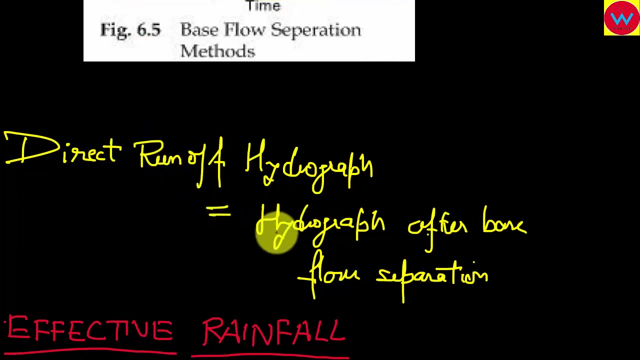 So these are two, three methods for obtaining base flow, But most common method is this, That is, we join A to B and all the water below this line is called as base flow. Direct runoff hydrograph is that hydrograph which is calculated after base flow separation. 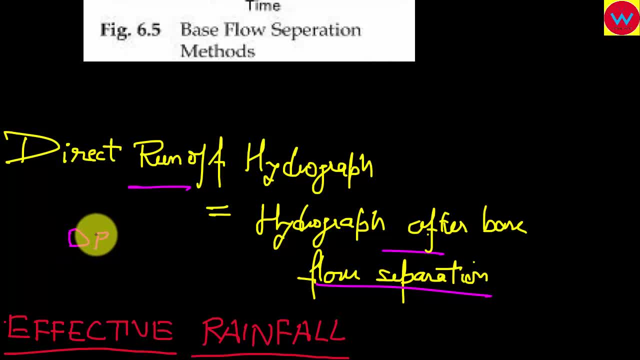 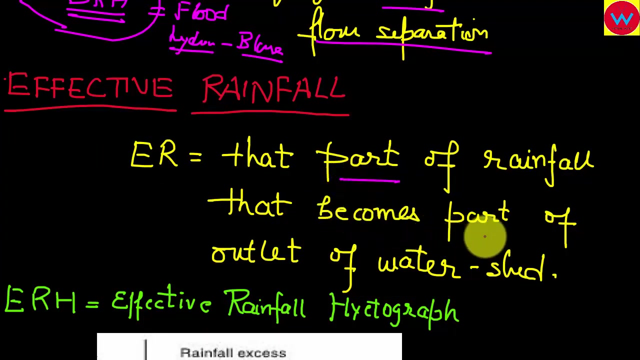 So we call it as DRH. DRH is your flood hydrograph: Flood hydrograph minus base flow, That is this. DRH is basically hydrograph obtained only through direct runoff values. Effective rainfall is that part of rainfall which becomes part of outlet of watershed. 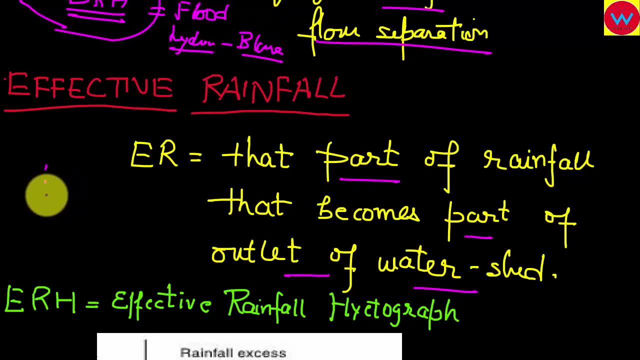 That is. We have seen that if rainfall is taking place, then- and this is our ground surface- It does not mean that all the water will come down or go down the slope. Some water will be intercepted, some will percolate, So effective rainfall is that part of rainfall. 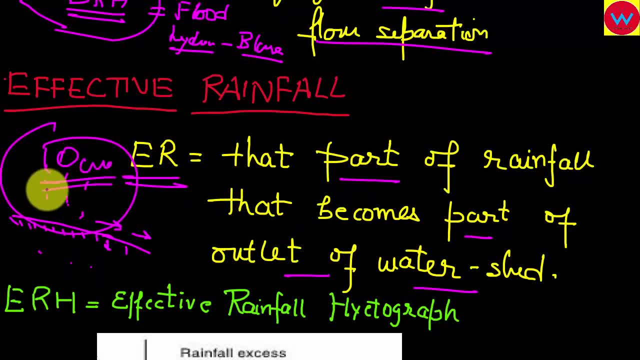 That part of total rainfall- suppose 10 cm of rainfall is taken place. It is that part of rainfall which becomes part of outlet, That is, which goes as a runoff, basically, and becomes the part of outlet of our channel, Our channel here. So that is known as effective rainfall. 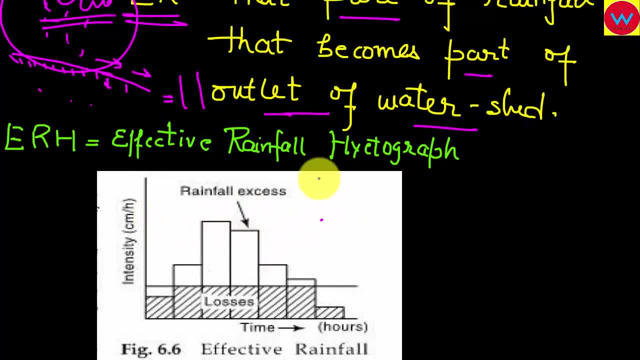 Now we have effective rainfall hydrograph. It is that hydrograph. Hydrograph is basically plot of intensity versus time, Basically cm per hour, intensity versus time. So ERH is effective rainfall hydrograph, DRH is direct runoff hydrograph. You can see the difference here. 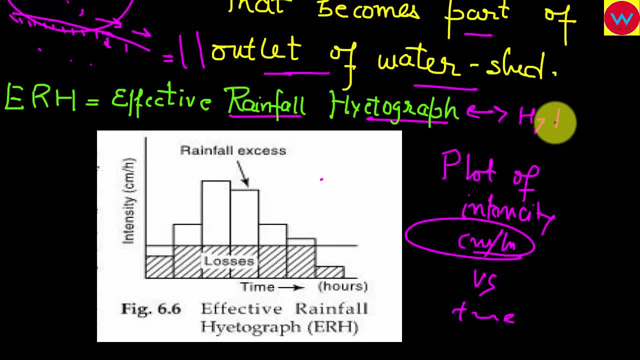 It is hydrograph And what we are dealing is hydrograph. That is, this is hydrograph. In hydrograph we have intensity. In hydrograph we have volume That is meter cube per second, And here we have cm per hour. That is our intensity. 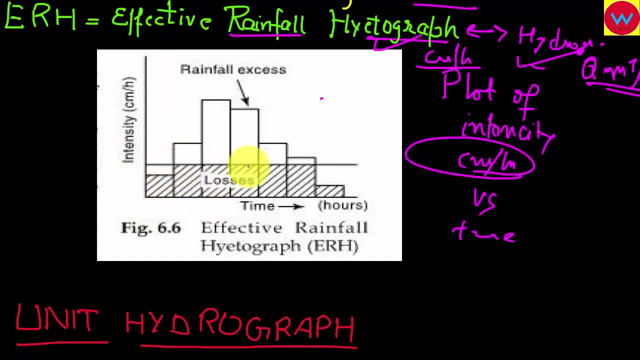 So in this case also we draw. We have seen in our first or second lecture that is called as phi index. That is, through phi index you can. You can separate losses and then calculate effective rainfall, That is, that part of rainfall which directly contributes. 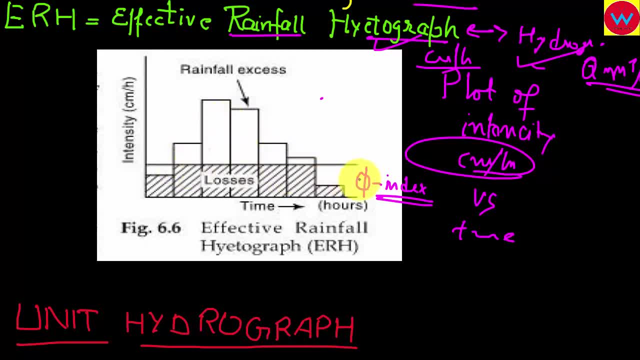 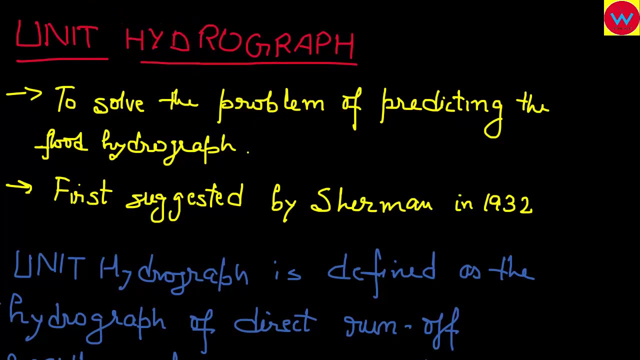 Which becomes part of runoff. So you have to calculate phi index. You can refer to previous chapters to know about how we have calculated phi index. Now come to next concept, which is a very important concept, Which is called as hydrograph or specifically, unit hydrograph. 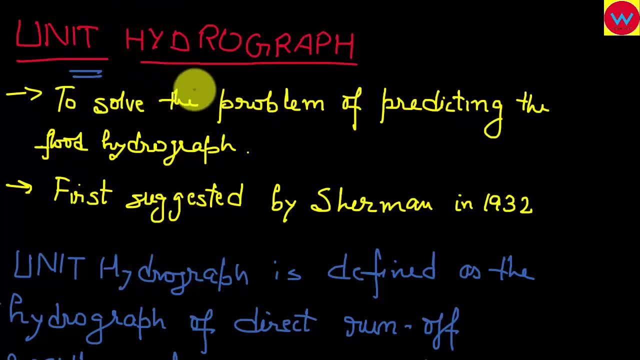 Unit hydrograph. Unit hydrograph is used to solve the problem of predicting the flood hydrograph, That is, we do not know the response of catchment for severe storms or rainfall. Then we can deploy unit hydrograph to predict how the catchment will behave for given rainfall or for the given catchment characteristics. 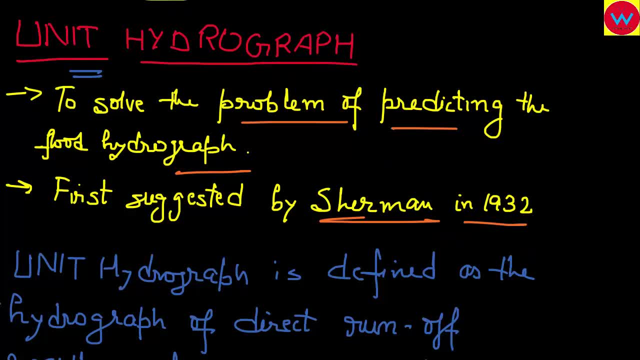 It was first suggested by Sherman in 1932. And since then it has been used extensively in the ground by the, By the water scientist and in hydrology departments of various governments and for predicting various rainfall and runoff characteristics And how the flood is going to behave for the given amount of rainfall. 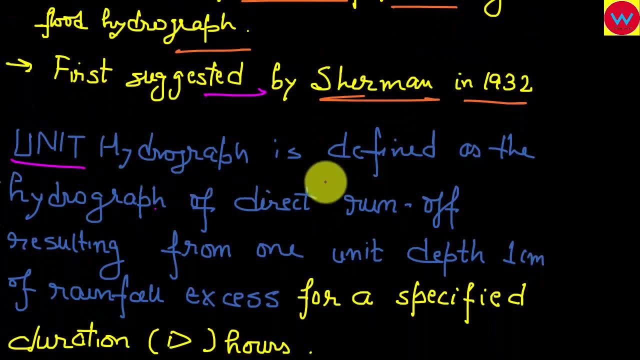 So let us define the unit hydrograph. Unit hydrograph is defined as the hydrograph direct runoff hydrograph Resulting from one unit depth, that is, one centimeter of rainfall access for a specified duration of d hours. This is definition. Now you need to understand this definition. 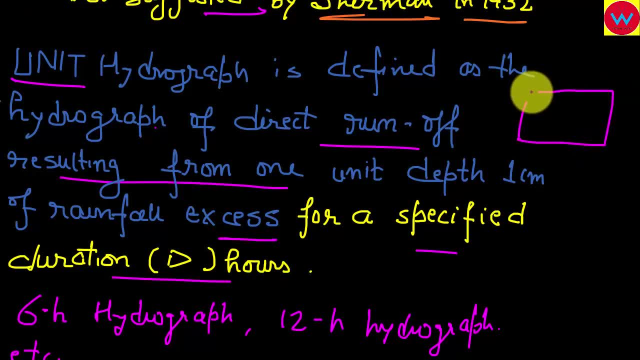 So let us say that we have an area A here. This is our area. Okay, On this area A, I have rainfall falling. This is my rainfall here on this area, R is my rainfall. So rainfall started from time t is equal to 0 and it ended at time t is equal to 4.. 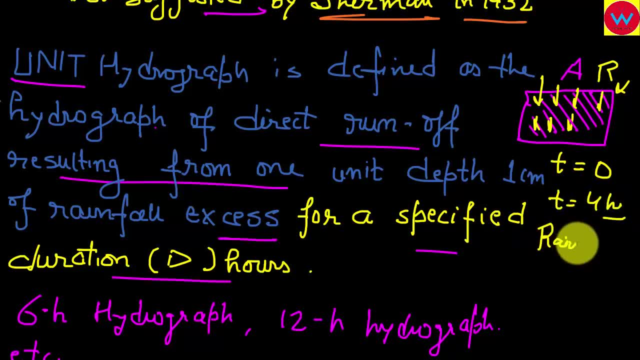 So what? I will say that rainfall was of t hour duration, 4 hour duration. So in this d we have, d is equal to 4, that is for duration of rainfall is called as d hour or 4 hour, whatever the value may be. So unit hydrograph: 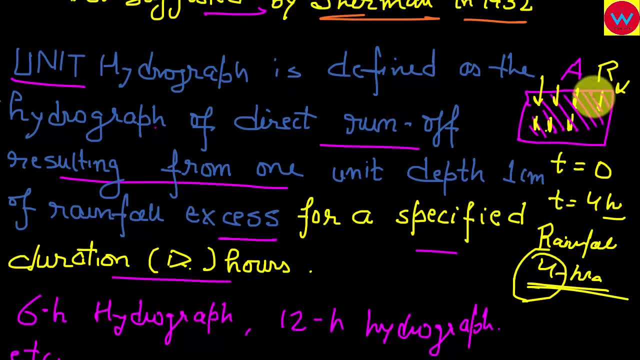 This is that The runoff, direct runoff, from this area is one centimeter, That is unit. depth of rainfall is has taken place on this area And the hydrograph resulting from that case will be called as the unit hydrograph Unit means rainfall access is one centimeter. 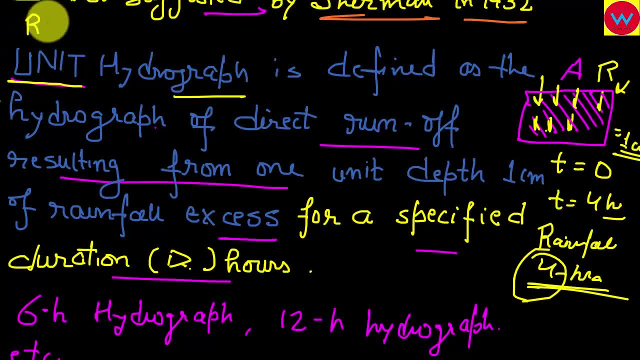 Basically the concept is that rainfall access is one centimeter over that for any given area And we have to plot hydrograph corresponding to these conditions And when hydrograph is plotted it will be called as unit hydrograph. So how we use unit hydrograph, that we will say that suppose for 5 centimeter of rainfall. 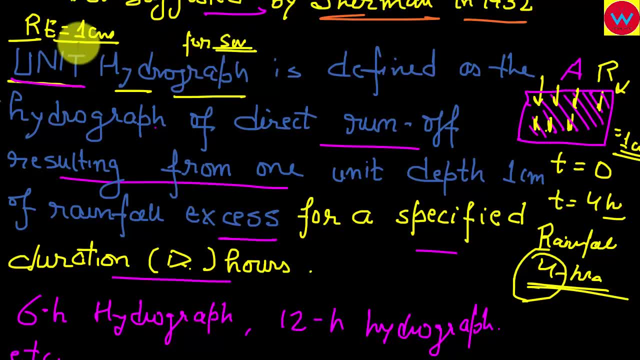 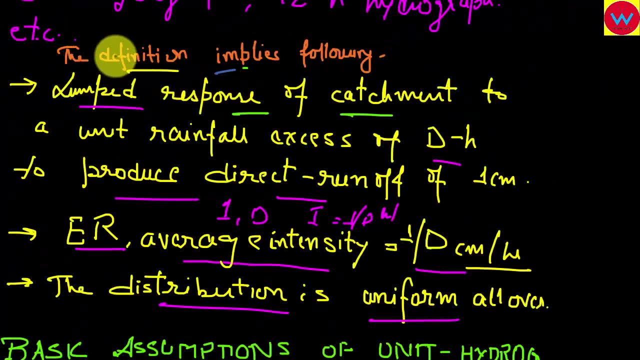 We will multiply all the coordinates by 5 centimeter, because we know the value of 1 centimeter. Let us look at the other properties of unit hydrograph. Let us once again look at the definition of hydrograph and what does it imply. 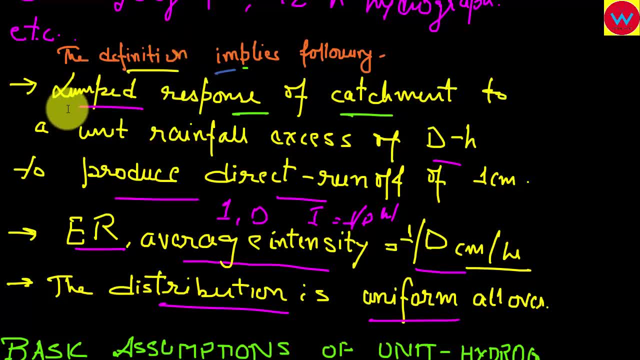 So, first of all, the definition of hydrograph implies that The rainfall- effective rainfall of one centimeter gives the lumped response for that given catchment. That is, our effective rainfall is one centimeter If this much of rainfall takes place for d hour duration. 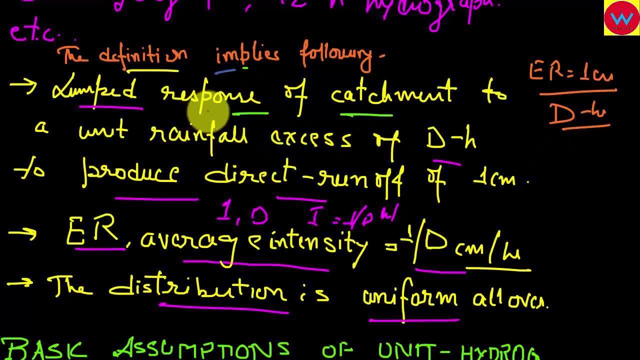 Then the hydrograph will be a response. Response means how the catchment, what are the catchment characteristics, Its slope, length, size and distribution of vegetation, etc. So the hydrograph gives the response of a catchment for a given rainfall axis of d hour duration. 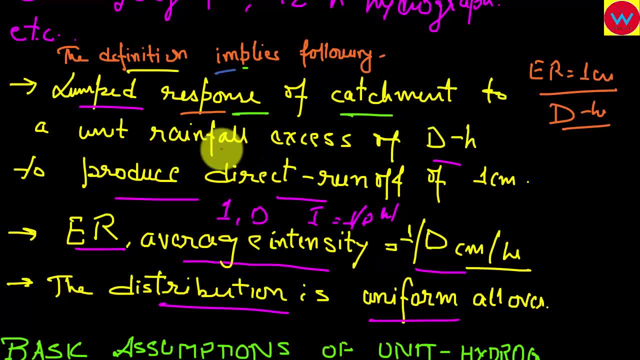 And the rainfall axis is one centimeter. That is why we are saying that it is a unit hydrograph or like that. So if our rainfall axis is one centimeter and duration is d hour, Then its intensity will be 1 by d centimeter per hour. 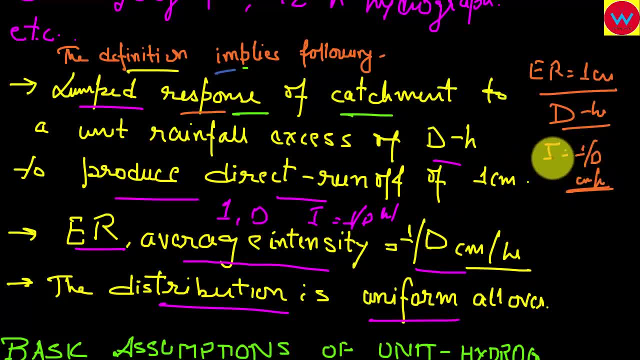 That is. intensity is how much amount of rainfall is falling per hour. Then it will be calculated like effective rainfall divided by total duration. That is the average rainfall intensity. we can say Average I. The distribution is assumed as uniform for all the catchment area. 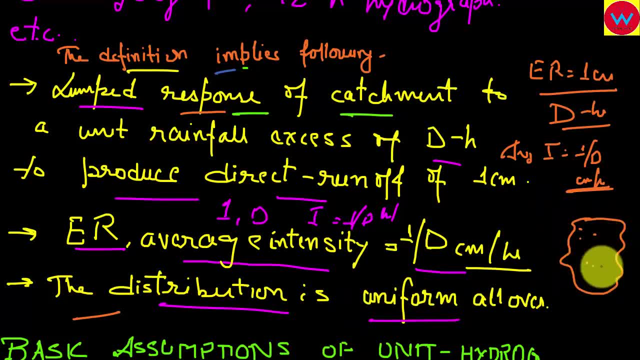 That is, if your catchment is like this, Then it is assumed that rainfall is evenly distributed. But it is not the case, Because in most of the cases- suppose your catchment area is like this- Then rainfall will take place only at these areas. 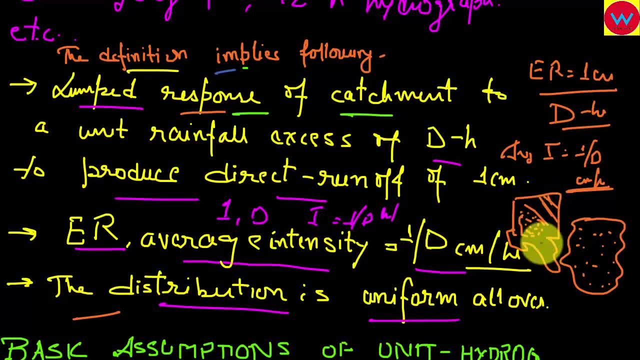 And this much area will be left out from rainfall distribution. So in that case our this assumption will give us an error. But for all practical purposes we have to assume Then only we can proceed with the simple hydrograph. Now we let us see that. what are the basic assumptions in unit hydrograph? 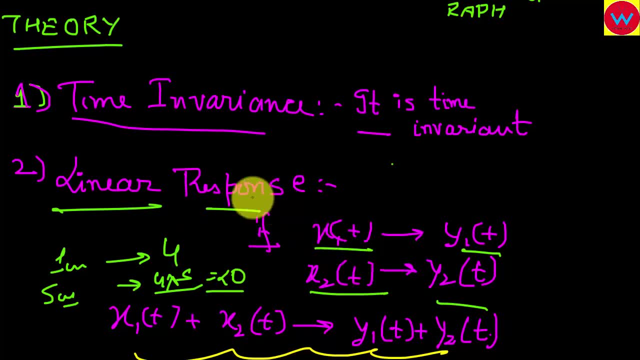 First is that if this, our hydrograph, is time invariant, It means that it does not matter when the rainfall takes place, Either it takes place in particular time of the day or month, or any season. The catchment will give the same Response for a given duration. 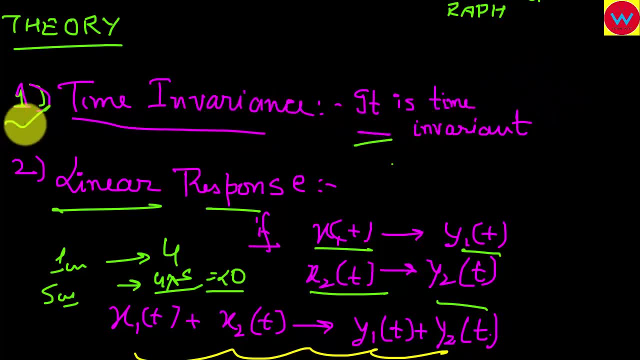 And for effective rainfall. So first is that it is time independent. Second is linear response. Linear response is that, as we have seen earlier, that for x amount of time at x, At x coordinate we have y1 value and x2 coordinate we have y2 value. 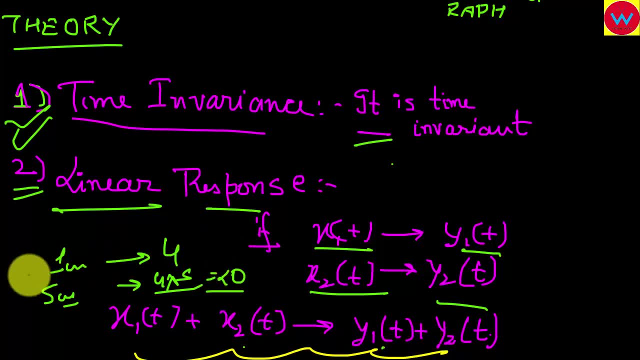 Then x1 plus x2, we will give y1 plus y2.. So if our effective rainfall is 1 centimeter, As I have told you earlier, And my y coordinate is 4. Then for 5 centimeter effective rainfall it will be 20.. 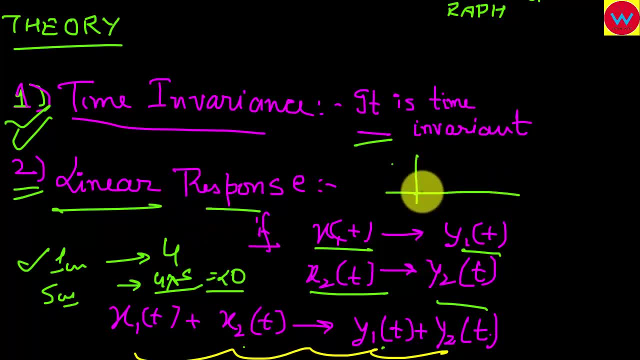 Basically what you see. that suppose this is your hydrograph number 1. And this is your hydrograph number 2.. So for same d hour duration, rainfall We can superimpose. If your base is same, You have to make same of your base. 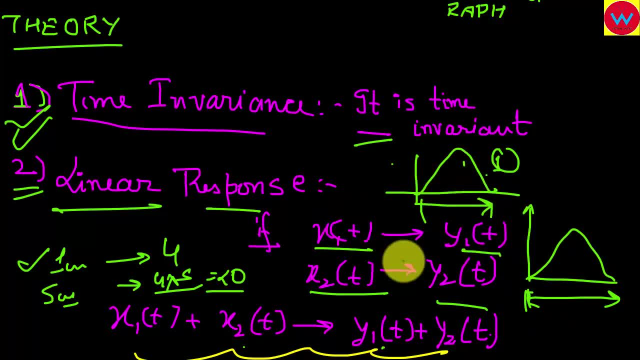 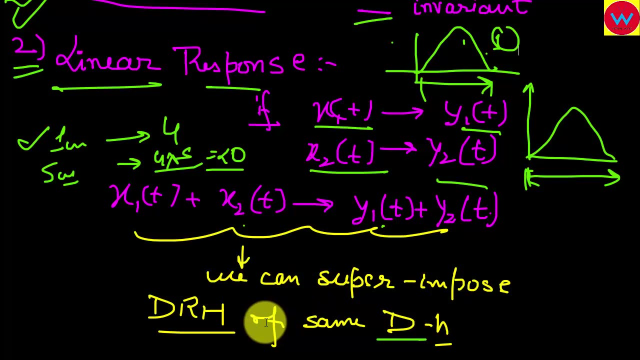 Then you can superimpose these two hydrograph And The resultant hydrograph will be The sum of these two coordinate corresponding coordinates. But one thing we have to keep in mind: that We have to superimpose direct run of hydrograph of same d hour duration. 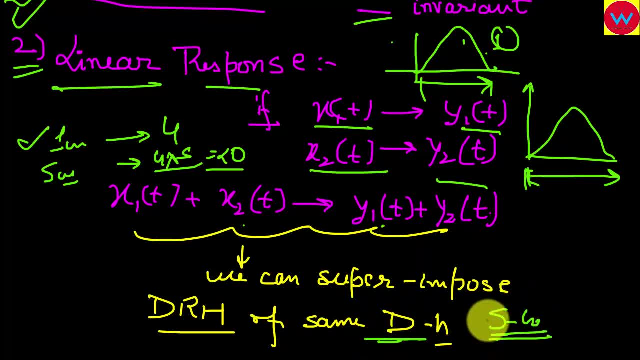 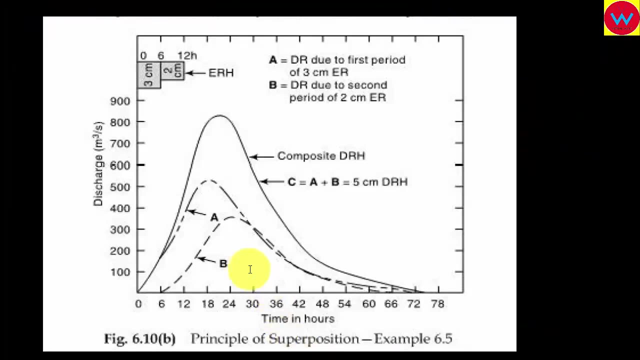 That is suppose 5 hour duration rainfall We can superimpose for only in this case only. But if we have 5 hour and 4 hour rainfall We cannot superimpose. It will not be valid in this thing, As I have told you earlier that. 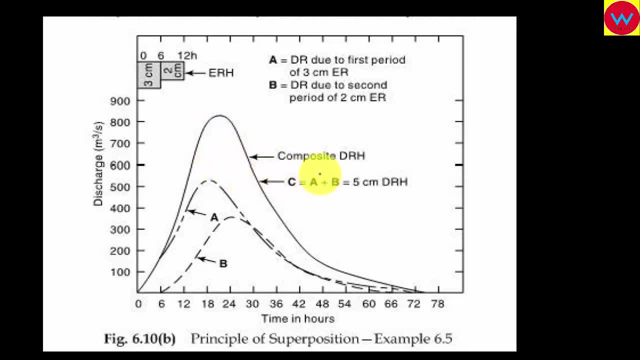 We can superimpose hydrograph for same d hour rainfall. This graph is an example of our assumption earlier. Your a hydrograph is direct runoff due to first period of 3 centimeter effective rainfall. That is this one. Now, after that, we have 2 centimeter of effective rainfall. 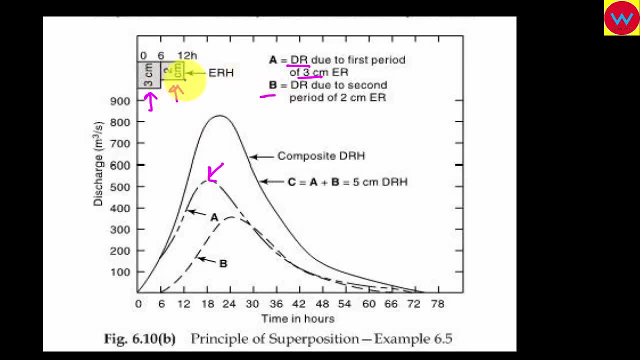 Another rainfall of 2 centimeter of, Which has 2 centimeter effective rainfall But same duration, That is, 6 hour duration. You can see here that Our first rainfall is 0 to 6.. 6 hour And second rainfall is 6 to 12.. 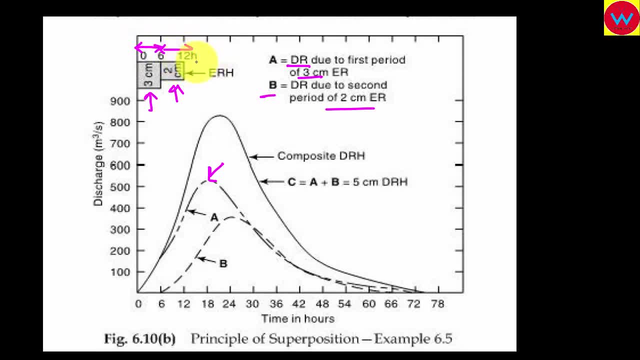 Then again, duration is 6 hour. So what we have done, We have plotted a and b separately And then, in order to show the effect of these 2 hydrographs, We have joined the ordinate. We have to do the summation of these 2 hydrographs. 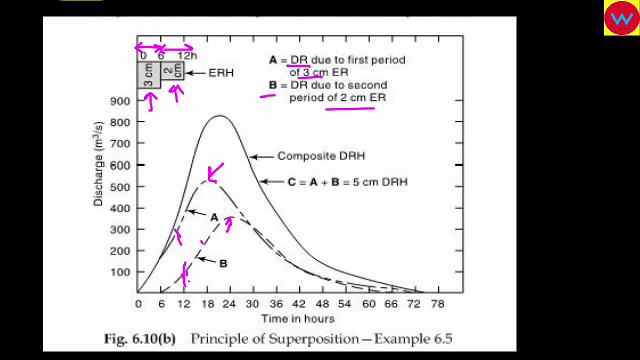 To obtain this composite direct runoff hydrograph. That is suppose at 18 hour time. If your ordinate this is y1. yb, let us, And this ordinate at this will be ya. Then ordinate for composite drh will be equal to. 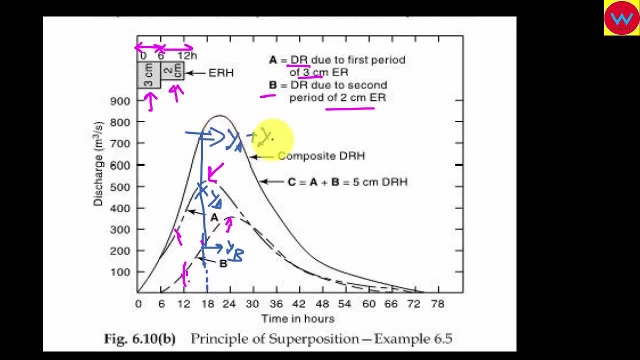 We have seen ya plus yb. So this graph is an example of our assumption that we have studied earlier That for the same dr duration- rainfall, We can do the summation of given hydrograph And the net hydrograph will be a composite hydrograph. 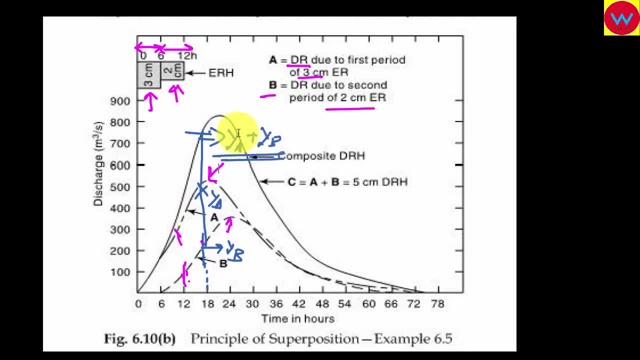 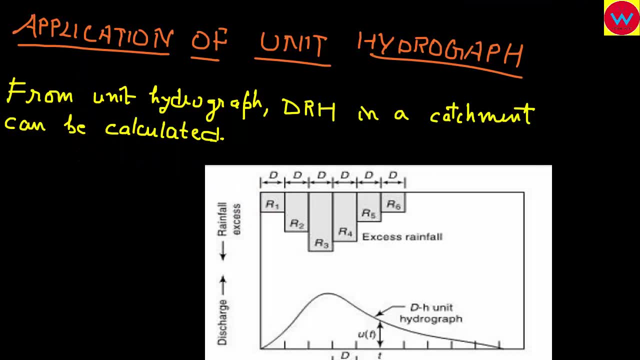 And it will be a valid one. Now let us look at what are the different application of Direct runoff hydrograph Or, specifically, What are the application of unit hydrograph To be more precise, Because in most of the cases We do not know in advance? 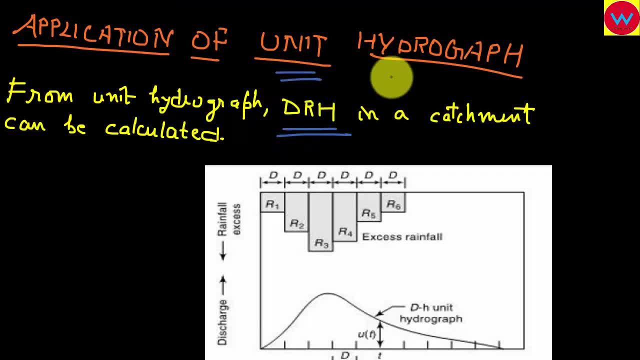 The drh for a given storm. We only know unit hydrograph And then we calculate the drh for the given rainfall axis. So the first application is written Like that: from unit hydrograph We can obtain drh for the given catchment. 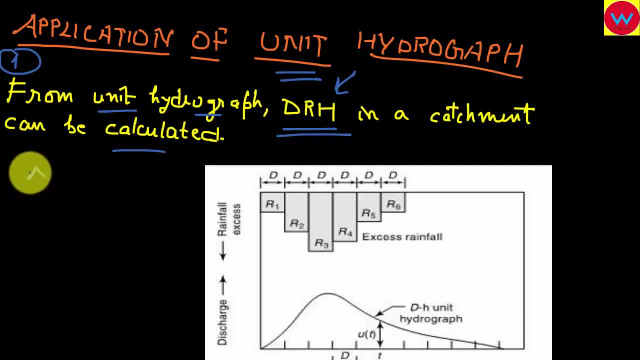 That is, for example, We have a catchment area A. Let us suppose that we have a catchment area A And we know the unit hydrograph. This is: let us say That we have our unit hydrograph. Unit hydrograph is not complete. 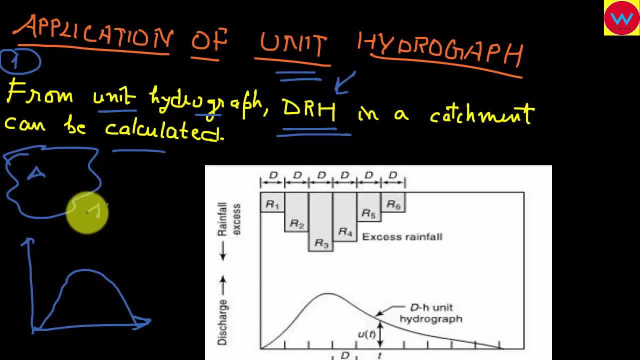 Without mentioning the duration of rainfall. So let us say We have 4 hour unit hydrograph. So if we want to know How much will be, What will be the discharge? Discharge When 4 hour unit hydrograph Of 10 cm. 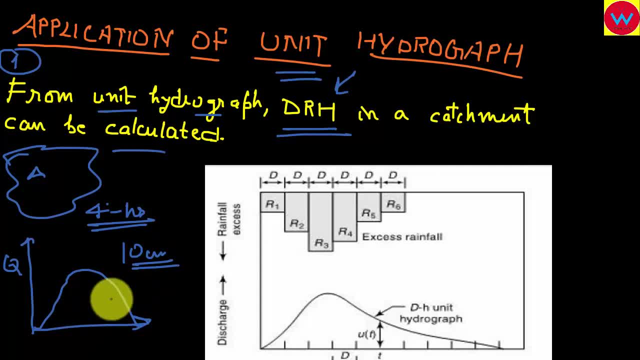 Excess rainfall Comes for that catchment, And what we will do Is that we will multiply all the ordnance Of this hydrograph by 10. Because in our assumption Of this hydrograph, We have taken rainfall axis. 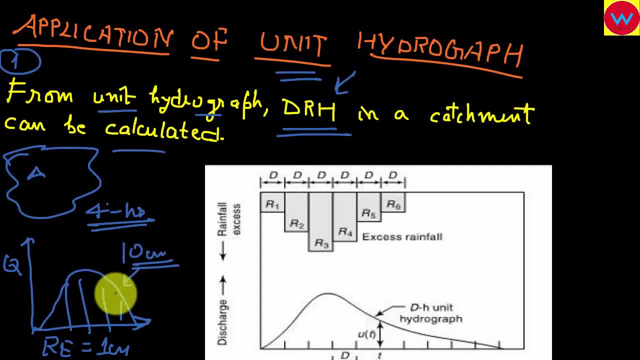 As 1 cm. So in order to get the rainfall axis Or discharge Discharge value for 10 cm Excess rainfall, We will be multiplying all the ordnance by 10.. That is the assumption That we have seen earlier. 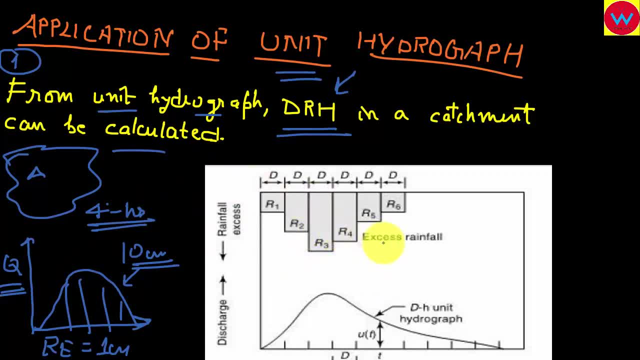 So This is our This graph. What does this graph shows? It shows that It shows direct runoff hydrograph Due to an effective, Effective rainfall hydrograph. That is Here. we have Our unit hydrograph. That is for. 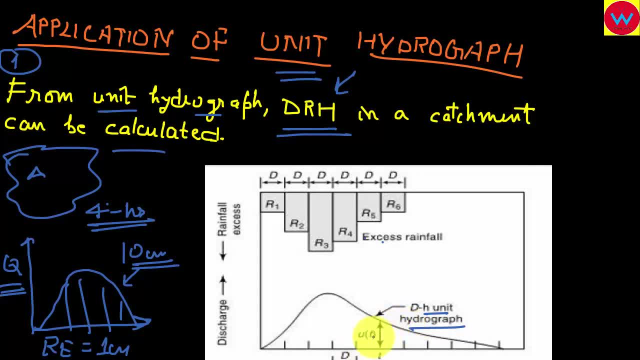 A function. Let us say that We have UT, That is, Unit hydrograph ordinate for At given time, T. So for What does this? What does this? So what does We know? What do we know by? 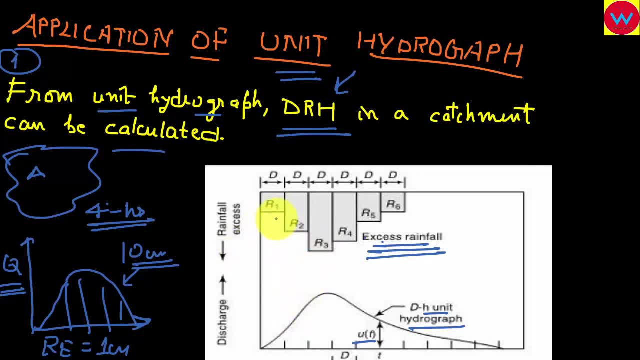 This graph. What we can do Is that we can. Here we have D hour And We have D hour rainfall. Rainfall access is R2.. Again, again, again. We have divided all the Given Given rainfall into. 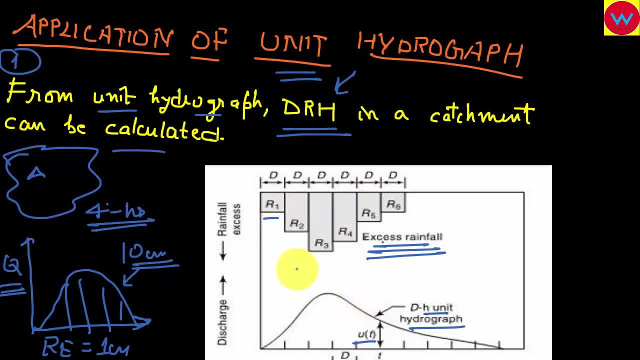 D hour duration, Rainfalls, And we have calculated rainfall access in that D hour duration. And now what we have done, What we will do Is that we will multiply D by, We will multiply And then we will superimpose. 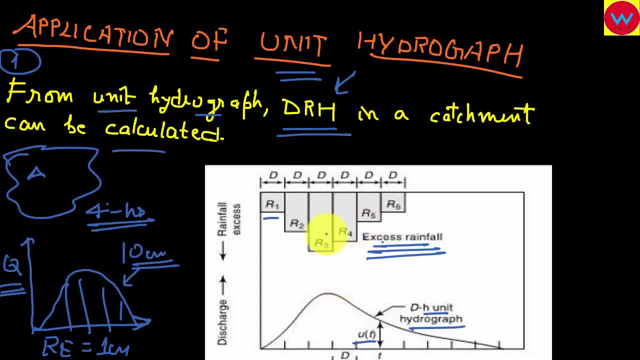 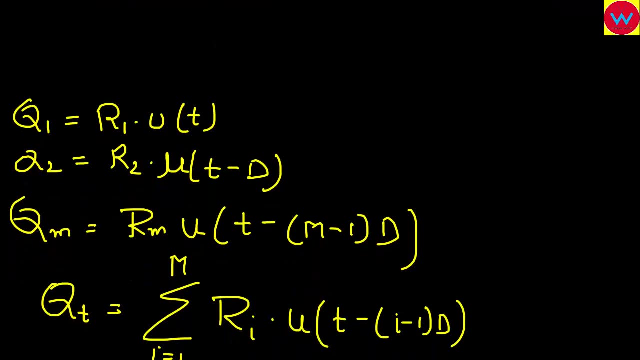 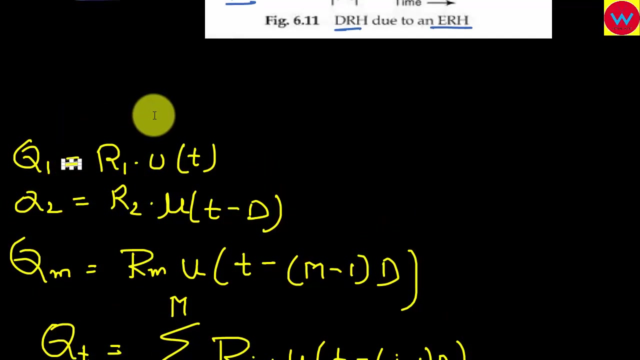 All the graphs to obtain Our D hour Unit hydrograph, To obtain our actually Direct run of hydrograph from this. So, how It is done, We will look at it in terms Of some Algebraic equation, For example, our discharge at. 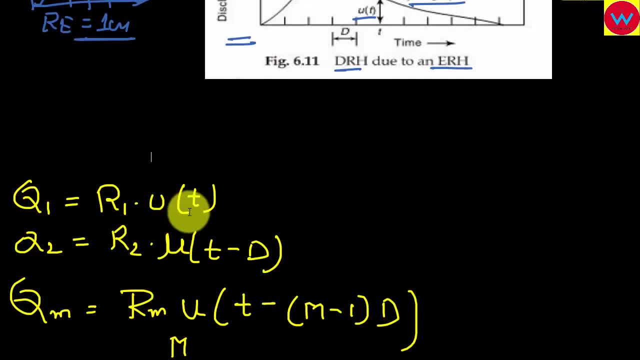 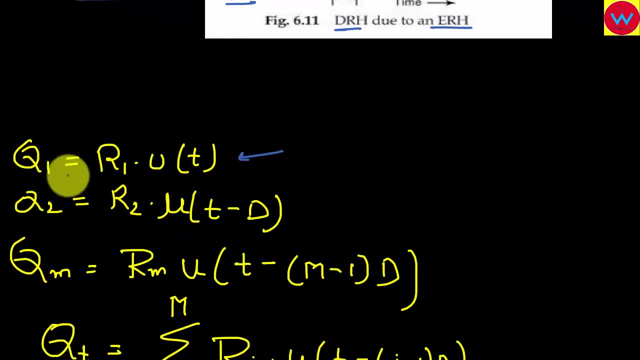 Interval one will be equal to R1 into unit hydrograph Ordinate at time t. You need to understand this equation That it says that Discharge due to Rainfall access of R1 at time t Is given by this, because 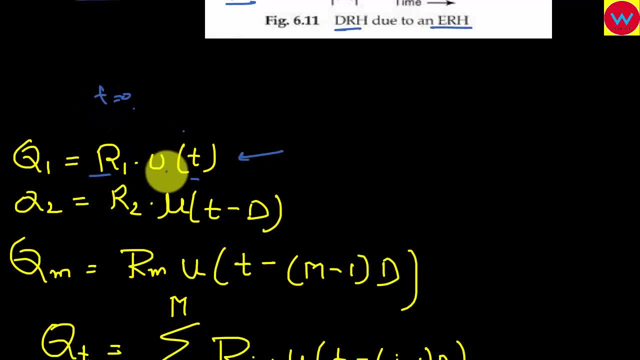 This rainfall access starts from. Time t is equal to zero. therefore, For time t, whatever the ordinate is there, It will be ut For second discharge, that is, discharge Due to rainfall access of R2.. It will be equal to The ordinate. 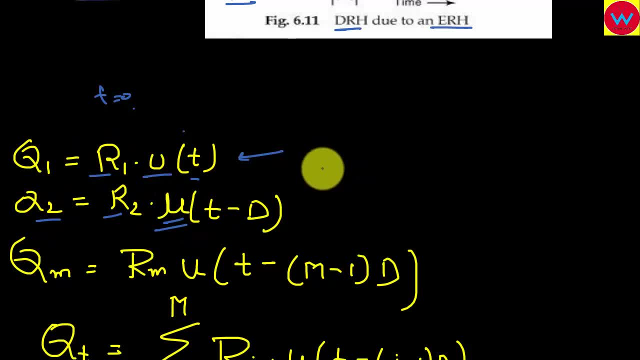 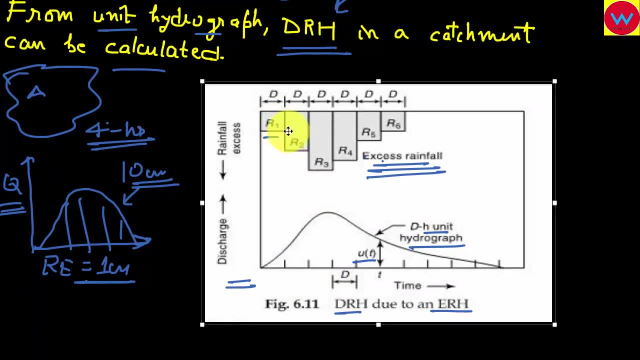 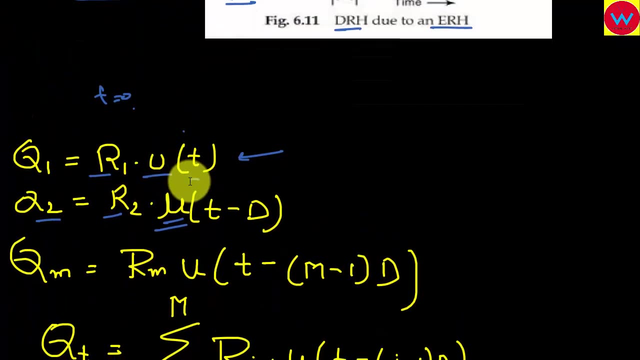 For unit hydrograph because The rainfall R2 starts From After The rainfall R2 starts like here You will see, rainfall R2 has started from T zero plus D hour, that is, D time after R1.. That is, if R1.. 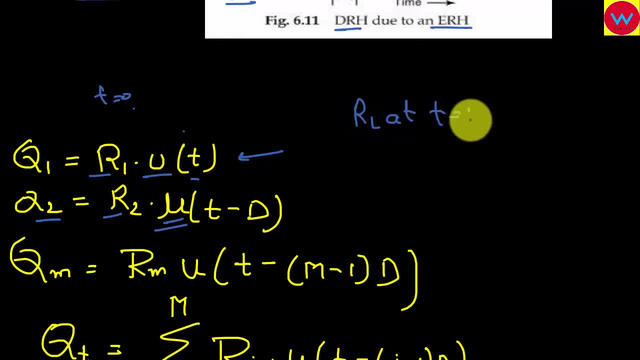 R1 starts at T is equal to zero, Then R2 will Start at t is equal to Zero plus d, And R3 will start at T is equal to zero plus 2d. So what we will do that. 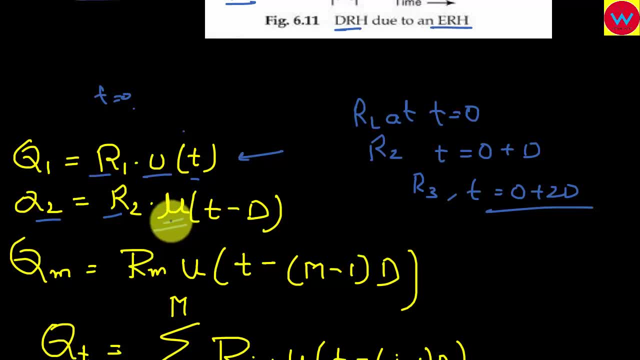 For finding corresponding U ordinate value For unit hydrograph. we will be Subtracting d ordinate From, As per our requirement. So q1 will be like this, q2 like this. Similarly, qm Will be like this: so 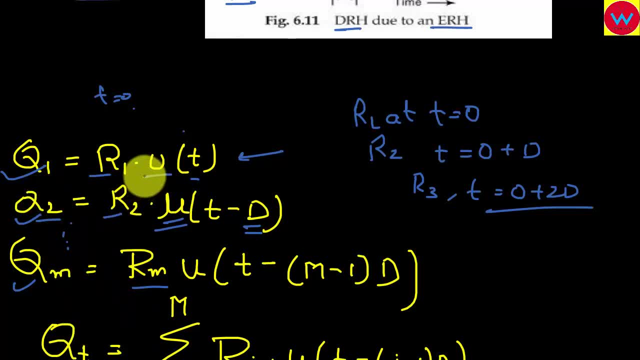 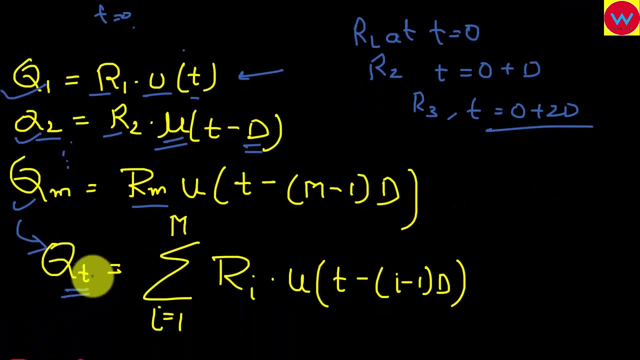 If we do the summation of All the discharge value Due to their individual Rainfall axis, That is, R1, R2, Rm, Then we will get qt. qt is the value of discharge At time. t- qt is the value of discharge. 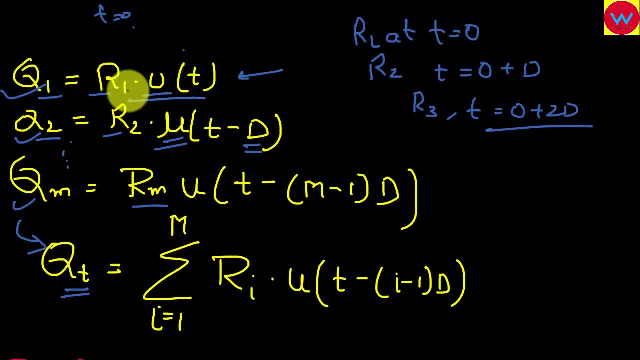 At time t. For discharge value 1, it will be Simply rainfall axis into Ordinate of unit hydrograph. For discharge value 2, it will be rainfall axis into Unit hydrograph ordinate At t minus d time, Because I have told you that. 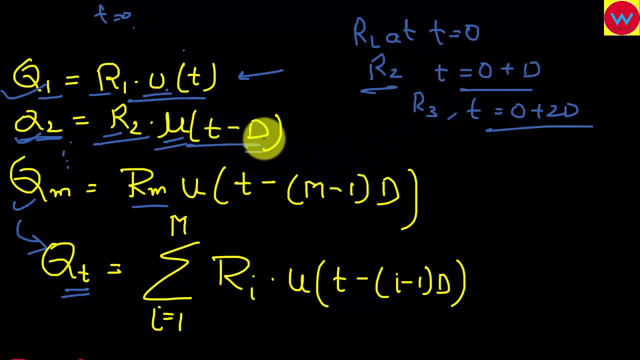 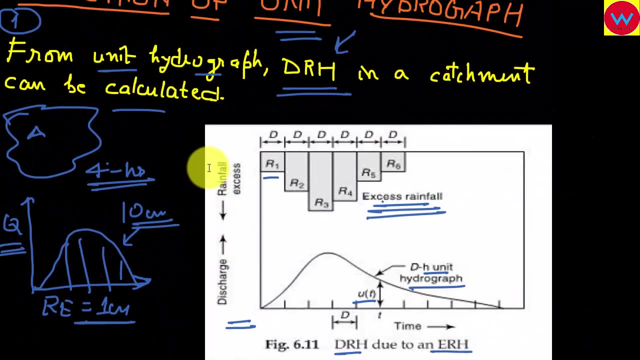 R2 starts from 0 plus d, Our duration. Therefore, we have to subtract d from t In order to Make it corresponding To time t. I think you have Understood this thing that We can calculate Direct Run of hydrograph. 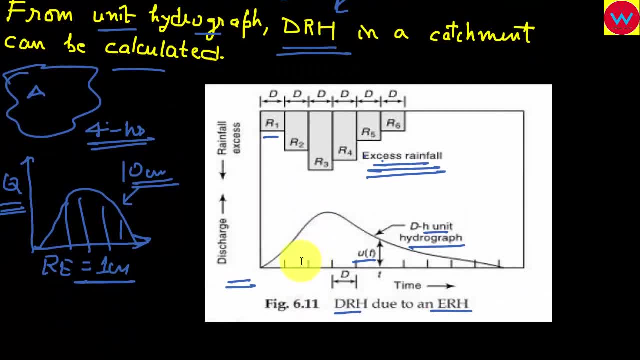 From unit hydrograph, That is, by multiplying Rainfall axis By the ordinate of unit hydrograph. As simple as that. But only thing You have to care about is that Please add the ordinate For their corresponding Values. 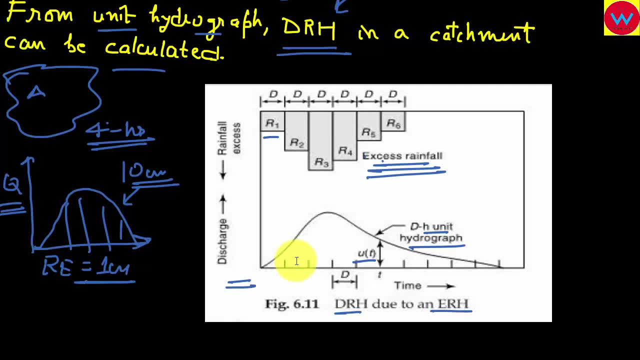 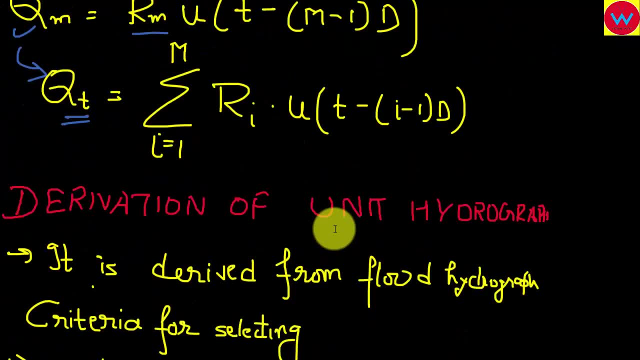 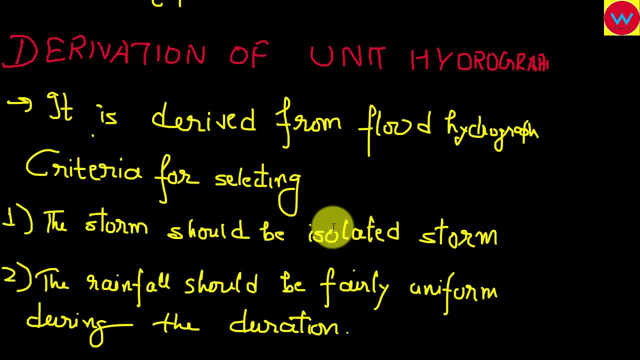 And shift the Shift, your Different rainfall axis With respect to your time interval. That you have assumed. Now, next thing We will See is a very important Concept in hydrology: We are going to look at How hydrograph. 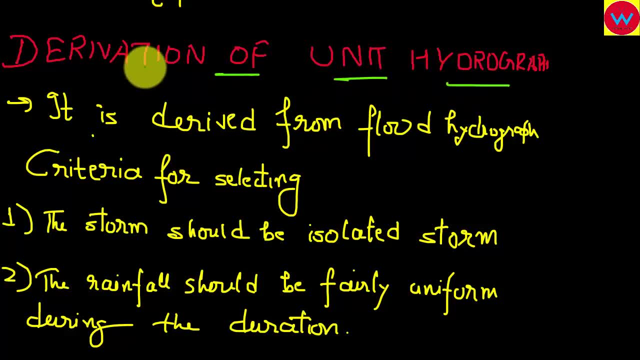 Is derived. That is how unit hydrographs are made, And after You gain the knowledge Of making unit hydrograph, You can make all type of direct run of hydrograph And from there You can do all sorts of thing. So what you can do, 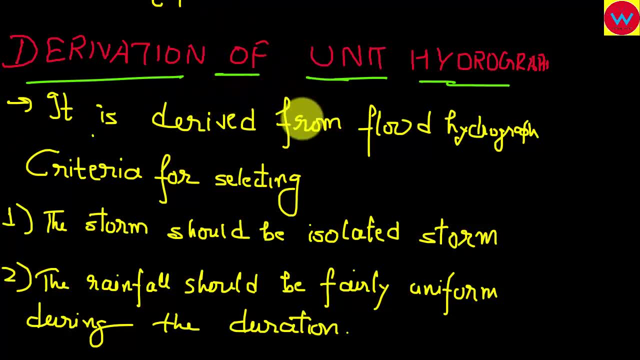 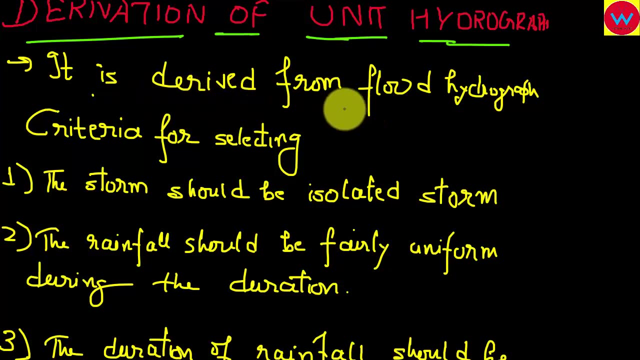 What are the benefits of Unit hydrograph, How it is done And what are the assumptions For calculating unit hydrograph We will be looking at very shortly. So It is derived from flood hydrograph. First of all, you have to. 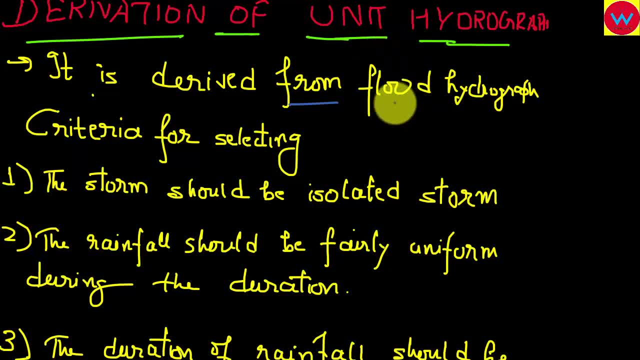 See that For calculating unit hydrograph You need to have flood hydrograph, That is, you need to have data Of discharge versus time For a given flood. Then only you can calculate Flood hydrograph By separating base flow, Which we will look very shortly. 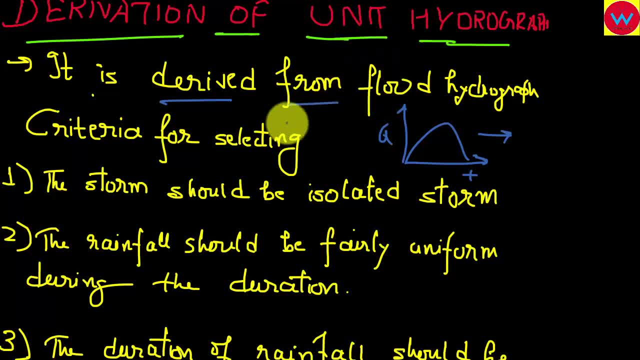 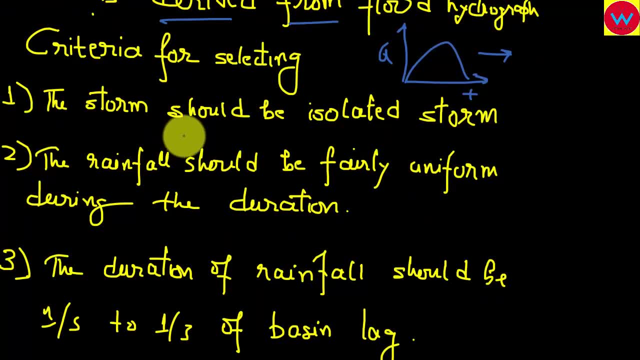 But first thing is that You need to calculate flood hydrograph. In order to calculate unit hydrograph, You need to have actually data from field. And how do we select which Which flood hydrograph data to take? It is the There are certain criteria. 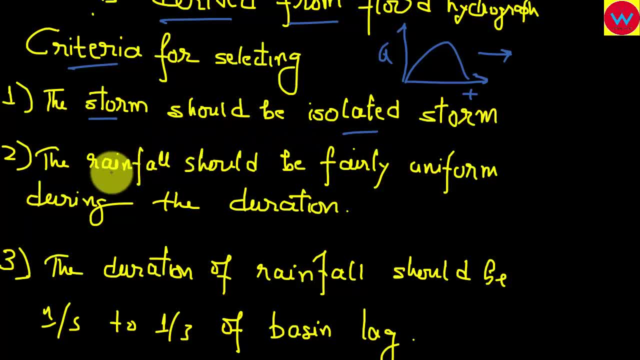 First is that the storm should be isolated storm, And that is, It should not occur in conjunction With other storms. Other storms are taking place nearby Or other similar events Should not be in association or conjunction With the given storm, So it should be an isolated one. 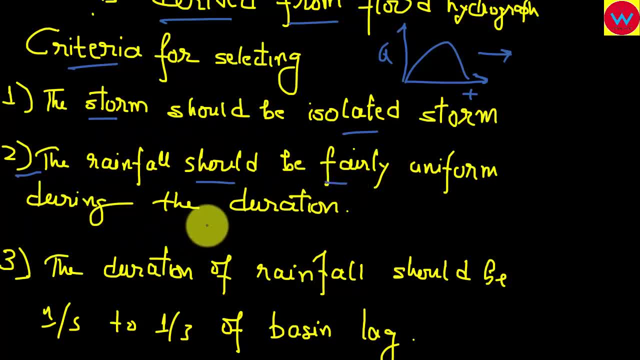 Second is that the rainfall should be Fairly uniform during the duration, That is, You know that Rainfall intensity- And it is In other Rainfall characteristics- Should be uniform And it should be spread over All Over all the catchment area. 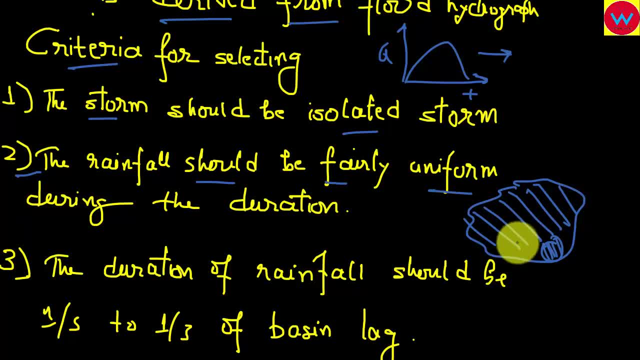 It should not be localized Like this. It should have uniform distribution Of rainfall And The duration of rainfall should be One fifth of To one third of basin lag. That is We. This is an important concept, Or assumption, or criteria. 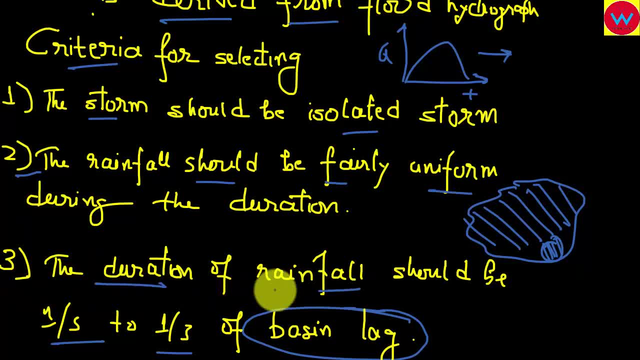 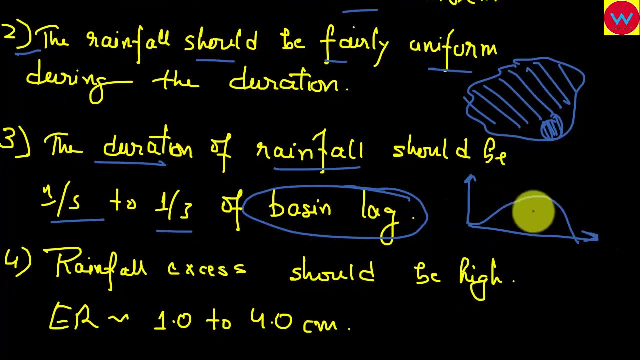 For selecting flood hydrograph To make unit hydrograph Is that the duration of rainfall Should be around One fifth to one third of basin lag. Now, what is basin lag? Basin lag is this thing. Suppose This is our hydrograph. 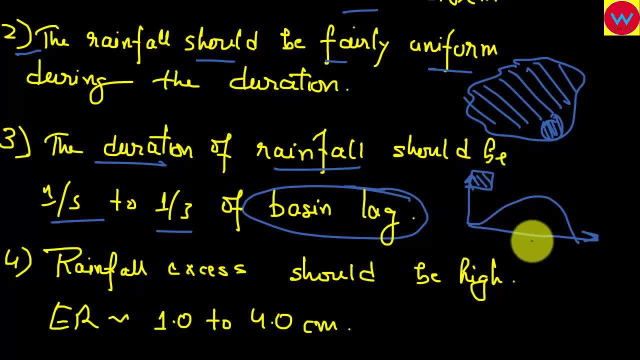 And this is our Rainfall. This is time t, This is q. So let us say that the center of mass Of our hydrograph is this And center of mass of Rainfall, access Is Is given by this line. 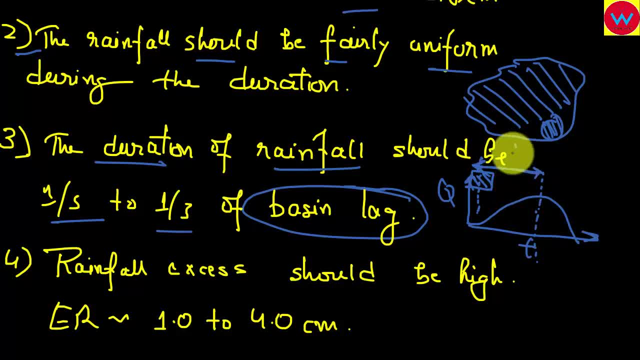 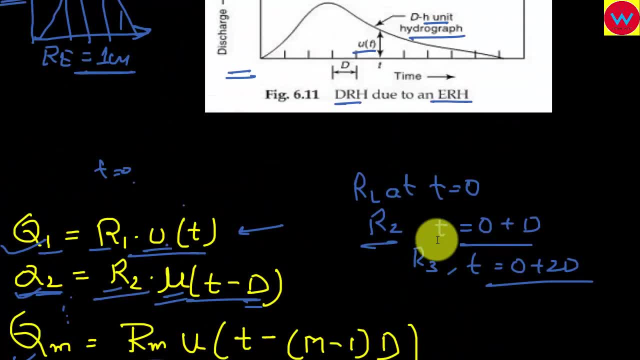 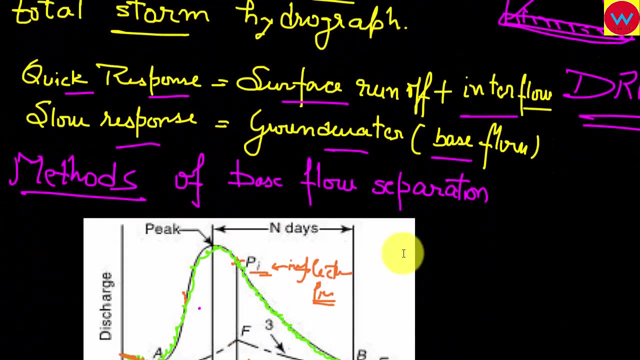 So the distance in time, Or basically the difference in time Between these two lines Is called as basin lag. I have shown you earlier In elements of hydrograph That. If you have noticed correctly That what is basin lag, Let me show it once again. 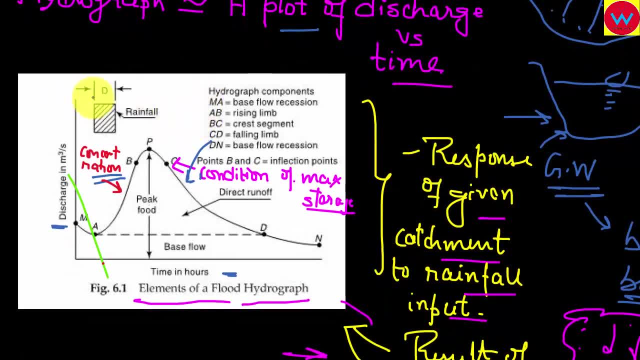 I don't think this. If The center of mass Is like this, And center of mass Of this hydrograph is this, Then this thing is called as basin lag. It's a Just an- Let us say that- Parameter we have. 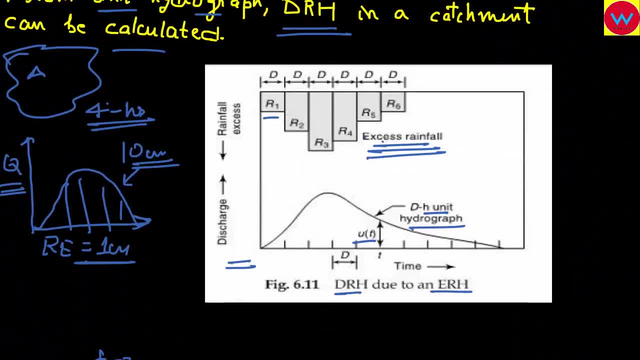 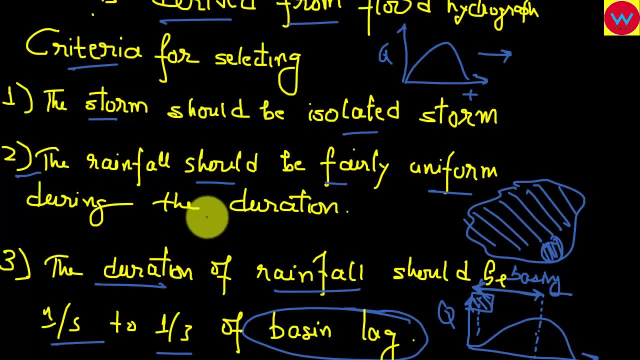 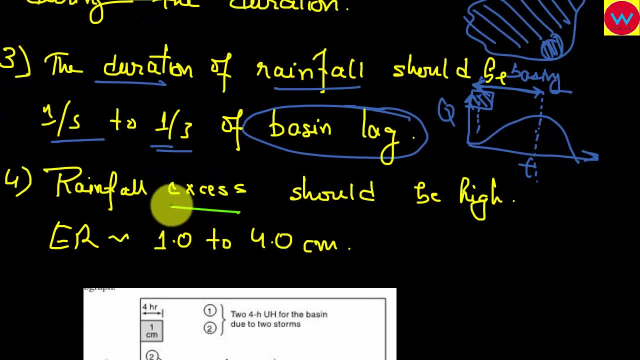 Defined to make our calculations Or other associated Thing quite easy. So one of the criteria for selecting Flood hydrograph is the duration Of rainfall. access Should be one fifth to one third of basin lag And the rainfall access should be high. 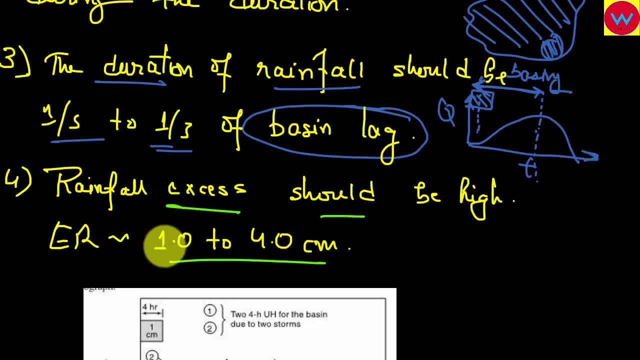 Because we need to Measure discharge values And if rainfall access is low, Then Q will be less And there may be a high degree of Error in measurement of Q And fluctuations may be Greater. So, in order to minimize those things, 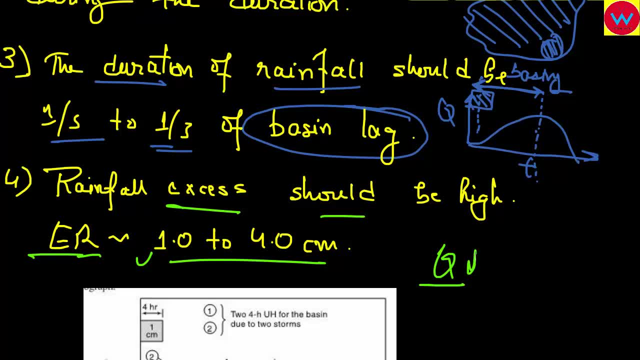 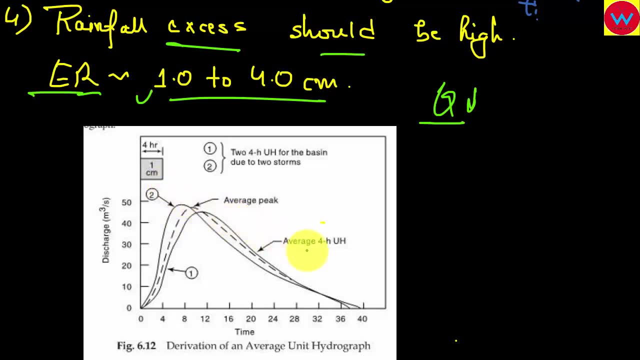 We need to have effective rainfall, So we have This graph. This graph Is an example Which shows that there are Two For our unit hydrograph. That is First: one is this one And second, one is this one. 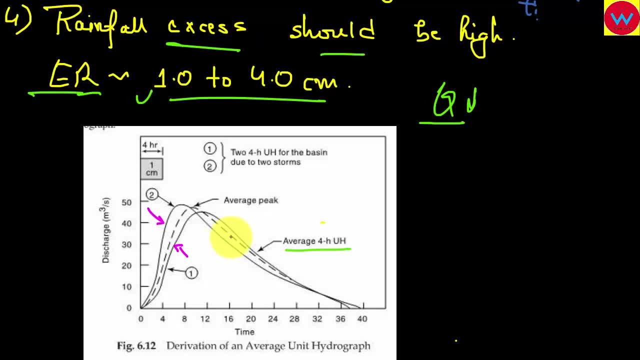 We have derived from flood hydrograph, Because every time We will not be getting similar shape And same parameters And everything will not be same In unit hydrograph derived from Different flood hydrograph, For the same, For our duration. 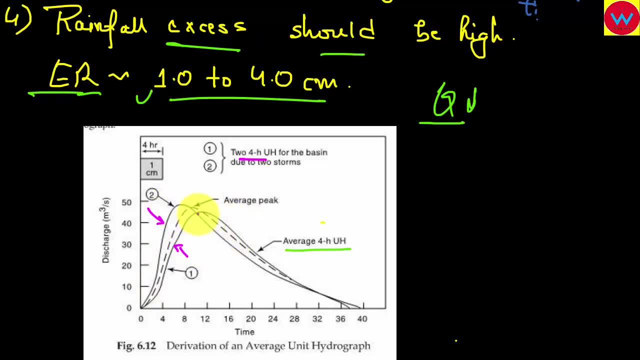 So when we plotted the first one, We got this shape. When we plotted second, We got this shape. Then what we have to do is that We have to take an average Average value of these two graph, And this dotted line is showing the average. 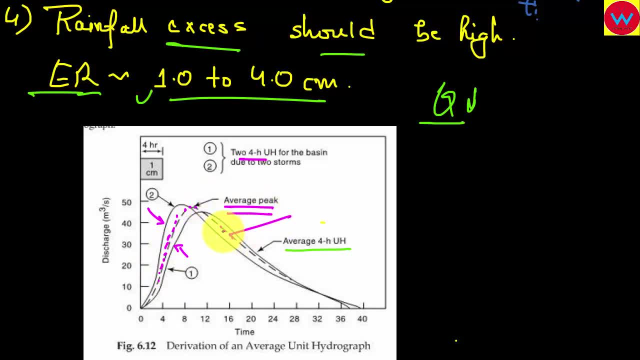 Peak or average value For our unit hydrograph. This dotted line Will be our final For our unit hydrograph, Which we will be use, Which we will use for making Other Direct run of hydrograph For our requirement. 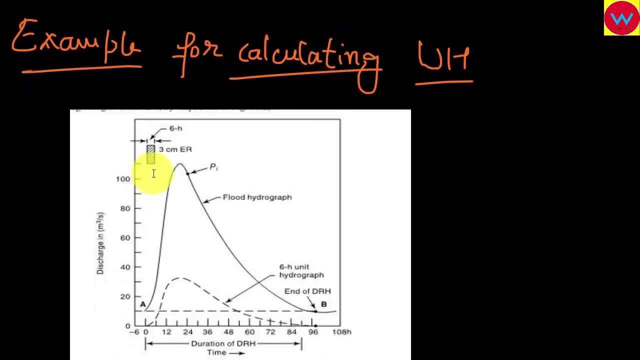 Now Let us look at How we calculate unit hydrograph, Which we will be looking Via a graph Which has been Taken from a book, In case Urumania, And in that book They have used an example, But I will show you. 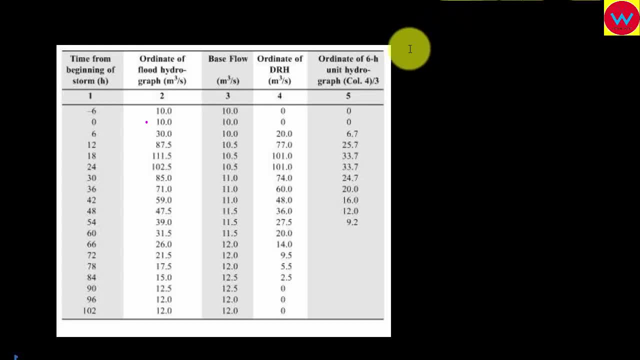 With respect to graph only. Before looking at graph, Let us look at some data From which that Above graph has been derived. I have taken this table from the book only, So what does it say? It says that At time, t is equal to 0.. 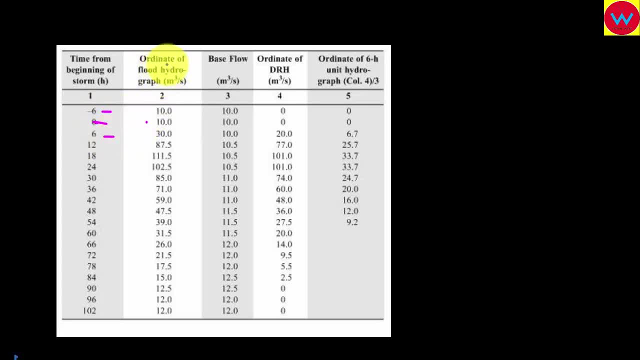 At time t is equal to minus 6. And at time t is equal to 6.. We have ordered An ordinate of flood hydrograph Given by column 2.. In column 1 we have time. In column 2 we have ordinate of flood hydrograph. 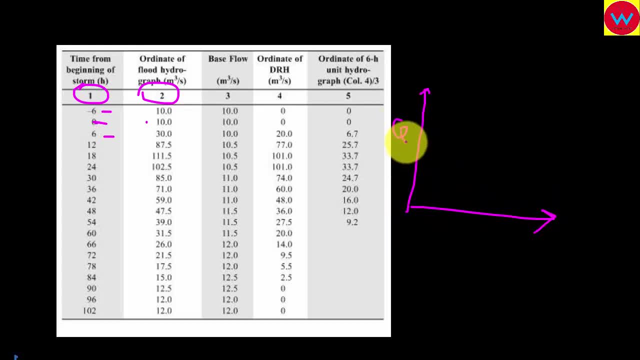 Remember, the flood hydrograph is your, The representation of total value of discharge With respect to time. It is. we have Seen the graph The first time. that was our flood hydrograph. So let us say this is our flood hydrograph. 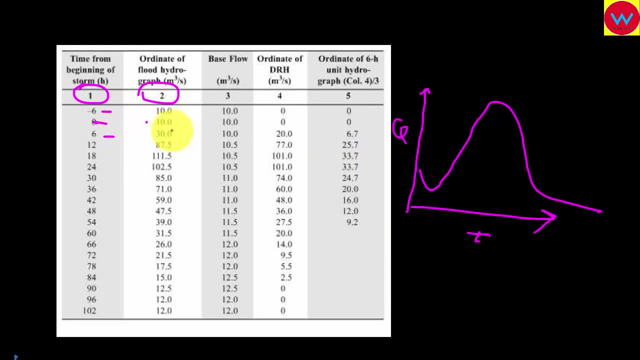 At time t is equal to 0. We have 10 meter cube Of flow in the channel And At different intervals We have total value of discharge in our In our column 2., Which we have obtained from observation. 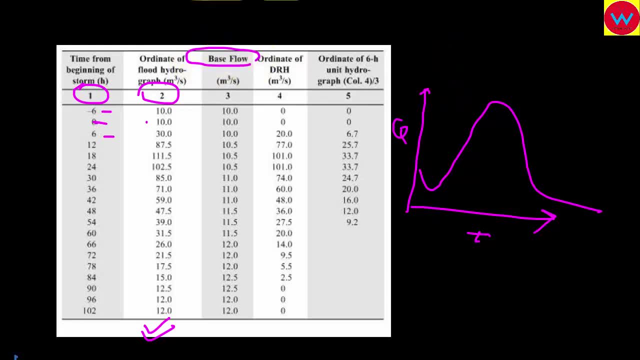 Then first step Is to calculate base flow. That is, let us write those steps. First thing We will do is to calculate. Calculate or Determine, Or whatever term you would like to use. Calculate Base flow Now In order to calculate. 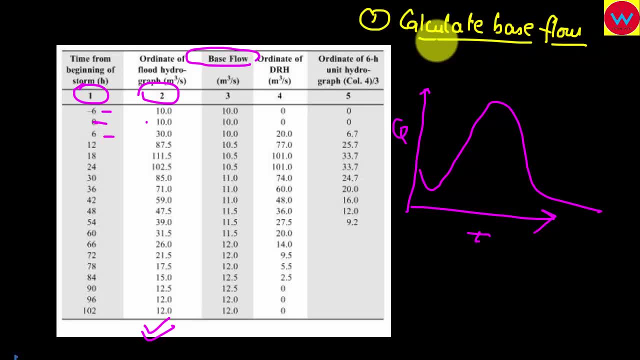 Base flow. You need to go back To our earlier discussion, Where we have discussed 2-3 methods Of calculating base flow And in those method You can obtain Your base flow, Which you will write in column number 3.. 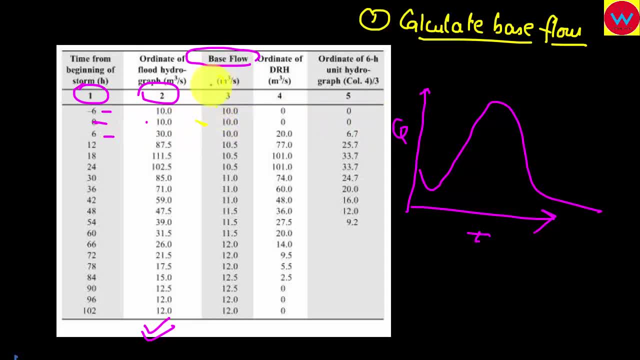 So You have written Base flow here In column number 3.. From your graph, Or from the data available with you. Second step: what you will do Is that you will subtract Base flow from your flood hydrograph To obtain direct run of hydrograph. 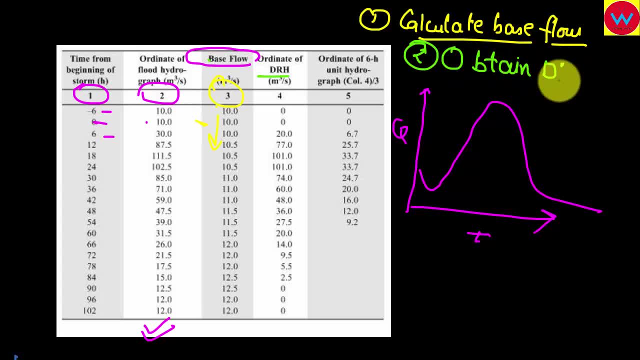 So, After calculating of base flow, Obtain- Obtain DRH, Direct run of hydrograph, Which we have defined as Flood hydrograph, Minus base flow, Called it as direct run of hydrograph. The concept behind This is very simple, that 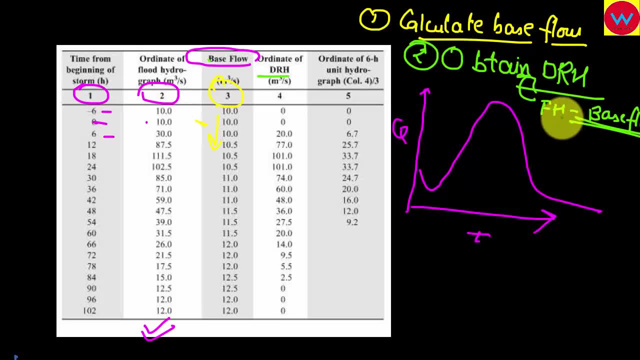 DRH is the effect of only Run of values at that time. It is no. We are subtracting base flow In order to minimize the value, Minimize the effect from ground water Or any other sources. We want to know the. 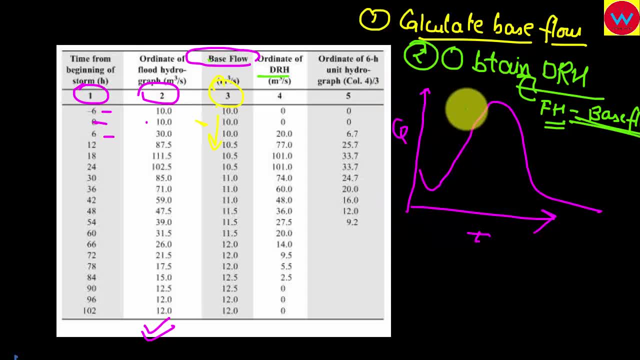 How catchment will react when Only run of values are there. Therefore, we have to. We have to separate base flow. This is our base flow. We have separated it. Then this above figure Will be our DRH. Now we have obtained. 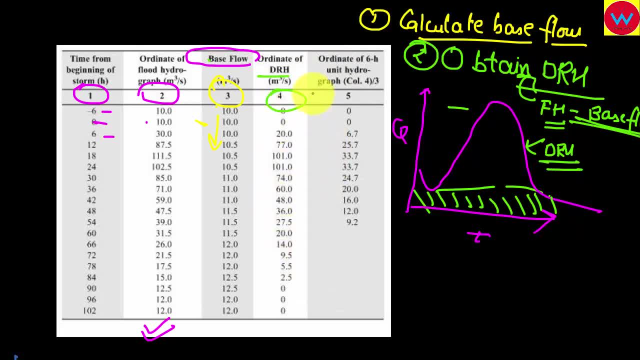 Our direct run of hydrograph. This data in column number 4.. Now the last step Is very simple. You do is that You know your effective Rainfall or rainfall access. You hide your Rainfall access. Let us say: 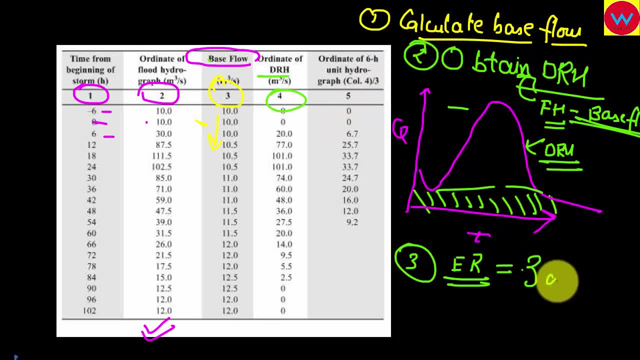 Your Rainfall access is 3 cm. So what you will do Is that You will divide the Ordinate of DRH by 3. Every ordinate of DRH by 3 cm. So Here let us say: 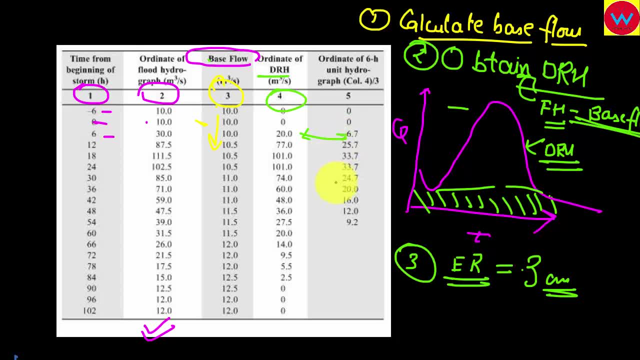 You can see that 20 has been divided by 3. To obtain 6.7.. 77 divided by 3. To obtain 25.7.. So this value Are obtained by dividing DRH by Effective rainfall. 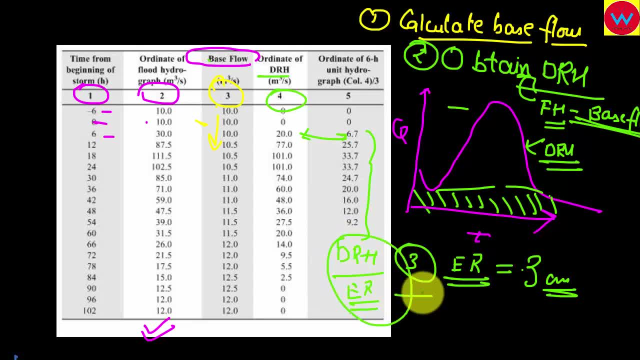 Values. We are dividing it Because we want to calculate. We want to calculate flood Hydrograph for Effective rainfall of 1 cm. We know values for 3 cm There by. Therefore, by simple logic, In order to calculate values for 1 cm. 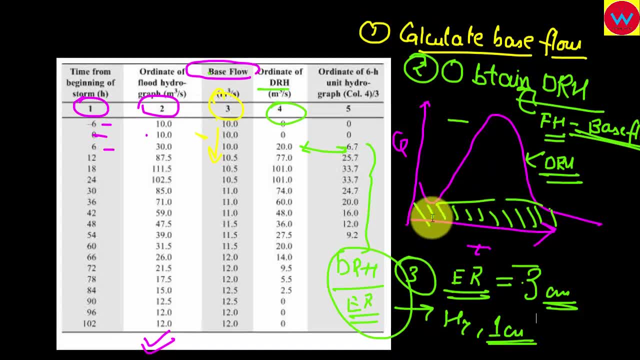 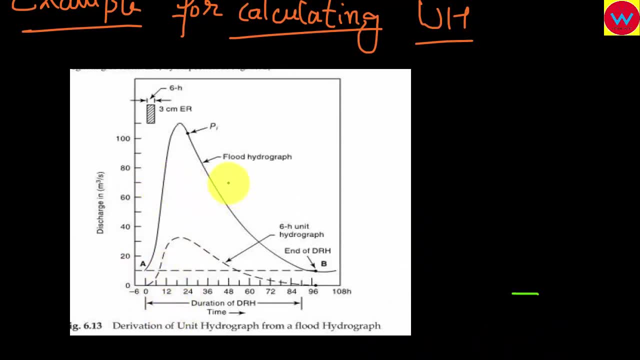 You divide by 3. Ordinates with respect to 1 cm Effective rainfall, And this thing has been represented In graph here. This is your flood Hydrograph. This is, And this is your base flow. You can see this line. 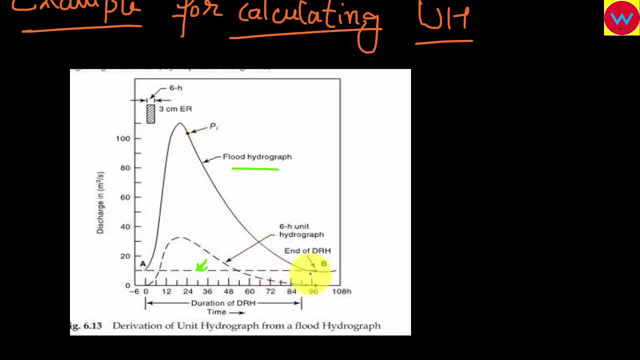 This is your base flow And after, First of all, You separate your base flow, This thing you have to separate, And then, separating your base flow, What you have to do, You have to divide your Every ordinate of this. 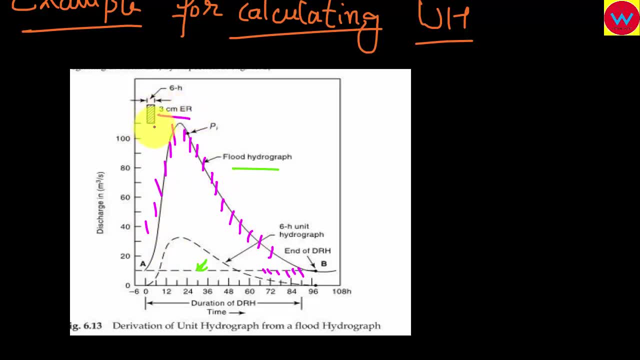 Direct run of hydrograph By 3 cm, Because your effective rainfall is 3 cm. It will be given to you. So It's a quite simple thing To calculate Unit hydrograph From given Flood hydrograph data. 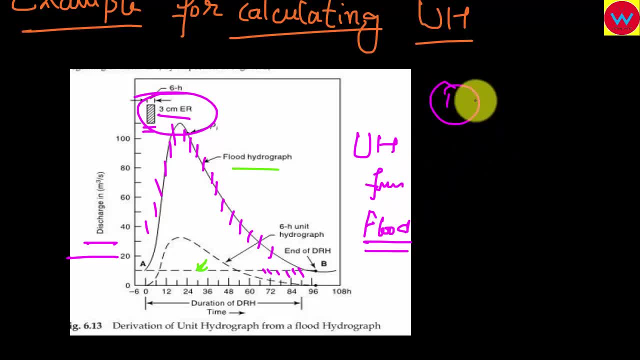 I will repeat you Again. for you, First of all, you calculate your base flow, Base flow. Then subtract base flow From Flood hydrograph, Flood hydrograph Based flow To obtain DRH. Then this thing Will be equal to your DRH. 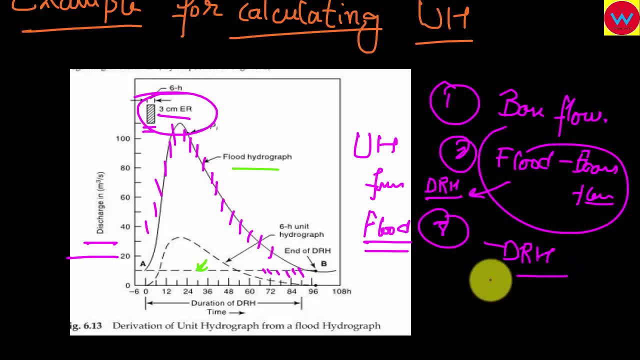 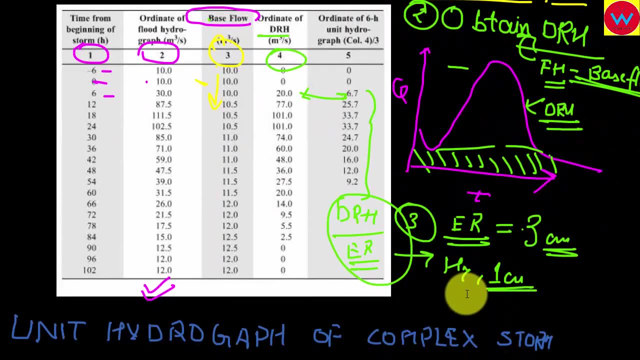 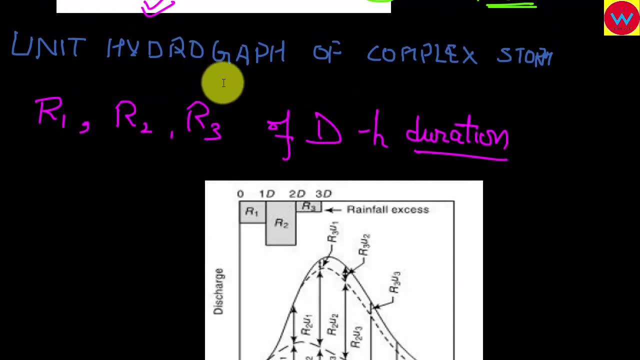 Then divide Your DRH values By 3 cm To get Effective rainfall To obtain Unit hydrograph. Now We look at Unit hydrograph For a complex storm, That is, Storms are taking place In succession. 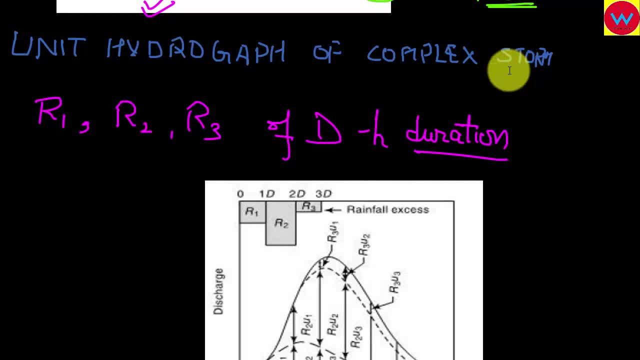 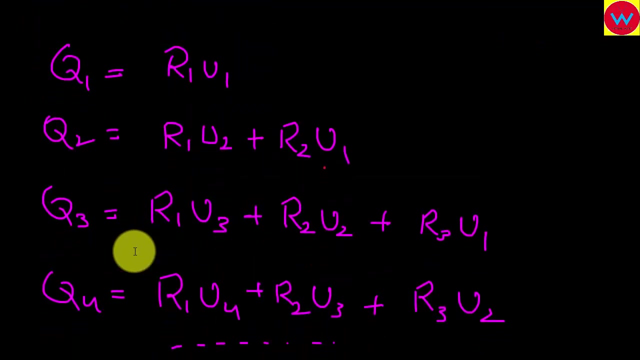 With one another, That is Rainfall. Now In this example You can see That we have R1.. R2., R3.. Three rainfall Access for DRH duration. Then what will be Unit hydrograph for that? 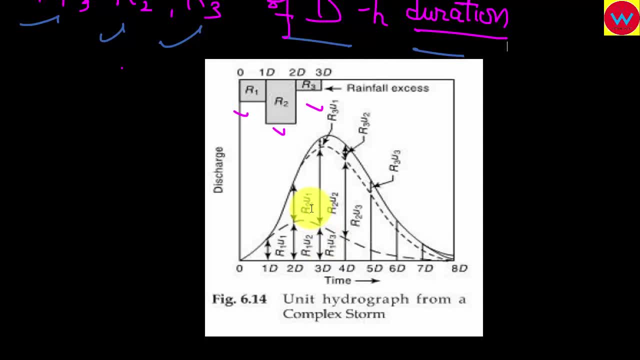 So Unit hydrograph: You can calculate Your unit hydrograph. So let us say, Let's say that U1., U2., U3. Are ordinates of Unit hydrograph Which we want to calculate, And 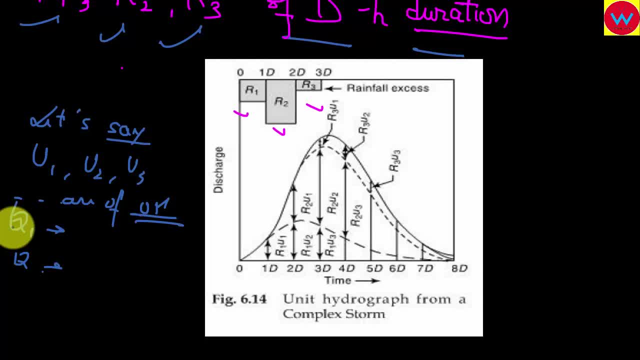 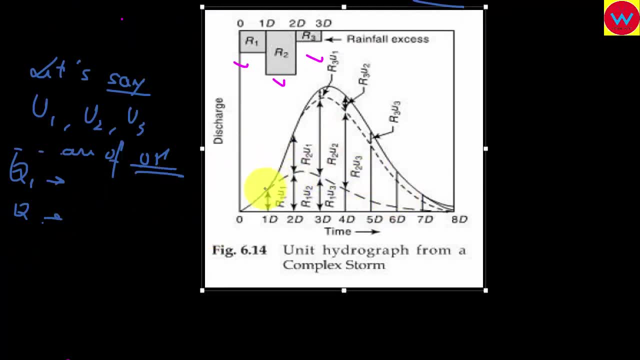 Q1., Q2., Q3., R1., R2., R3.. You can see the Graph here. In this We are having This final graph As flood hydrograph And in between You can see Your unit hydrograph. 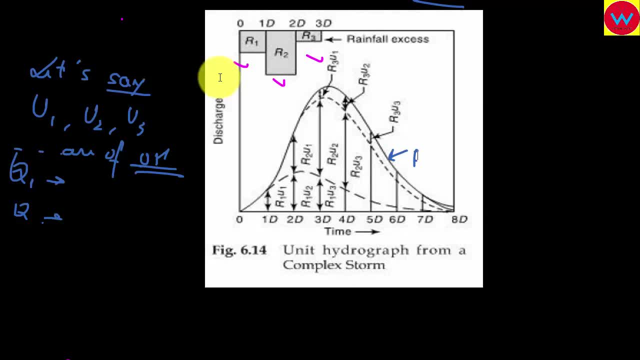 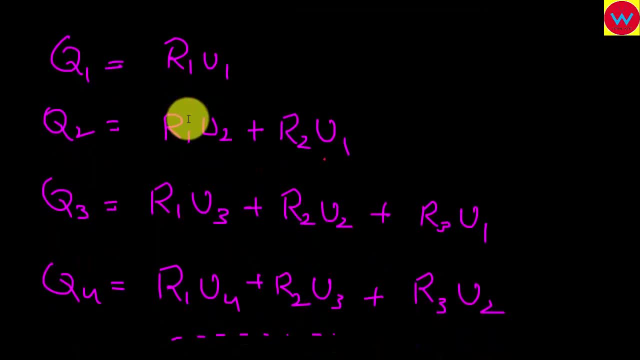 But We do not know Value of Unit hydrograph. So how we do, How do We proceed with this Is like. We know that for discharge Q1.. Q1 is the value of discharge At this place. 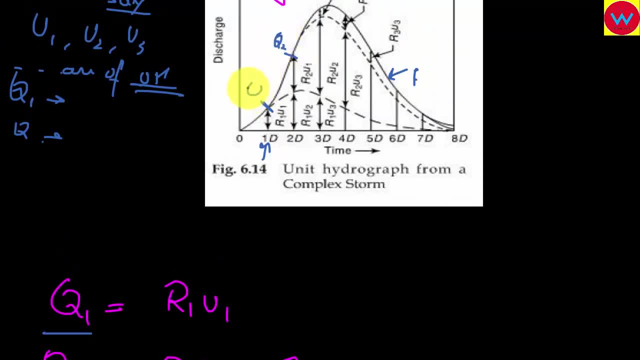 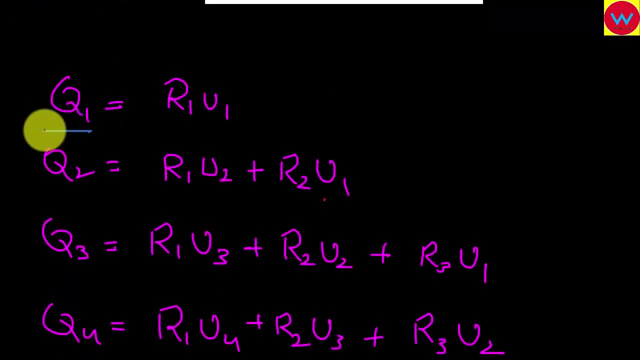 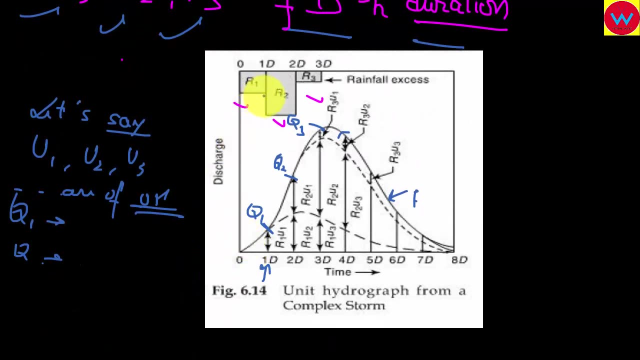 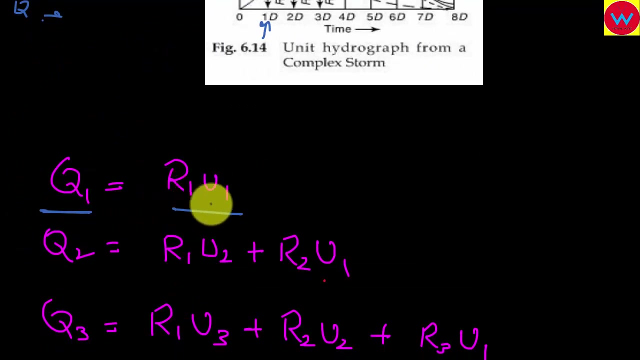 Here, Or you can say At this place: Q2 is the value of discharge Here, In For Q1.. Only R1 will be contributing Because In this duration Only R1 is effective rainfall Which has taken place. 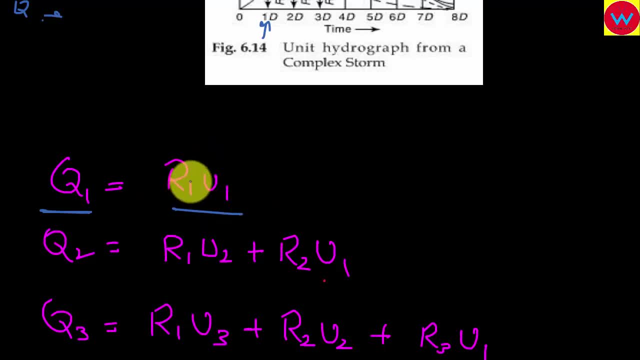 Between 0 to D hour, So We will multiply Unit of Let us, Which we have assumed We will. R2 has started, That is, second rainfall has started, So We will multiply it with R2.. And 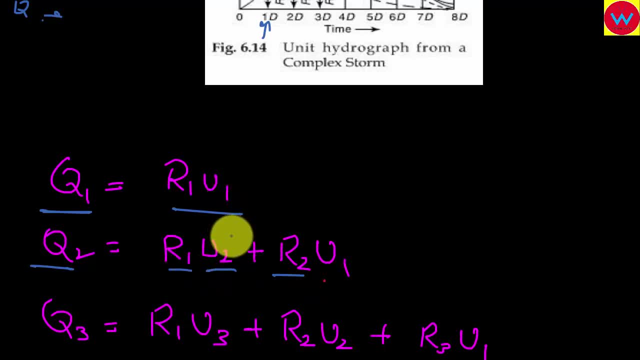 We will multiply the value of R1 with U2.. It is because It is because For Q2 value Our, There will be two Rainfall which will contribute to second discharge. So These two terms, You need to see that. 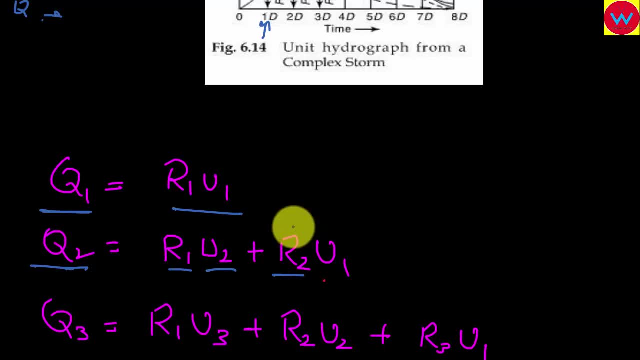 Our Rainfall R2 has just started, So We will. This effect only will be in U1.. We will multiply it with U1.. And for R1 value, The rainfall has Proceeded quite a bit, So We will multiply it with U2.. 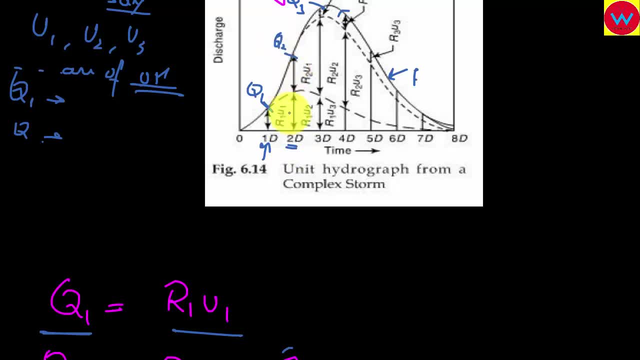 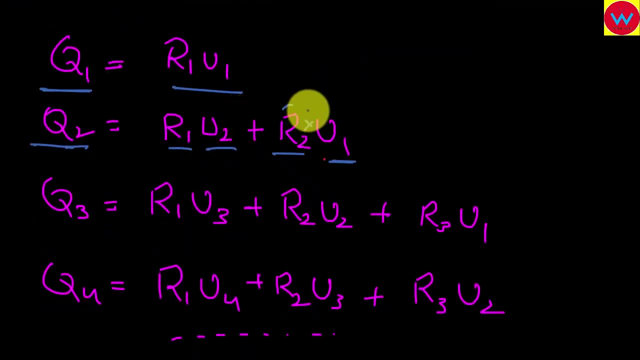 You can see it in graph here. That Is U2.. Here The value of R2. Is multiplied with U1. And value of R1. Is multiplied with U2.. If you are finding it difficult to understand, You can. 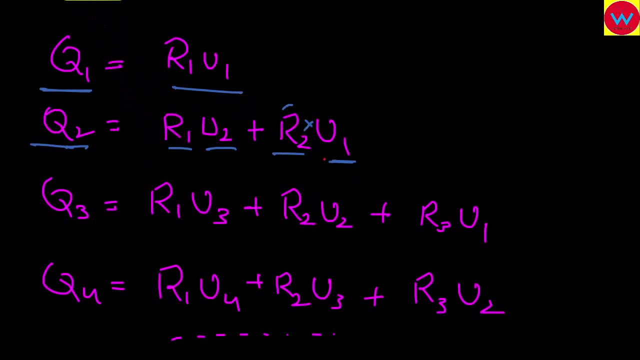 If you are finding it Difficult to understand, Visualize it Like this: Because R1 is the initial rainfall, So it will contribute in all of the discharges. That is one thing. So Here you have R1. Okay. 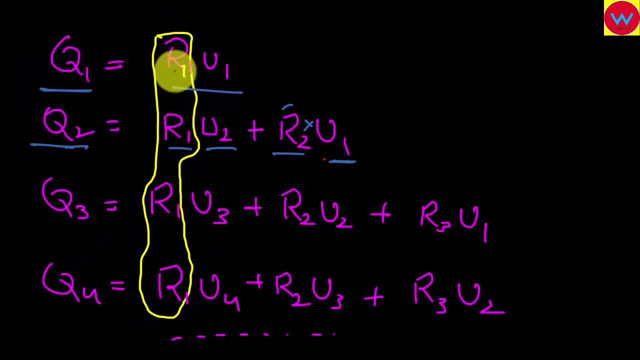 So R1 will contribute In all of Q1, Q2, Q3.. And so What we do? We multiply R1 with U1, U2, U3, U4, U5. Like that, So its contribution is in all. 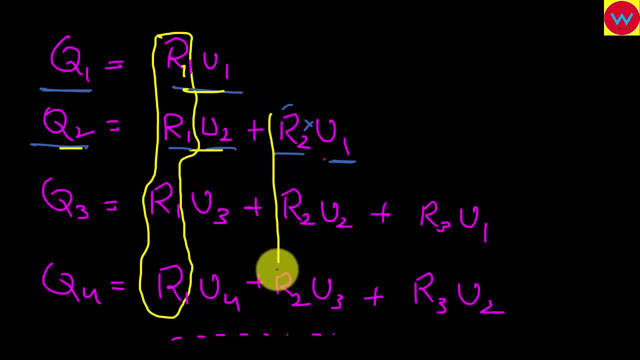 And R2 will start from Q2 discharge, So R2 will contribute From this Q2 in all of the So again, Multiply R2 with U1, U2, U3.. R3 will start from Q3.. 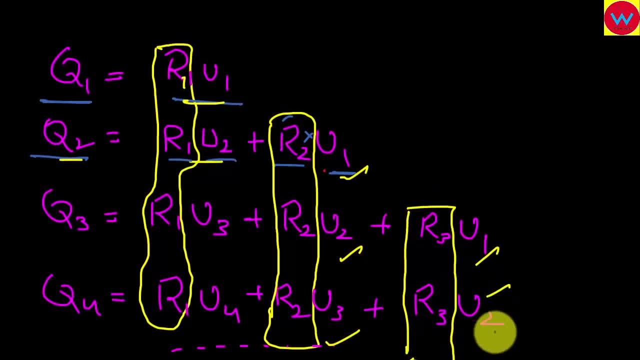 So again, You can Multiply R3 with Q1, U2, U3.. Because you know, In order to calculate flood hydrograph, You have to multiply your, You have to multiply your unit hydrograph With respect to rainfall access. 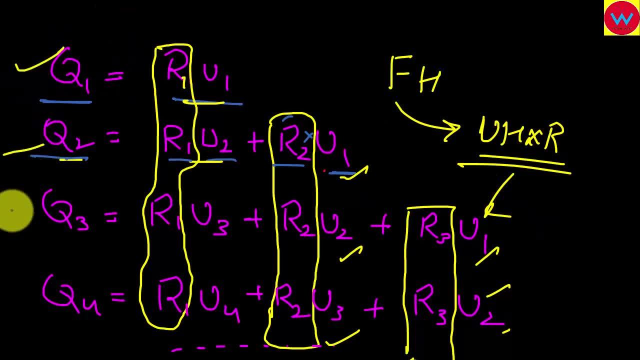 That is the concept which we are using here. So we know this: Q1, Q2, Q3.. We know R1, R2, R3.. So, using all this equation, We will be able to calculate U1, U2, U3, U4. 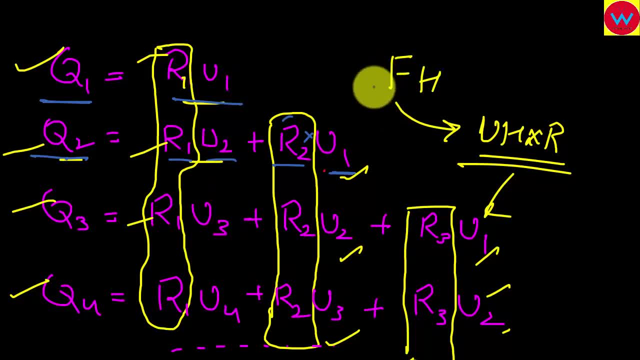 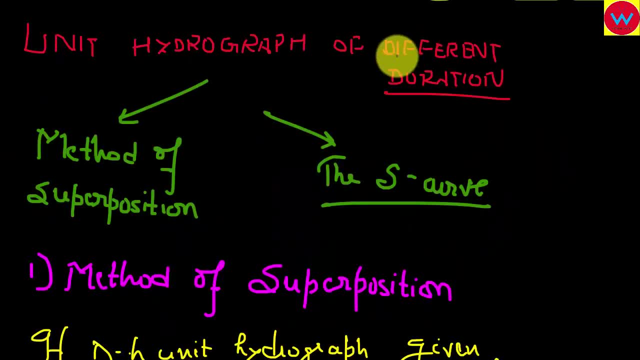 And like that. So we will finally plot our unit hydrograph By doing the Reverse calculations. Now we look at How do we make Or obtain hydrograph, Unit hydrograph for different durations. There are basically two methods. First is method of superposition. 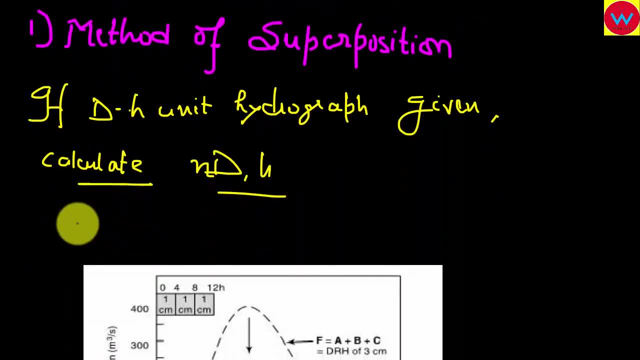 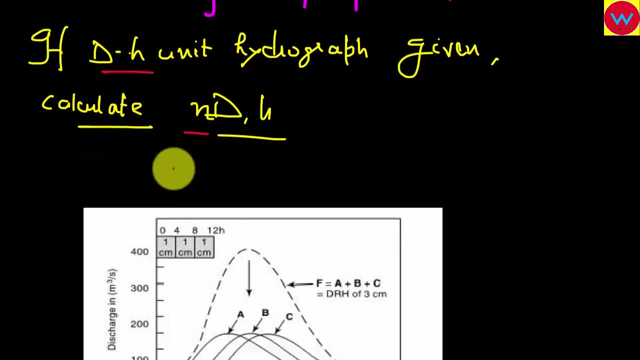 And second is the method of S-curve. So we will look at. In the first method There is method of superposition. What we do is that If D unit hydrograph Is given, Then we calculate N times D our unit hydrograph. 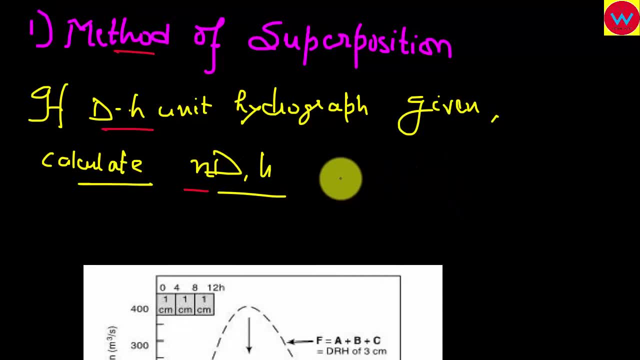 That is, For example, That suppose, If 4 our unit hydrograph is given And You want me to calculate 8 our unit hydrograph, Then It is why We can calculate it, Because 8 is multiple of 4.. 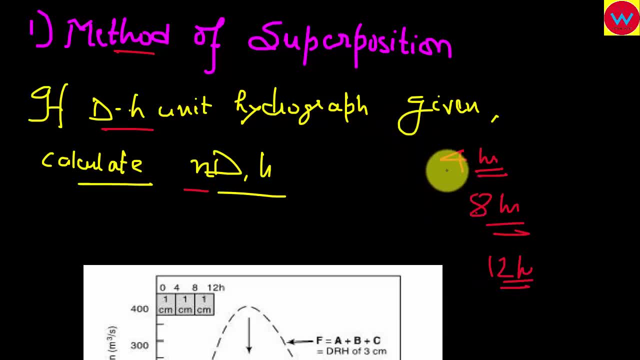 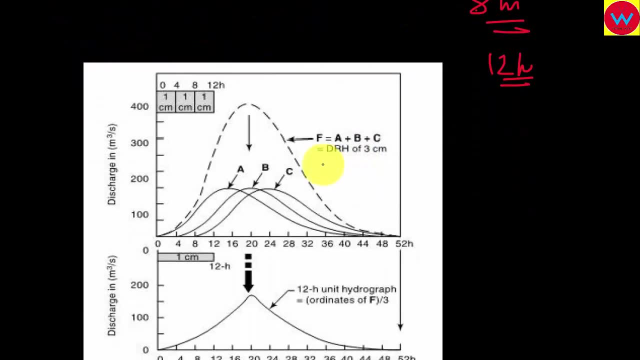 Or I can also calculate 12, our unit hydrograph. So in all the unit hydrographs For D, our duration, Which are in multiple of 4.. Or our given value, We will be able to calculate. So what we do is. 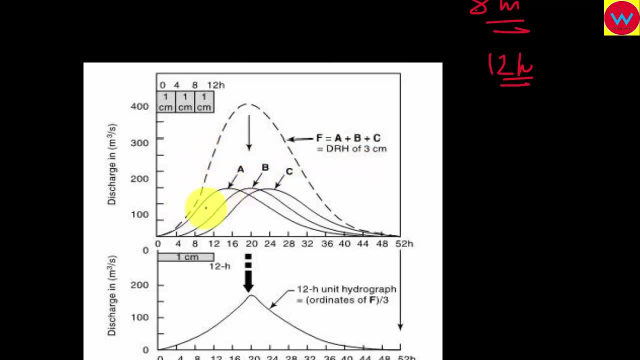 We plot, We plot All the unit hydrograph In our first unit hydrograph Of 4 hour duration And the rainfall excess is 1. As the definition of unit hydrograph says. Then you, What you do, is that: 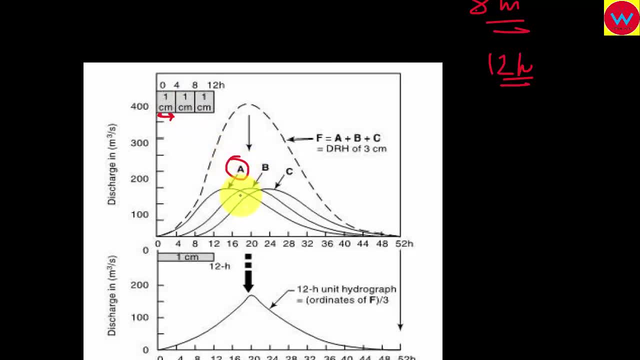 You shift A by 4 cm, That is, you Make another rainfall of 1 cm Excess rainfall. So your This A graph has shifted to From 0 to 4.. So all the parameters will shift Correspondingly for 4 hours. 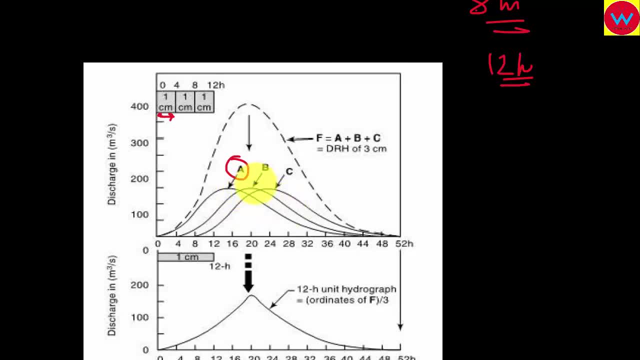 So you obtain another, Another hydrograph. We name it as B. Then again shift B to By 4 hours To obtain C. We are basically shifting. Why we have shifted 3 times Is because we want to know. We want to know. 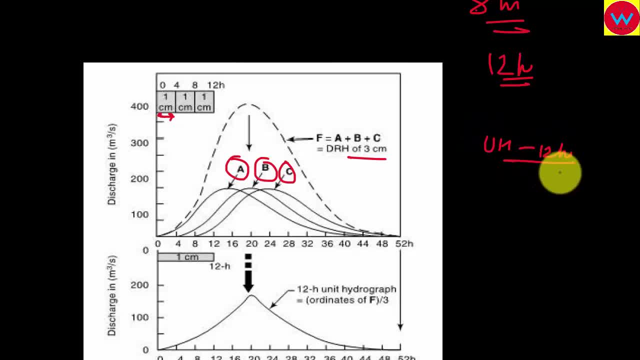 Our unit hydrograph For 12 hour duration, So we have to Shift from 0 to 4.. 0 to 4 is given, So we have to shift from 4 to 8.. Then 8 to 12.. 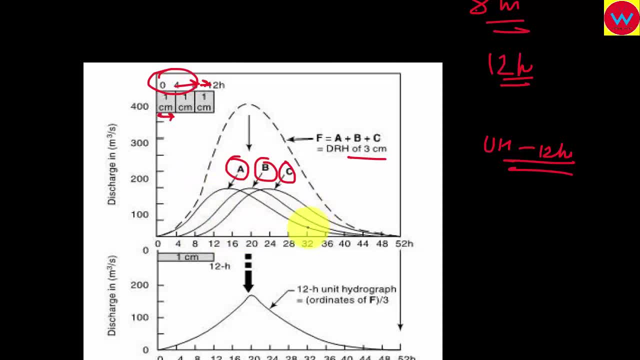 So What we do is that We add all the values of this, All the 3 graphs, to obtain Is this envelope. Envelope is given by dotted line, But what happens? that When we add all the values, We get the value of. 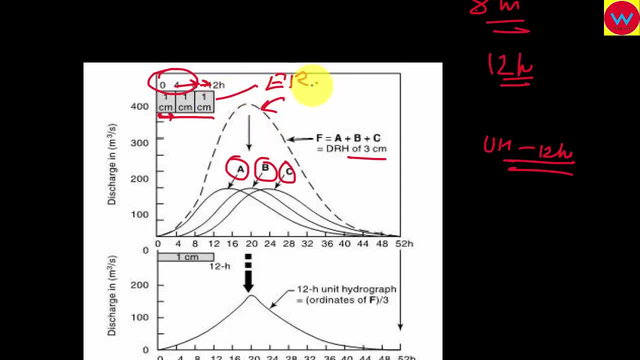 Hydrograph for Effective rainfall of 3 hours. Here ER becomes 3 cm Or DRH. Direct run of hydrograph Is obtained of 3 cm This envelope hydrograph. So we cannot say that By adding all the 3.. 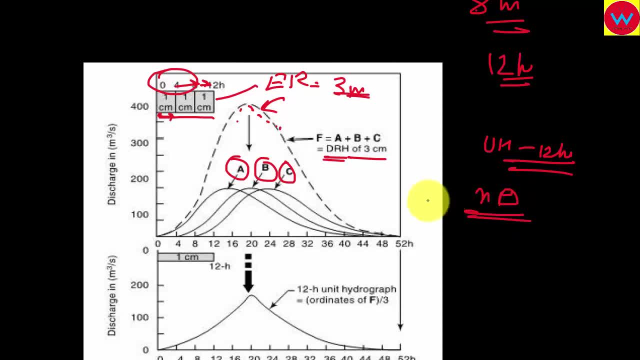 De our unit hydrograph. We obtain And de our unit hydrograph. This will be wrong, Because what will happen? that 1 cm value will be added And we will get 3 cm value. So What we will do is that. 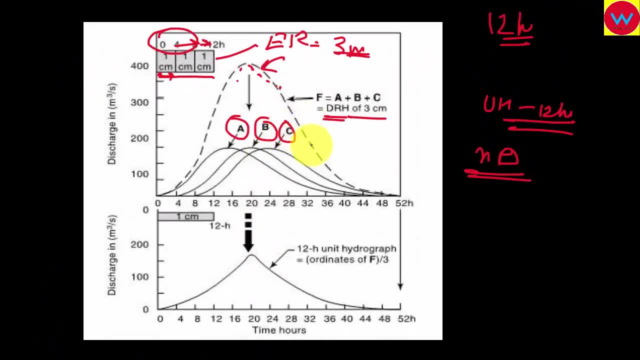 Simply, we will divide the value of This dotted line, Dotted hydrograph By 3 cm, Because the rainfall excess is 3 cm. So we will get finally This hydrograph, Which is our 12 hour unit hydrograph. 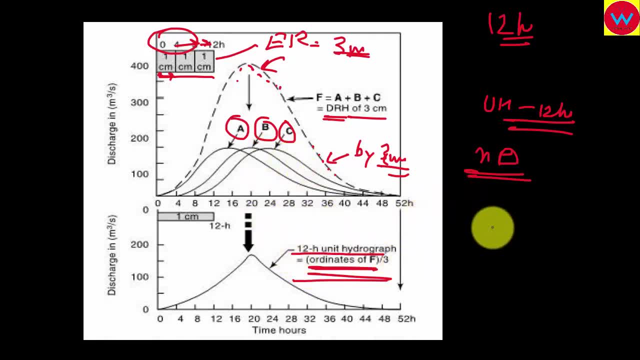 Which has been Obtained from 4 hour unit hydrograph. So what we have done Is that we have obtained 12 hour unit Hydrograph From 4 hour unit Hydrograph. We have been able to do this. 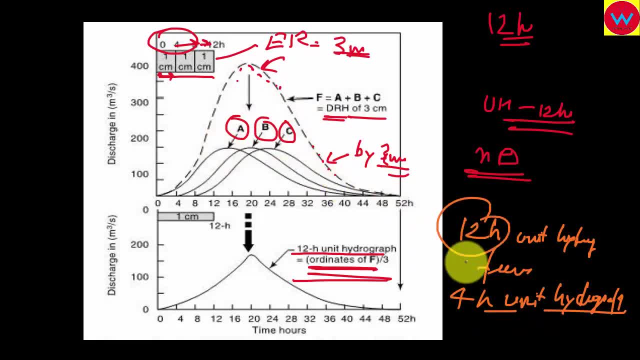 By, simply by superposition, Because 12 is multiple Of 4.. It is 3 times the multiple of 4.. So we have to Shift this 3 times, That is, from 0 to 4 to 8.. 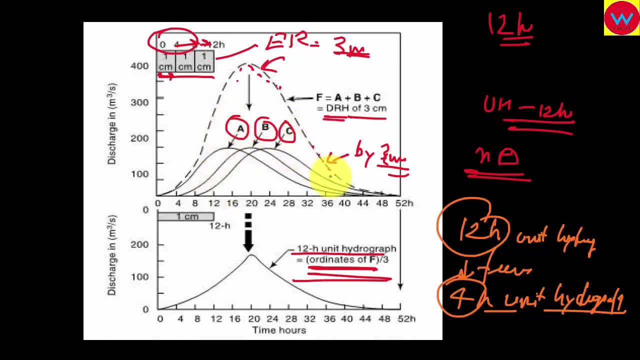 And then we Have summed all the values And then we have divided it by 3.. So you need to be clear Why we have divided by 3. Because when we sum all the 3 unit hydrograph, We obtain the. 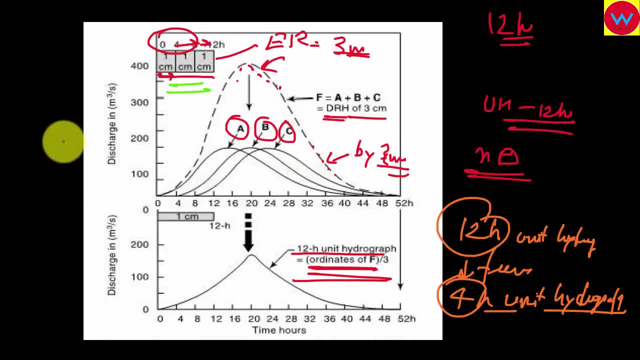 3 cm of effective rainfall. So in order to obtain unit hydrograph- That is, for ER is equal to 1 cm- We need to divide the DRH In order to obtain unit hydrograph. So this is our final. 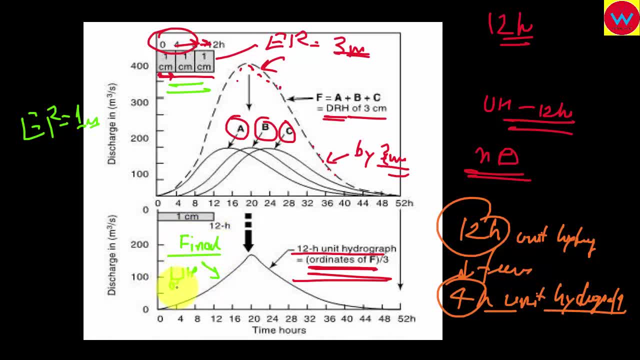 Final Unit hydrograph of 12 hour duration Obtained from 4 hour Unit hydrograph. I think it is quite clear enough And very simple to do Next thing. We will look at second Method, that is, S curve method. 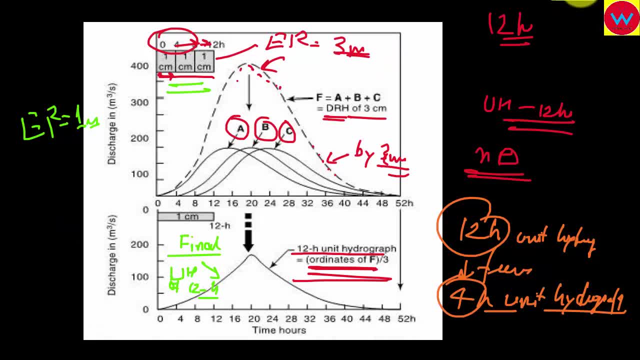 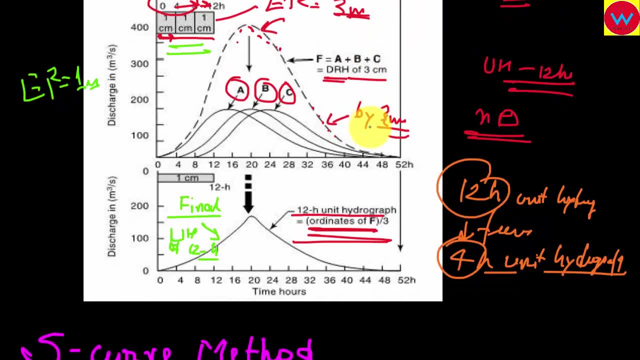 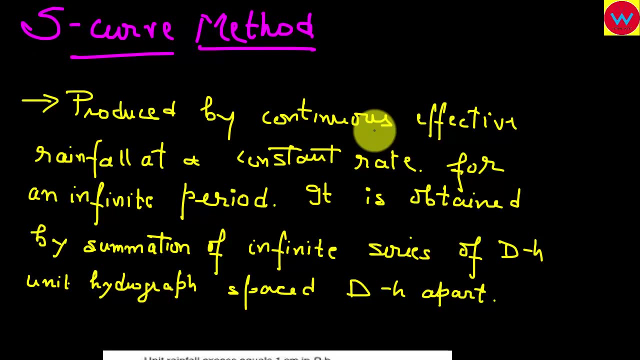 It is quite tricky, Or Quite Difficult, in the sense that Things are not as simple As we have seen here. So let us see S curve method. S curve method Is produced by continuous Effective rainfall At a constant rate. 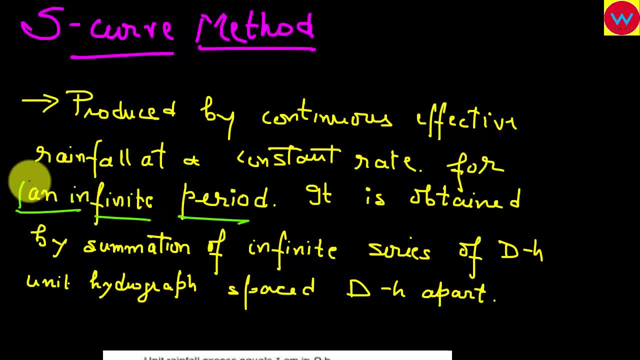 For an infinite period of time. We have to Remember this term, That we are calculating S curve, We are calculating unit hydrograph From an S curve method. Okay, This what we do: that We Assume the rainfall For a constant rate at an infinite period. 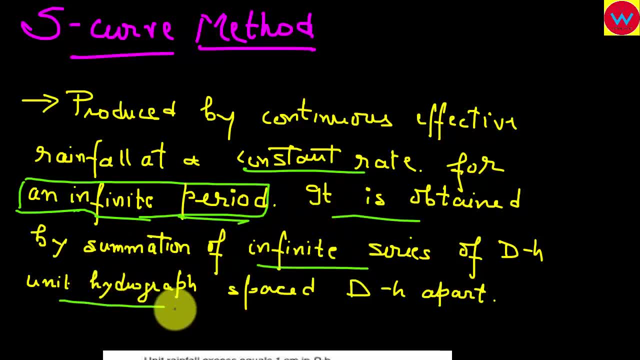 And it is obtained By summation of infinite series of D hour unit hydrograph space, D hour apart. I think you may not have understood It from definition, So let us look At the graph Method of explanation. But once again, what we do is that. 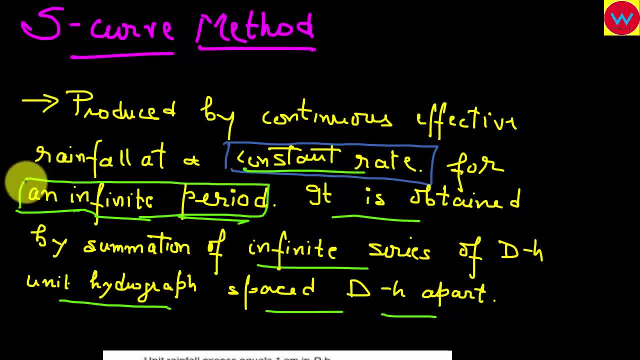 We assume a constant rate And we assume the rainfall To be for an infinite Period of time. So we What we do, is that We obtain it by summation of Series of such D hour hydrograph And which are space D hour. 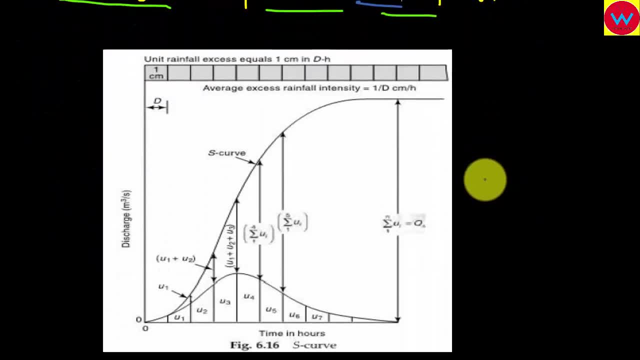 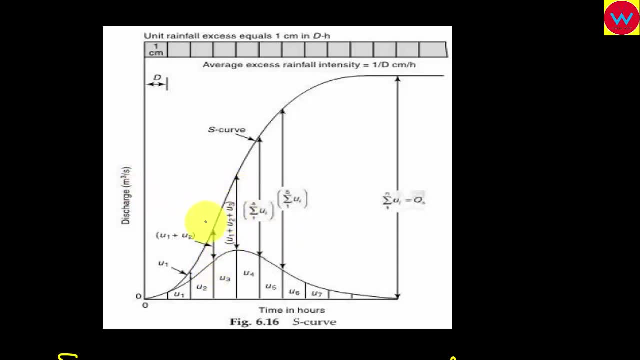 Apart. So This is our S curve method. In this, What happens is that Our Unit hydrograph D hour Are spaced D hour apart. That is, if First hydrograph is at zero, T is equal to zero. 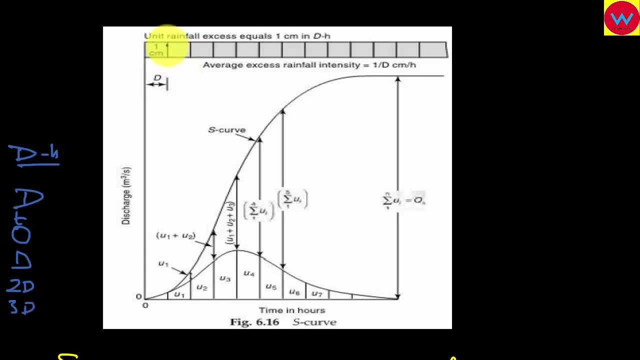 Then second will be D, Third will be 2D, Similarly like 3D. Here you can see your hydrographs, This, So this is a infinite series And all the All the rainfall Excess is equal to one centimeter. 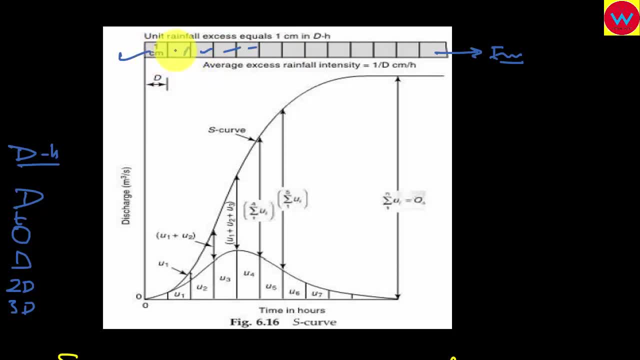 Here Your first Rainfall Excess of one centimeter. Second, Third, Fourth, Fifth, Sixth, Seventh, Eighth, Ninth, Similarly like this. So What happens is that This is our S curve. It has a. 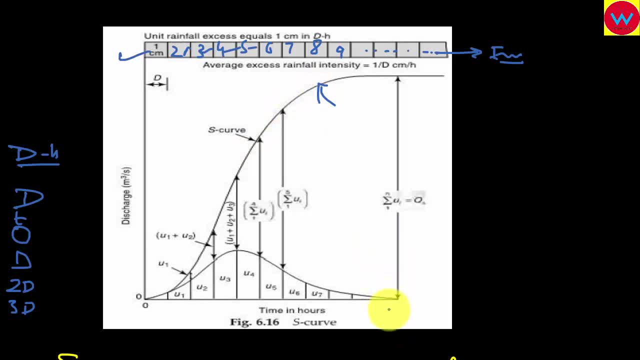 Steep initial slope. Then after some time, That is, after your Base duration of One unit hydrograph, It will have a constant value, That is, This is your S curve. From the S curve We will be calculating Our unit hydrograph of desired duration. 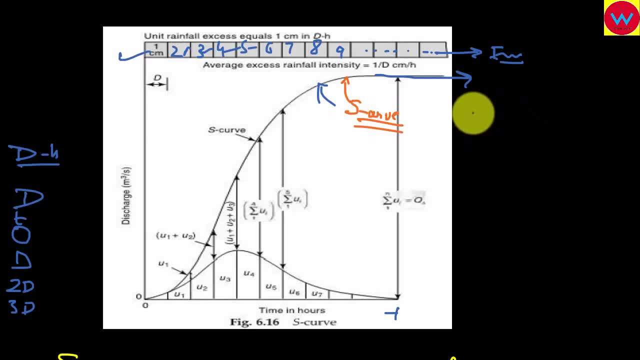 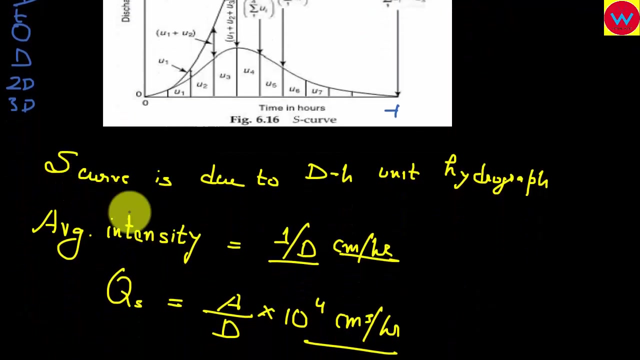 So, First of all, Do like this: You- This is your first hydrograph- Second, Third, Fourth, Fifth, Sixth. So If you sum all this, What you will get, This, This curve, This Which we have shown here. 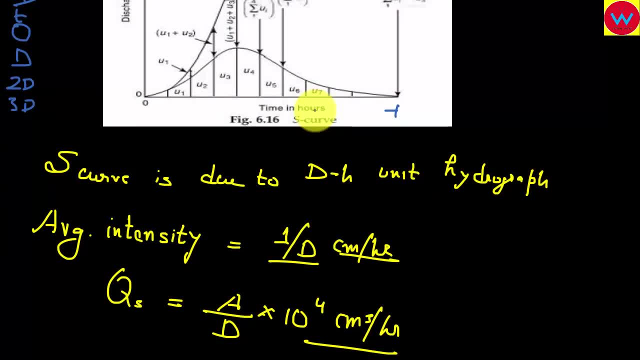 This is our unit hydrograph. We have seen How do we obtain it. Now. Average intensity Will be Equal to one By the centimeter per hour. It is because We have rainfall. access Of one centimeter And duration is D. 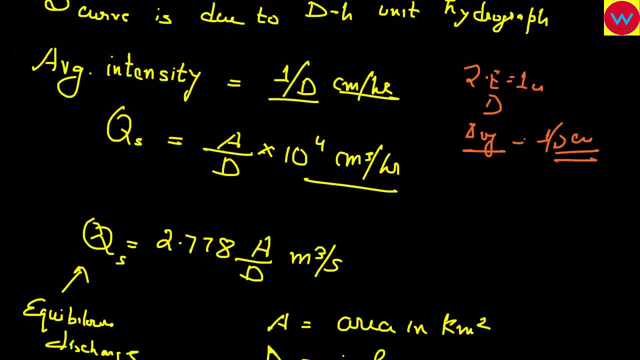 Therefore average intensity, As we have seen, Discharge value At equilibrium condition Will be given by A, by D, into Your area. Basically its discharge Is equal to Area into Into Intensity. So After calculating it, 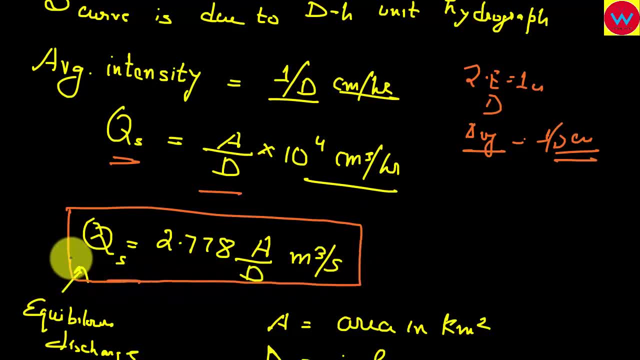 In appropriate terms, We get the value of Qs. That is equilibrium discharge: 2.778 A by D, Where A is area in kilometer square And D is in hour. So what is Qs? This value is your Qs. 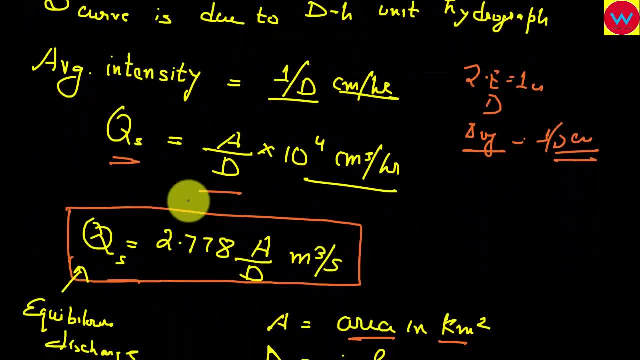 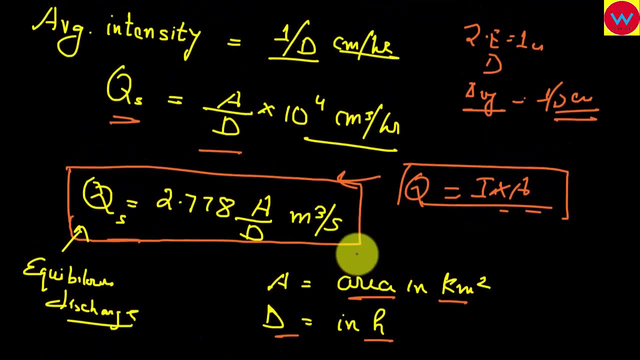 This equilibrium discharge. This value is your Qs, Which we have calculated it like this, And You should know that discharge is calculated By intensity into Area for the given values. We have used it in this Formula. So If we move ahead, 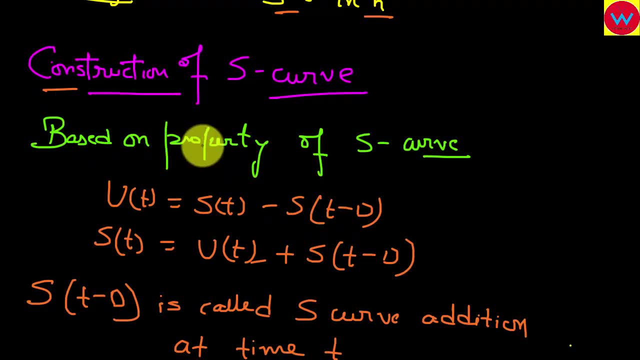 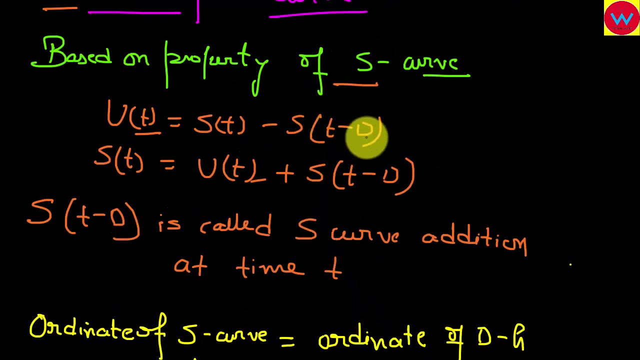 We see that How the We have seen that S curve is. We have made S curve And, based on the property of S curve, We know that, Based on the property of S curve, We have derived one important thing. So first of all, look at this thing. 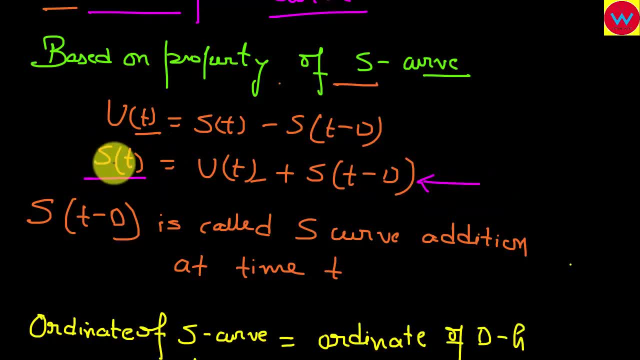 This equation. This equation says that S curve at any time t Is given by unit hydrograph ordinate At that time Plus the previous ordinate of S curve, Just previous ordinate Separated by D hour. So in from this equation. 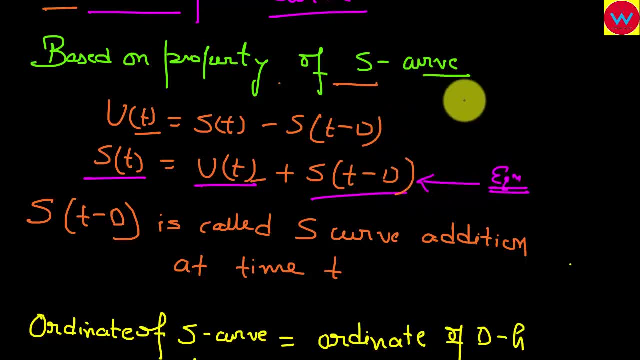 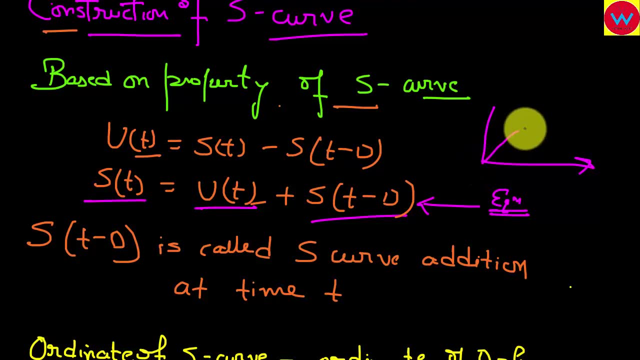 This is quite common To understand or easy to understand. This is why, because What we are doing is that We are summing all the Unit hydrograph Which are spaced D hour apart, So you can visualize this from here. 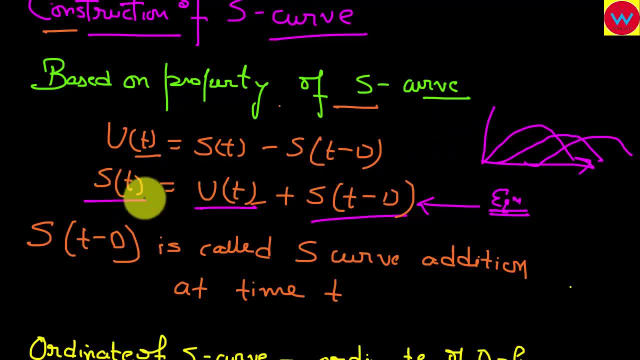 For For given S curve At time t, The, its value will be Equal to summation of unit hydrograph At that time. So if we are calculating, If we are calculating this At here, value at here, So we will have. 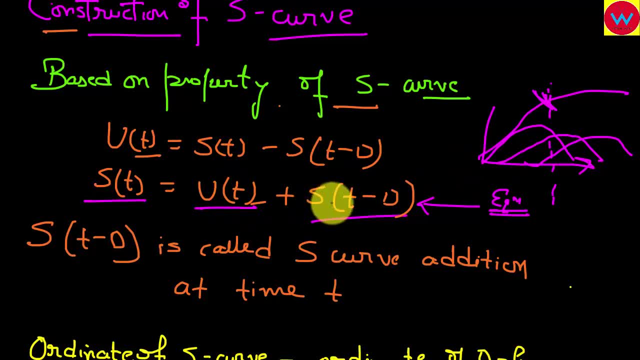 Unit hydrograph For the given time. Ordinate of S curve: One time, one D hour duration. Before that Time: t. From this we will be getting this equation, That is unit hydrograph at time t Is equal to S t minus. 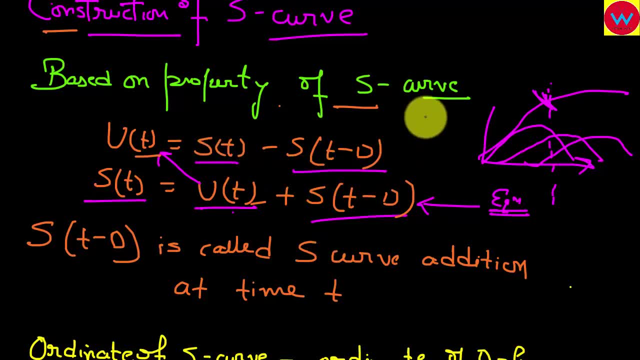 S t minus D. If you are not able to understand This equation, then please draw your Diagram and then from Here there you can easily understand What I am trying to say. I know it may be quite confusing, But its quite. 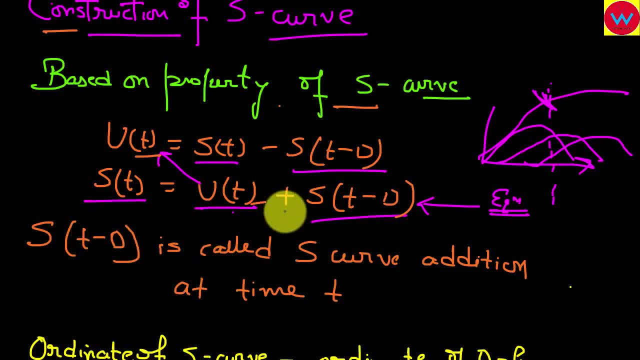 Easy and not difficult, Too much difficult to understand. So what we are doing, that S t minus D, That is ordinate of S hour S curve At t minus D. time Is called as S curve addition of time, t It is. 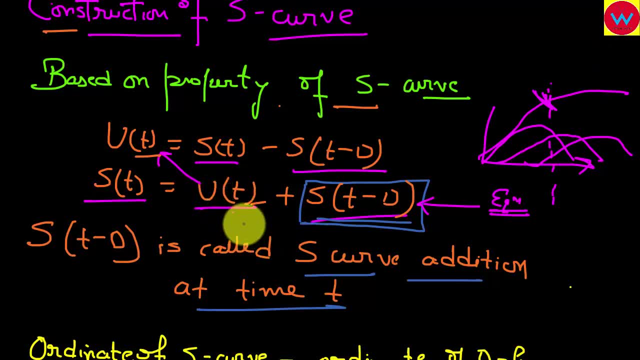 It simply means that If you want to make your, If you want to Obtain your value of S curve at time t, You have to add This S curve addition, This thing S curve addition In your unit hydrograph Ordinate, that is U t. 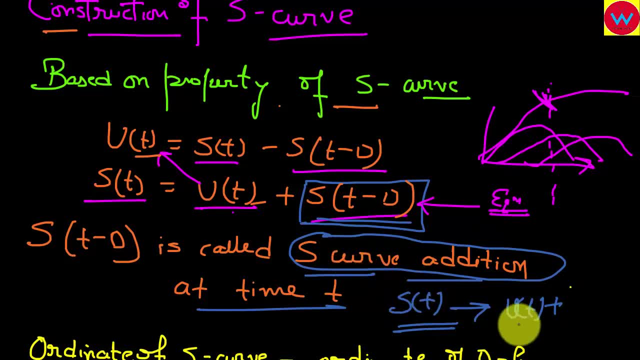 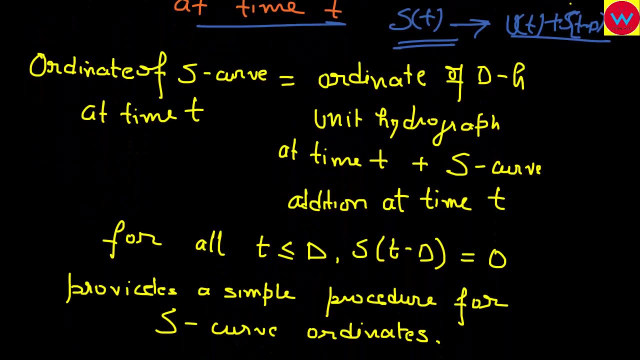 Plus S curve addition Plus the S curve Addition, that is S of t Minus t. Let us look at One concept Ahead. but what I have told you is written here. You can copy it. That is ordinate of S curve. 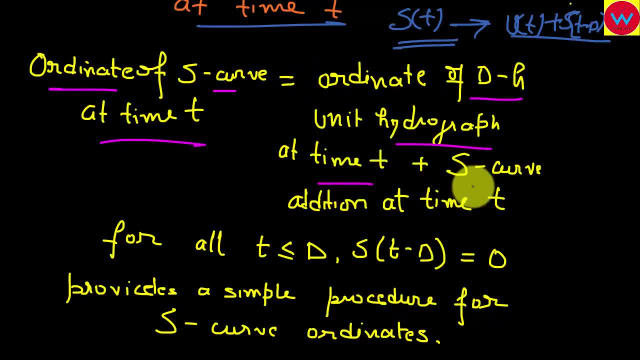 At any time. t Is given by this ordinate of D Hour unit hydrograph Plus S curve addition at time t. So S curve addition at time t Is what Your value of S of t minus t Is your S curve addition of time t. 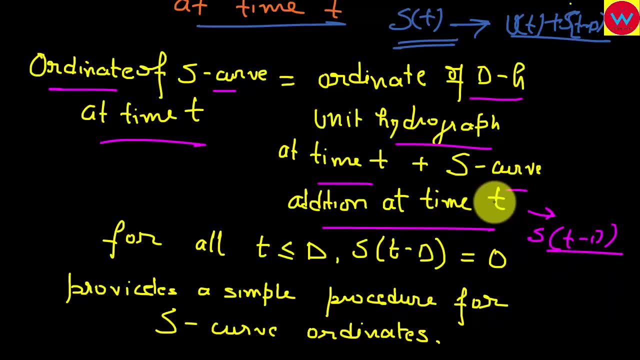 At t. So all the So ordinate of S curve At just previous Value is your S curve addition. So this is important property. You can start from t Is equal to zero And then you can move ahead. So your values will. 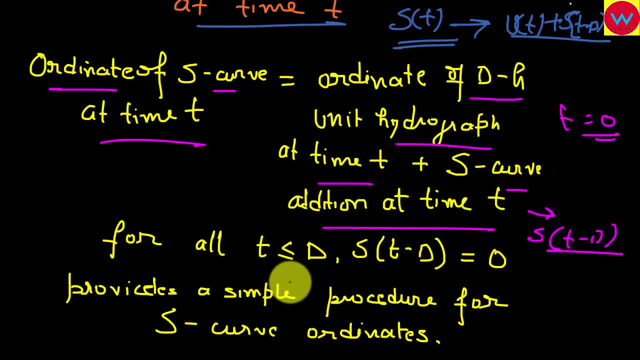 For any S curve will be calculated Because for t Is equal to zero, There will not be any S curve addition, As I have told here. That is for all the values For t Less than d, S of t minus d. 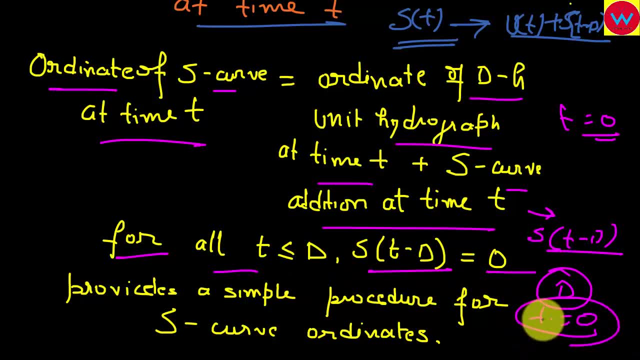 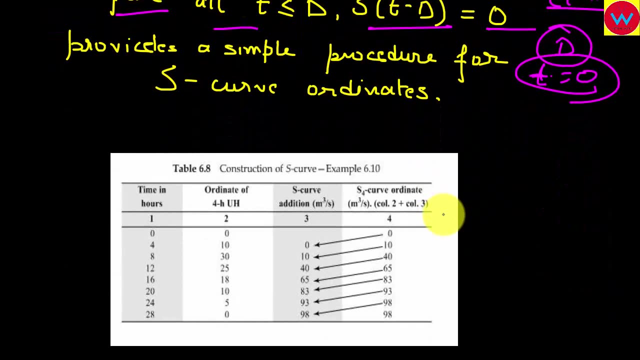 Is zero. So only for t Is equal to d And greater than d, We have S curve addition, And before that Our S curve addition is zero. So I am showing you This table in order to Make it quite understandable. 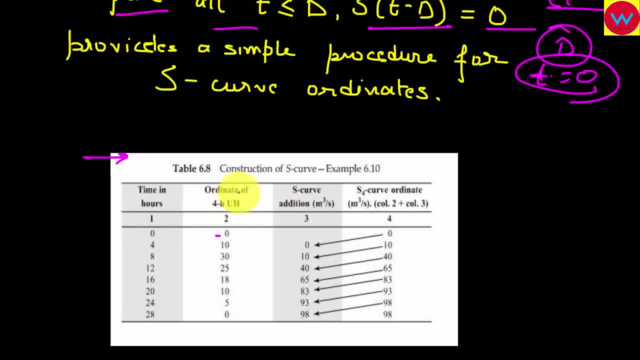 How we can calculate Ordinates of S curve. We have ordinate of 4 hour unit hydrograph, Given in column number 2.. We have time, given in column number 1.. And for We know that We have to space our unit hydrograph, 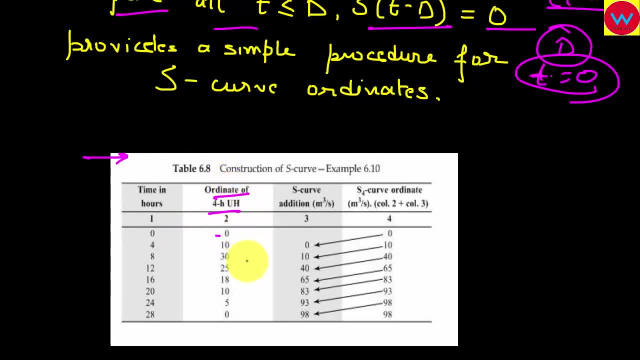 By d hours In order to obtain S curve, And S curve is infinite series of Summation of Infinite series of unit hydrograph Space d hours apart. So you can continue this, But we do not need to continue. 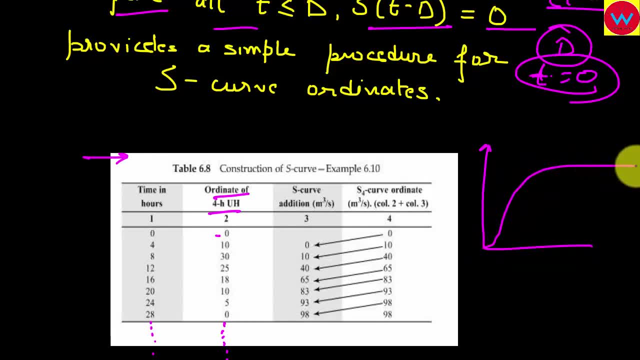 Because we know the shape of unit hydrograph, That after reaching the equilibrium Stage it will not change. So we need to know the ordinate Up to here. only After that we can assume it to be constant. So what we Know, that 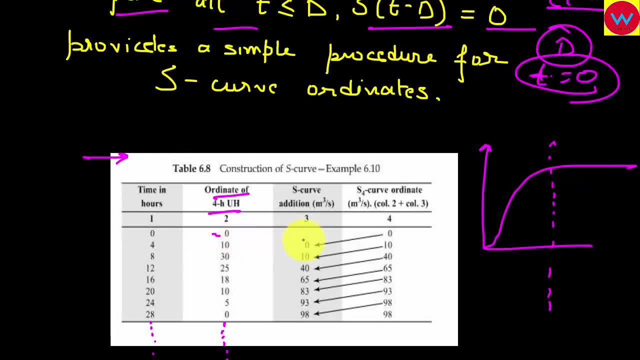 From the property Of S curve addition Is that For t is equal to zero. There will not be Any S curve addition, It will be actually zero. So It is not even valid. So Our S curve ordinate is zero. 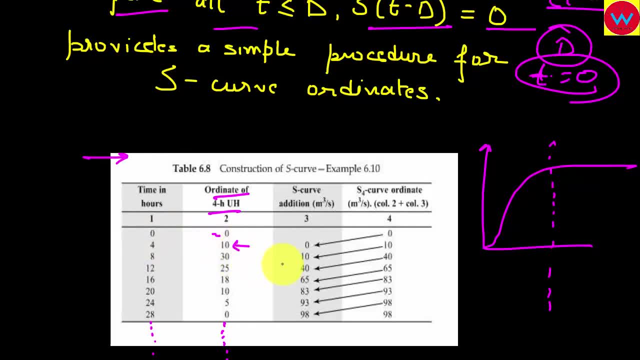 At t is equal to four. Our unit hydrograph ordinate is ten. Okay, So At t is equal to four. Our This, This equation, says that for t, T less than equal to d S curve addition is zero. 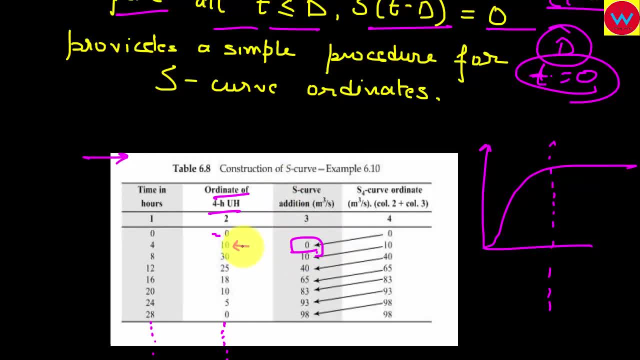 So we have value zero here, And In order to obtain S curve you have to plus. You have to sum The ordinate of unit hydrograph Plus S curve addition, So you will get The value of ten here At t is equal to eight hours. 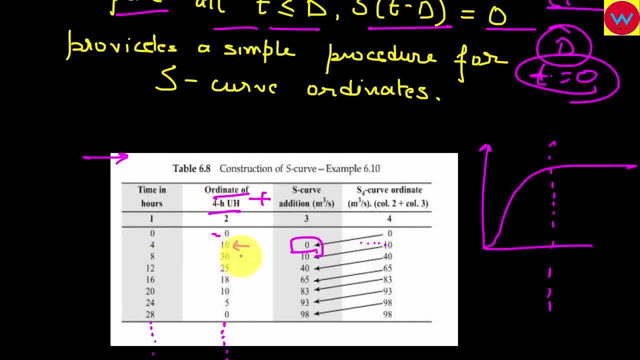 We have ordinate of For our unit hydrograph as thirty And S curve. addition is The value of S ordinate, S curve, ordinate just Before that step, So just before this step, That is, just before Time. t is equal to t eight. 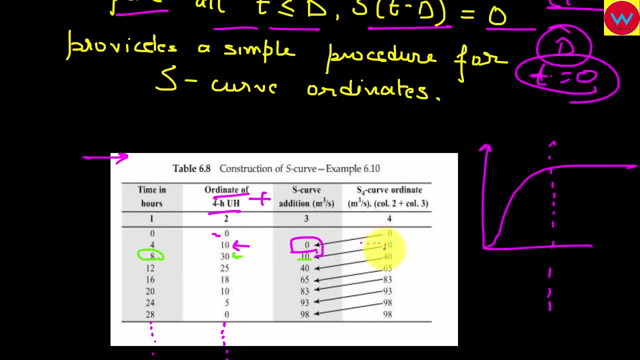 It means that at t is equal to four, We have the value of S. curve is ten. So ten will become S curve addition. for the next step, This is quite simple thing to understand. That is the value of S curve. ordinate becomes the. 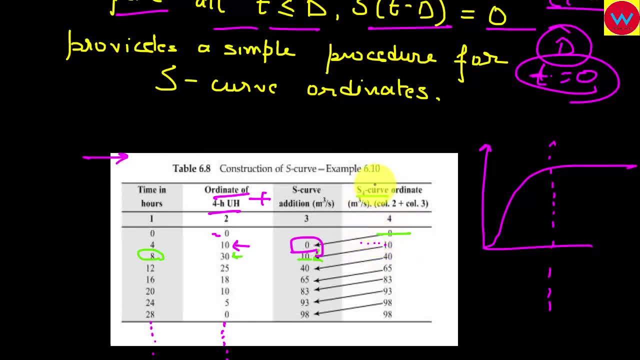 S curve addition for the next step, That is, at t is equal to zero. S curve ordinate is zero, So it zero will become. Addition. S curve addition for next step, That is you. can You have seen the arrow here? 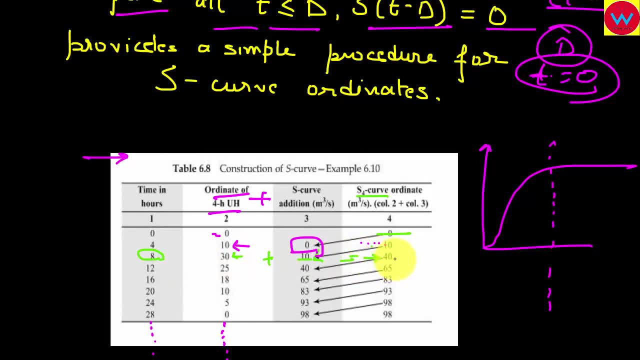 It means the same thing. So the total will be thirty plus ten. It will be equal to forty. here Now this forty will become addition for next step. That is, forty is equal to Twelve. Then it will become sixty five. Then sixty five will become. 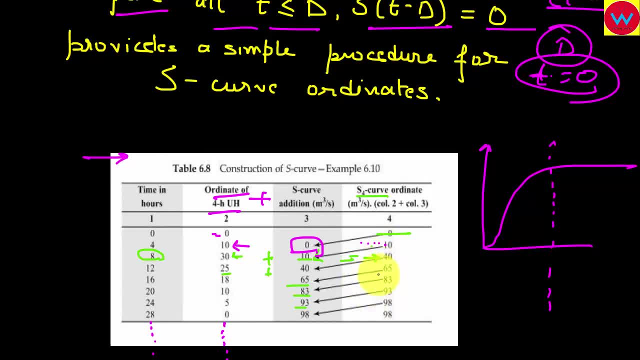 S curve: addition for the next step. Similarly, You get value here. It becomes addition for the next step. Then it is quite simple thing. And we are seeing that We are getting ninety eight. So ninety eight will become our equilibrium discharge. 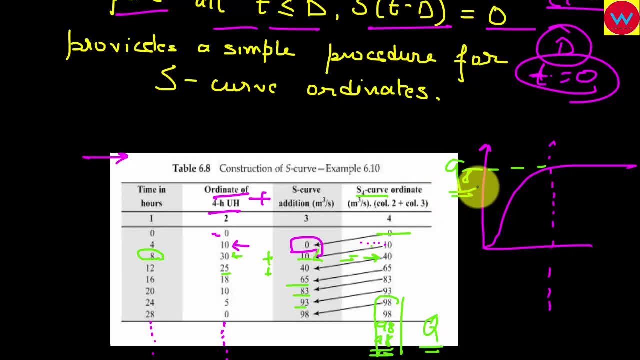 Q. So here It will be your ninety eight. Now we have obtained S curve. Now, from S curve, we will obtain T, our unit hydrograph. What we are doing is that We are obtaining T, our unit hydrograph. 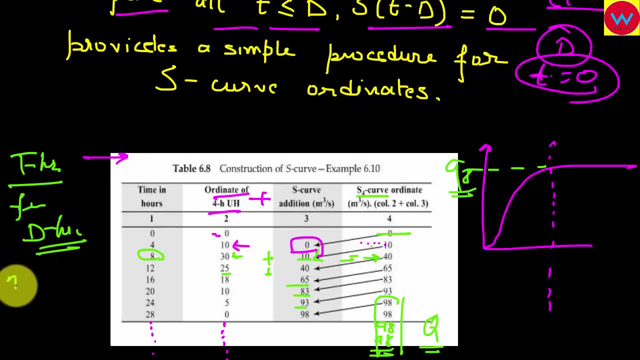 From D our unit hydrograph Earlier. what we have done, We have obtained N times D our unit hydrograph From D our unit hydrograph. That is N. D was multiple of D And here T is not the multiple of D. 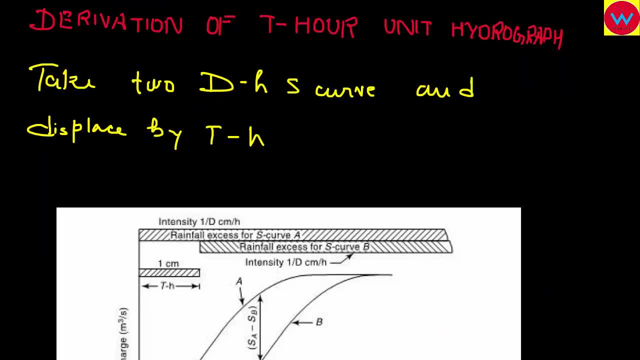 It is the unit hydrograph. In order to Derive T our unit hydrograph From given T our unit hydrograph, We Take two D our S curve And displace it by T ours. So First of all, you calculate. 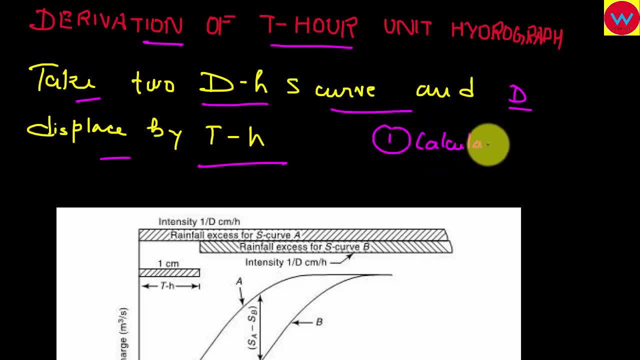 Ordinate of S curve. Calculate S curve For given D our. Then you displace Your S curve By T ours. For example, Let us say This is our 4 hour unit hydrograph Given values, Then we need to calculate S curve for this. 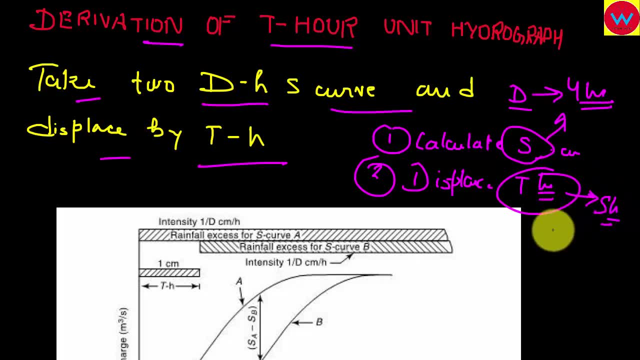 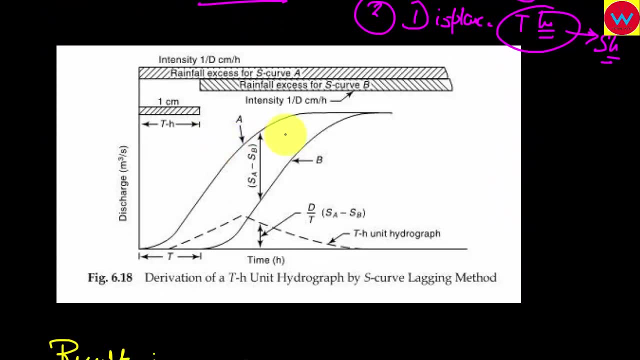 And then we. If you want to calculate 5 hour unit hydrograph, Then we displace these two by 5 hours. Let us see in the graph This: A Is First S curve And We displace it by T, ours. 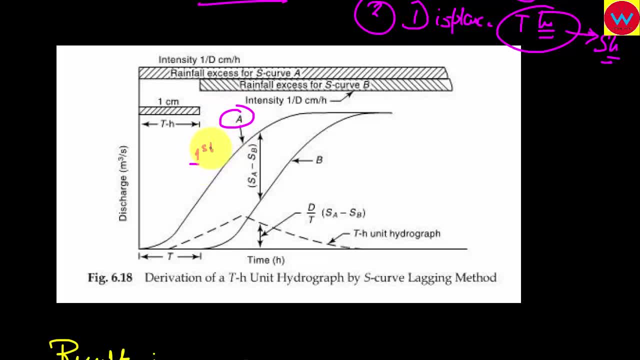 So all the ordinates are displaced. So Here it comes, And here we have second S curve, That is B. Now What we need to do Is To. What we do Is we calculate the difference Of these two? 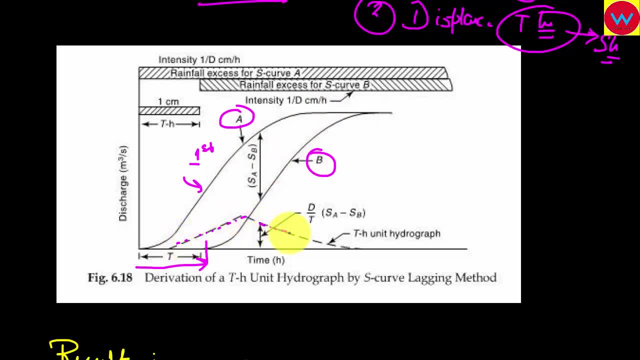 S curve. So this dotted line represents The value of the difference of These two, S A minus S B. But what will happen That? What will happen Is that When we are subtracting B from A, Our rainfall axis- 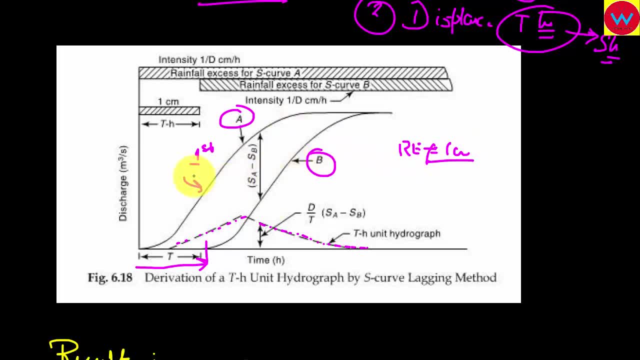 Will be equal to 1 centimeter. So we cannot say that Just by subtracting We will obtain unit hydrograph. What will happen is that We will obtain a DRH Of T hour duration. Where rainfall Where? 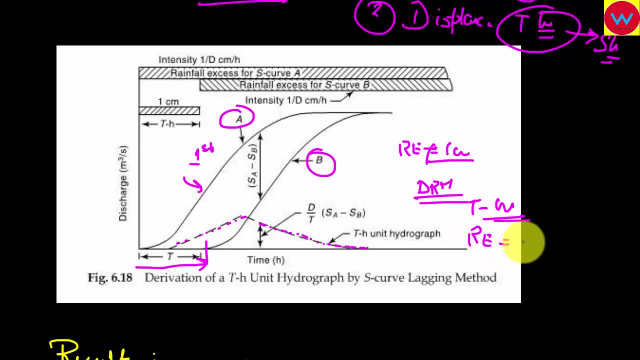 Rainfall axis will be equal to Your Time Into intensity. Intensity is, So Rainfall axis will be equal to T by D centimeter. But we need to calculate. We need to calculate our values For 1 centimeter of axis of rainfall. 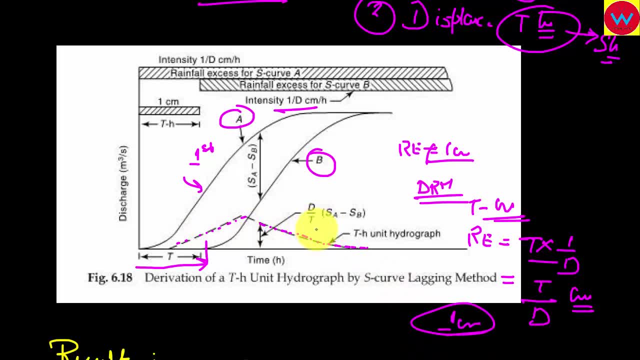 So whatever Ordinance we get, We will divide it by T, by D. So you see here That S A minus S B. You can write it like this: S A minus S B, divided by T, by D. So our 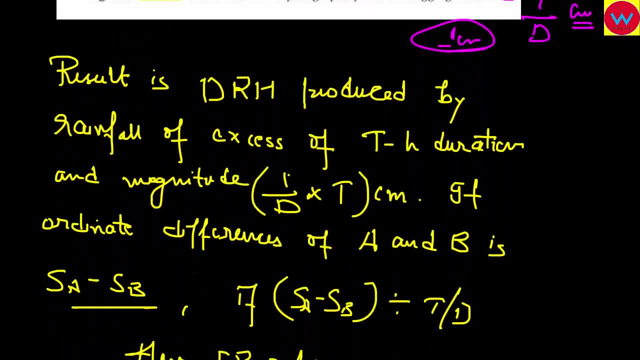 Rainfall axis is this And how we have obtained Is that? Because the result Of subtracting the 2 S curve is DRH. You have to remember this thing. The result is not unit hydrograph, The result is DRH produced by. 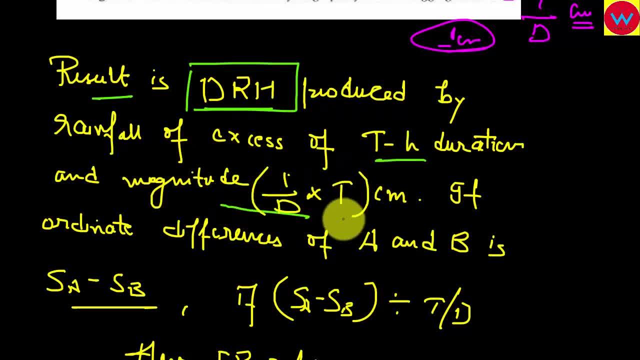 Rainfall axis of T hour duration, Which has a magnitude of 1 by D into T. It is so because T is the duration and 1 by D is the Average intensity. Rainfall axis is 1 by D into T. 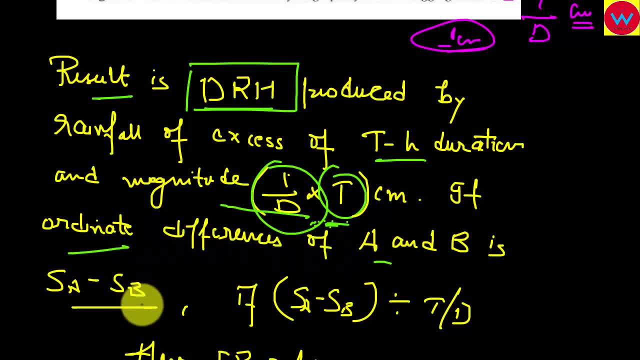 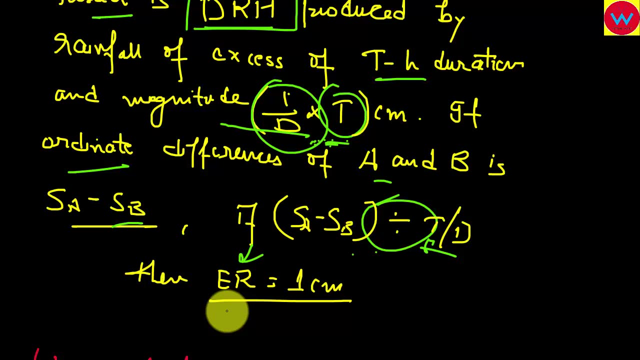 So If the ordinate differences of A and B Is S A minus S B, And if we divide it by T, by D, we get The value of Effective rain. We get value of effective rainfall For 1 centimeter. 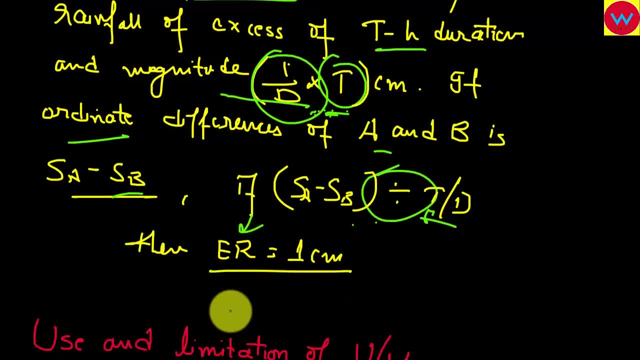 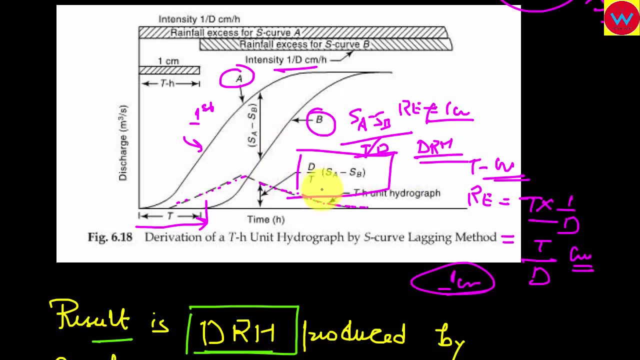 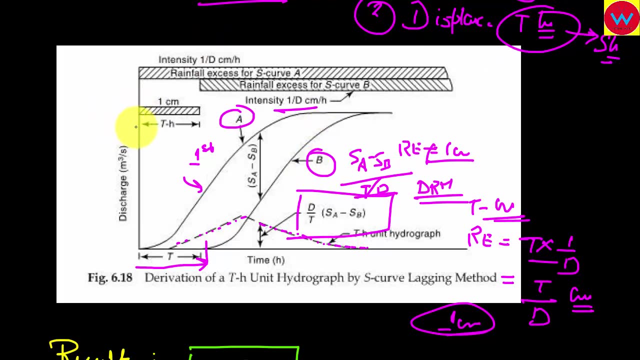 So now we can see that Our, Our graph Represents Rain unit hydrograph. So you have seen How we have calculated T hour unit hydrograph From T hour unit hydrograph. It is quite a complicated process, But you have to remember. 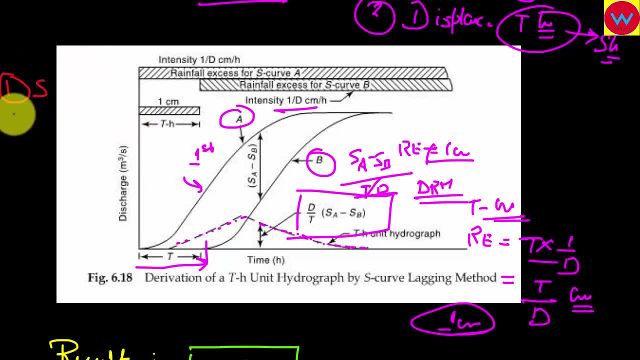 I will once again quickly summarize those steps. First step is that you draw S curve. Second step is that You displace S curve by T hour. And the third step is that You calculate the difference of 2 S curve S A minus S B. 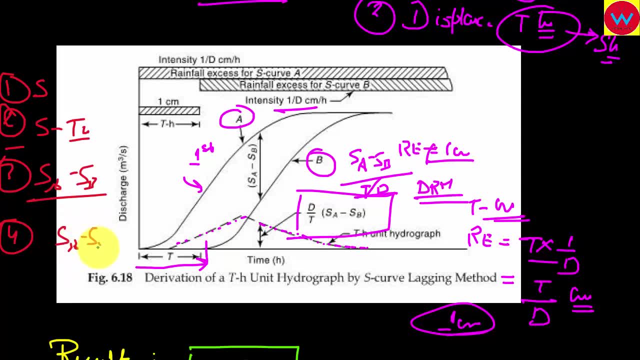 And the fourth step is that Divide the ordinate of S A minus S B By T by D, That is T by D of rainfall axis. So now you will get a graph Which has ordinate of 1 centimeter of rainfall axis. 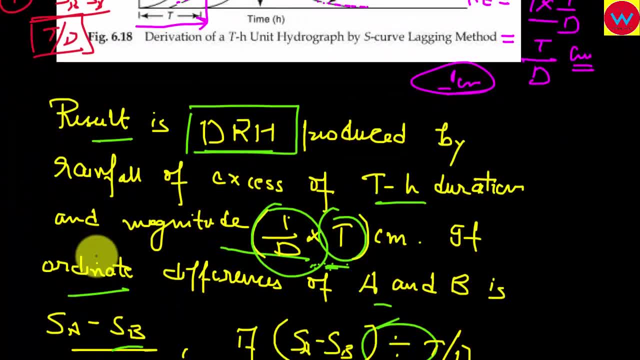 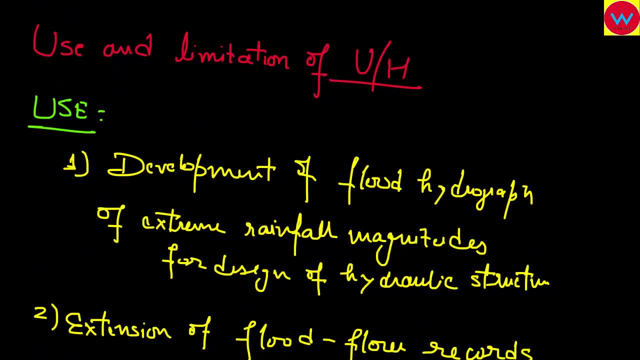 And it will show It will be called as unit hydrograph. Now, what are the uses and limitations Of unit hydrograph? We will look at it very quickly. Our first use is that We can use it for the development Of flood hydrograph. 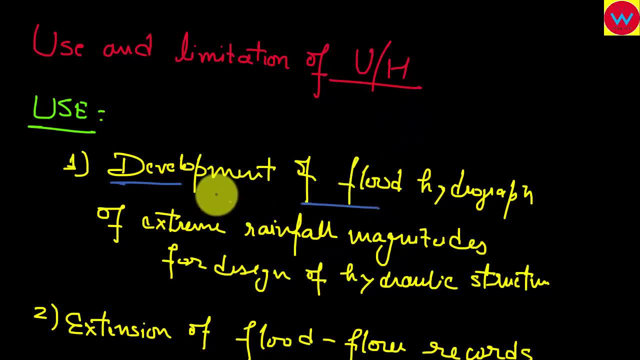 If we do not know How the catchment is going to behave For the given rainfall axis, We will use unit hydrograph method. Basically, We are interested in Knowing the extreme rainfall magnitudes For the design of hydraulic structure, That is we are interested in. 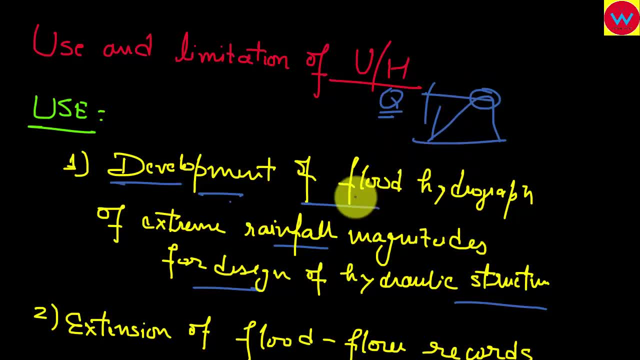 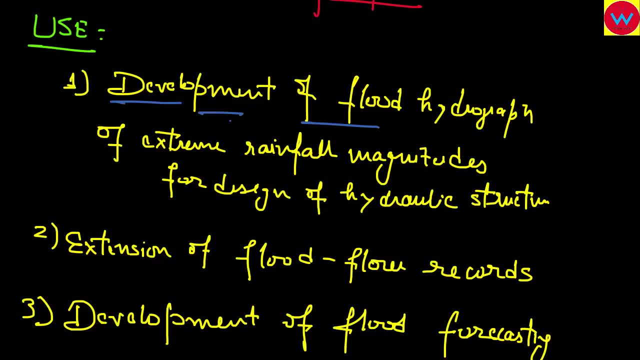 Knowing the value of this peak, That is, how much maximum Q value will be there For rainfall extreme, So we can use it in this. This hydrograph can also be used For Flood flow records, that is, If we do not know. 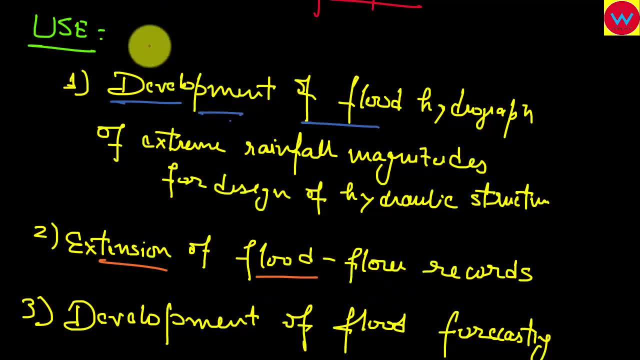 The record values of some flood. Then we can use The ordinate obtained from the Hydrograph to Interpolate or to extend Our record. And third advantage is That we can develop The forecasting method of flood, That is. 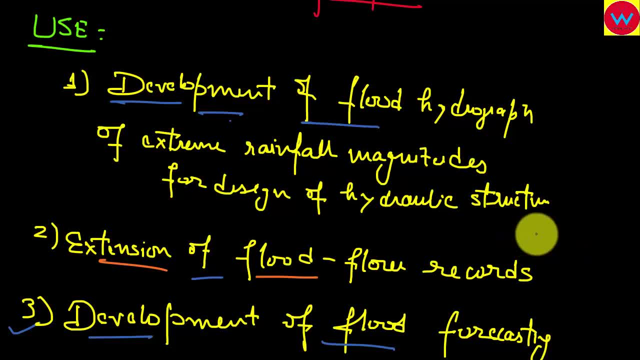 If a particular amount of Rainfall axis is likely to be there, Will there be a flood or not For a given characteristic, Given catchment area? It is. if the, This value of Hydrograph is like this, This shape of hydrograph, then 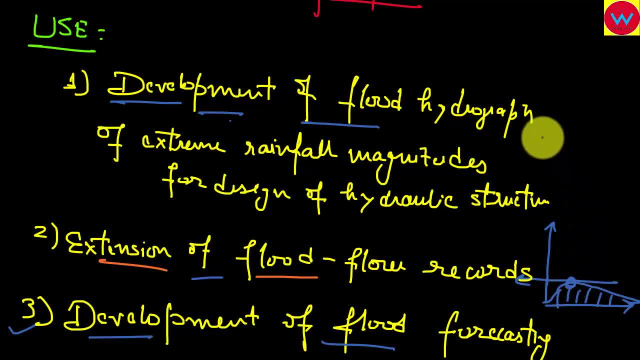 We know that we do not have a high peak Value of discharge here. But suppose the our Graph of hydrograph Is like this? then we know that We know it in advance That our maximum peak Is likely to be this much value. 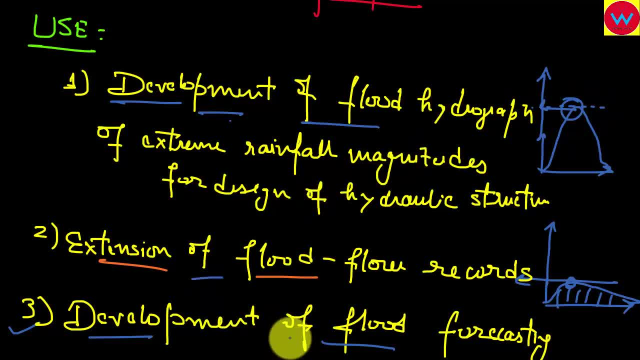 And it may be unsafe For our Hydraulic structures. or We can forecast flood On the basis of discharge values And how the water Is likely to recede, based on the Study of recession limb of hydrograph. So there are. 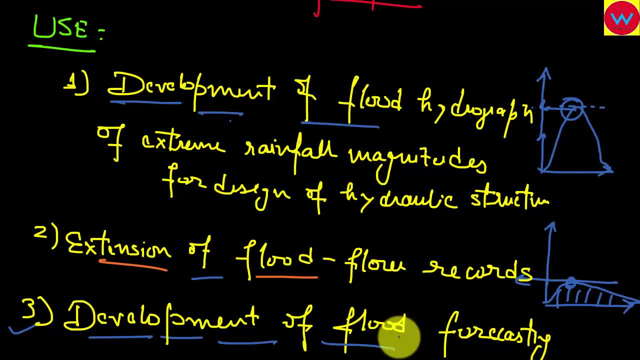 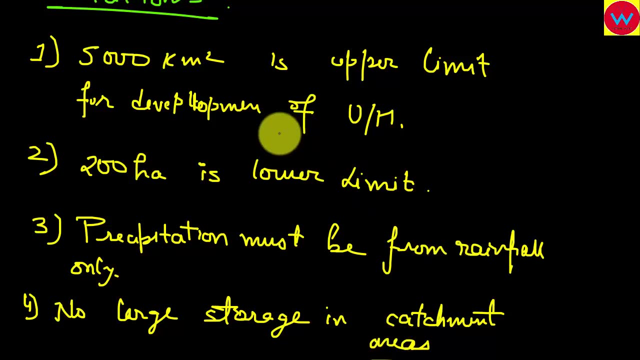 Lot of things we can do With the help of hydrograph, But these three are main Use, which we have looked at shortly. You can study it in detail. Now let us Look at limitation of Hydrograph. So the first thing is that 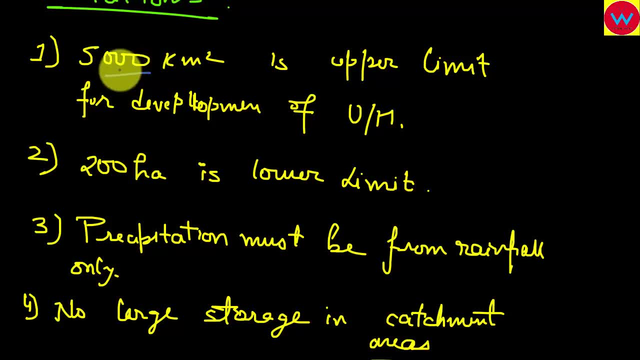 You know that Our assumption states that We know that 5,000 km2. Is upper limit for development of hydrograph. That is, we cannot Make hydrograph Hydrograph from 10,000 km2 of area. 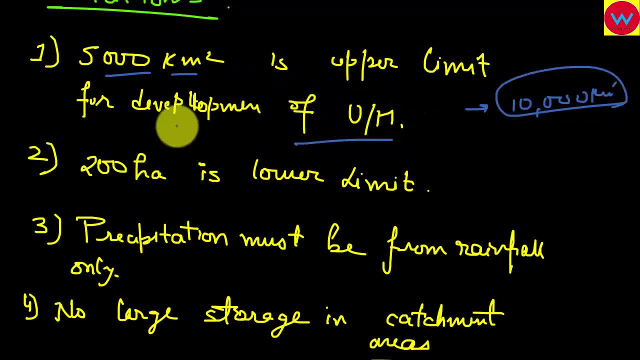 Because that will not be a valid one. Assumption: 200 hectare Is our lower limit. We have to be. We have to choose Area or catchment from These two Limits only. Third Limitation is that precipitation must be. 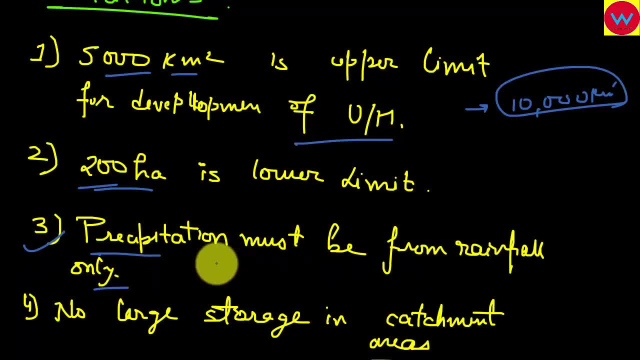 From rainfall only. That is, we cannot assume, We cannot obtain the values for Ice fall, Snowfall or other Forms of precipitation. We have for Assume for all practical purposes That precipitation is from rainfall only, And We have to also look at